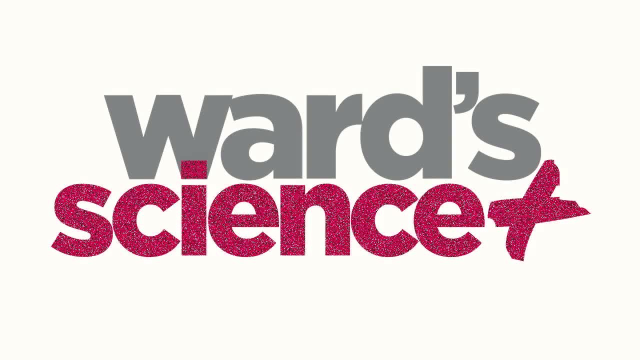 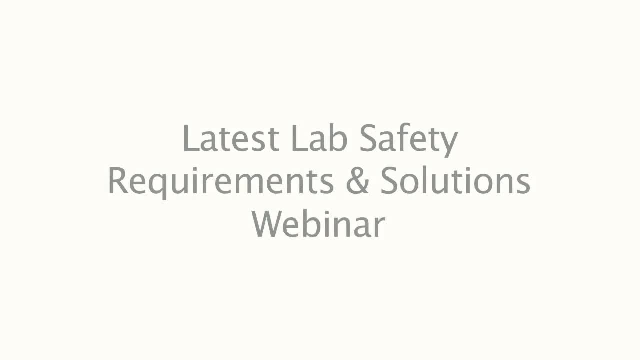 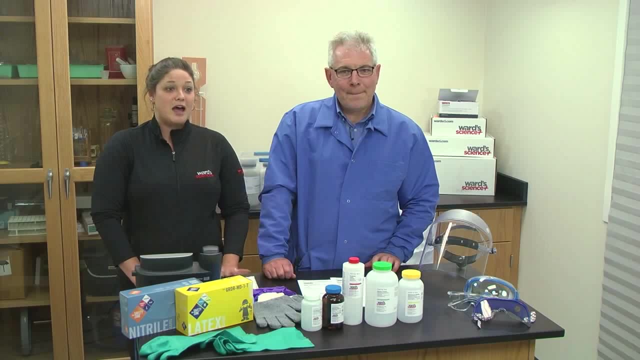 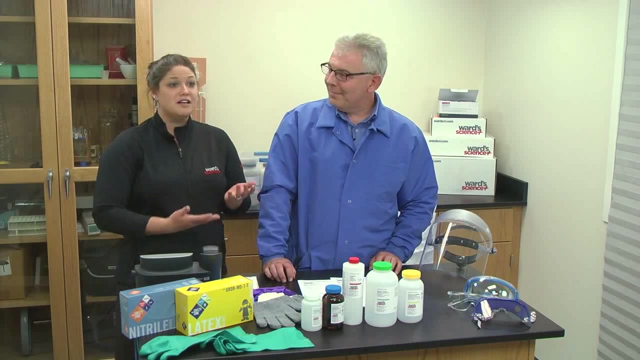 My name is Dr Liz Hoffman. I'm one of the scientists here at Ward Science and today I'm happy to introduce Alex Milenich, who has over 25 years of chemical and biological safety training and expertise. He's been manufacturing and selling chemicals and working with chemicals pretty much his whole life, so we're very happy to have him here. 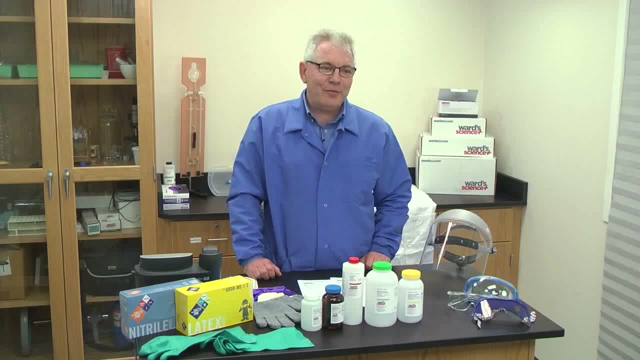 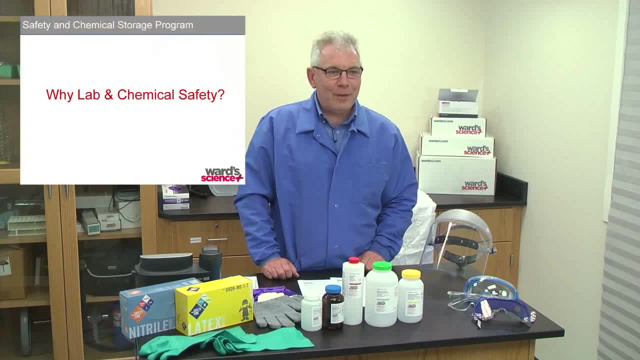 Again. my name is Alex Milenich and this is actually my first webinar. Most of the time I'm doing presentations in person. I can look out and see, you know, 90 people in a classroom. This is a little different for me, so it's kind of cool as we can go worldwide. 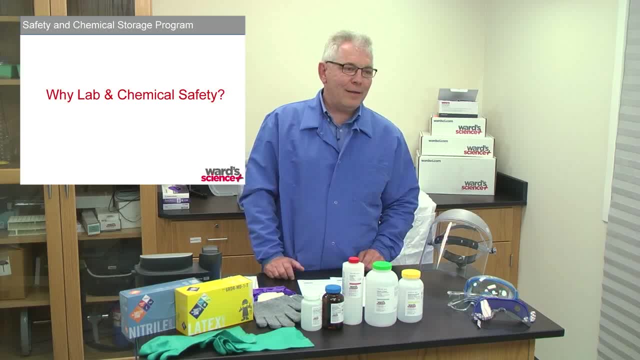 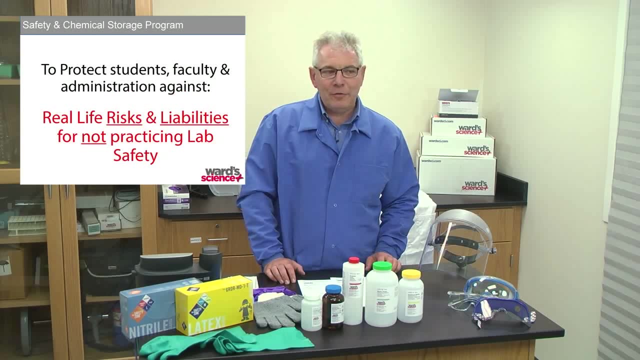 So we want to talk about safety and chemical storage. You know why lab and chemical safety? Well, it is also important one. we want to protect our students, Our faculty, our administration against real-life risks and liabilities for not practicing lab safety. 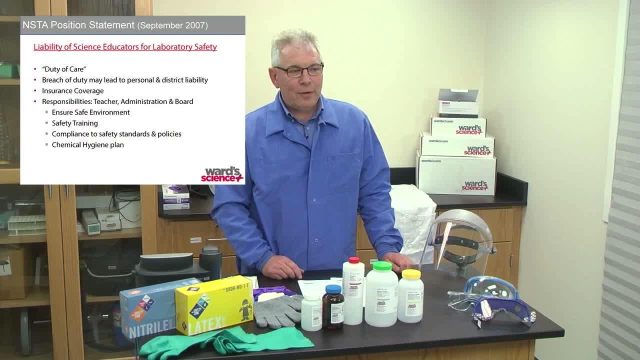 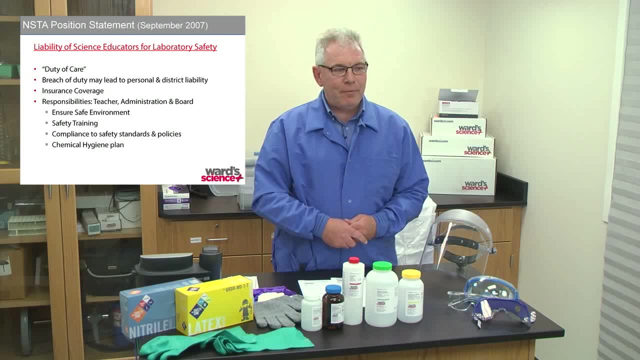 Next, please. So there is actually. we have to worry about a little bit of duty, We have to worry about a duty of care. So in that classroom setting- and I'll give you an example of a local school district here in the Rochester area- 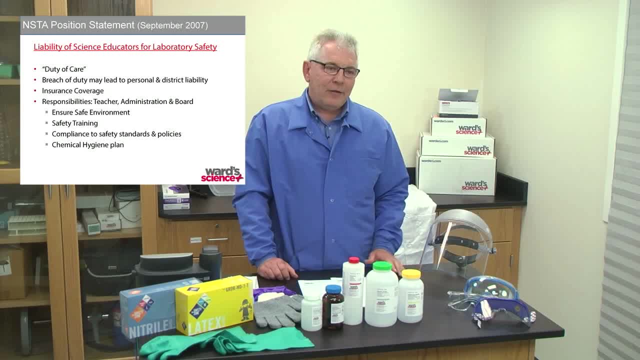 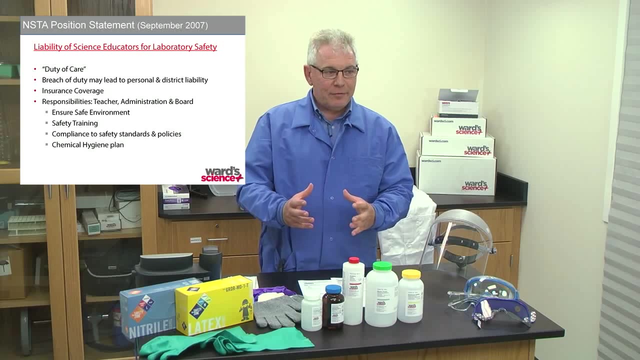 So there was an issue where they didn't actually test any of their IWA stations, And so they. So the teacher decided that they were going to use open BATS of methanol, And so we were going to have those, you know 8 inch wide things of methanol. 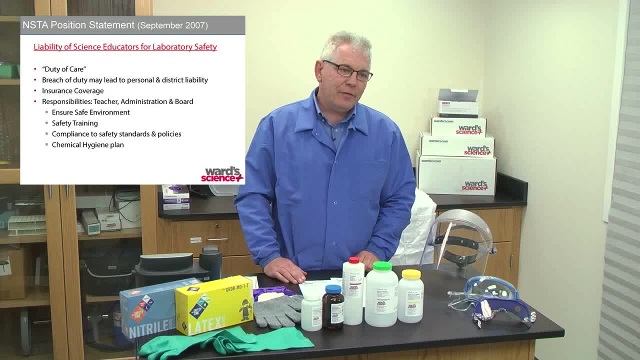 We lit them. We lit them And the students are actually going to then take a chemical. We're going to look at how they are burning. Unfortunately, one of the students actually caught on fire, So they didn't actually have. they didn't test any of the IWA and or showers in their classrooms. 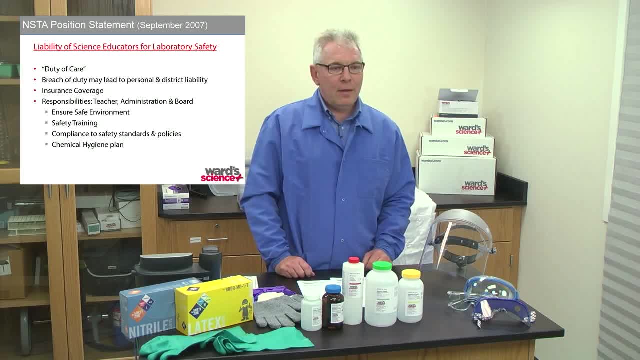 So when they went to pull the shower to actually help out the fire, they're off. So there is a duty of care around that, in the sense that general laboratory safety has to be undertaken in the classroom. We have to actually worry about that breach of duty and how it is, how that impacts you as a 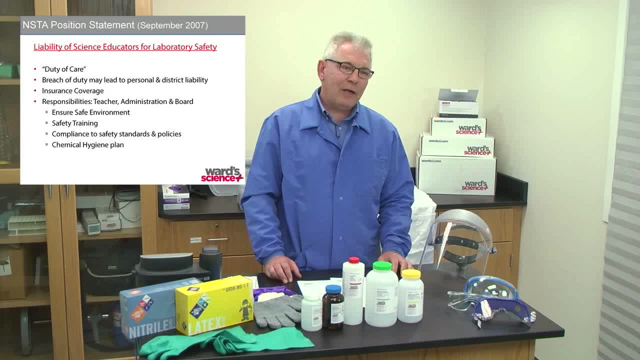 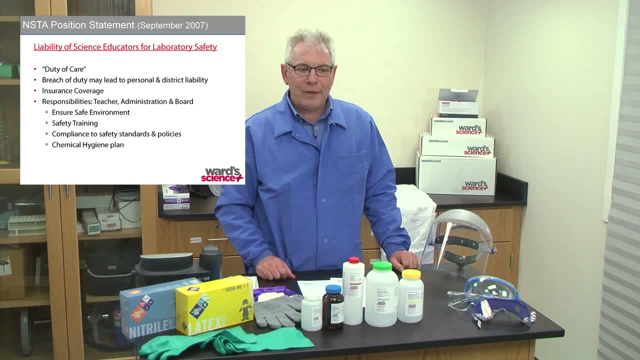 teacher or the district liability around that. We want to make sure that we actually have a safe environment around us, we actually have safety training, we have compliance to those safety standards and policies and a chemical hygiene plan put in place. You, as a teacher, have to go through training in. 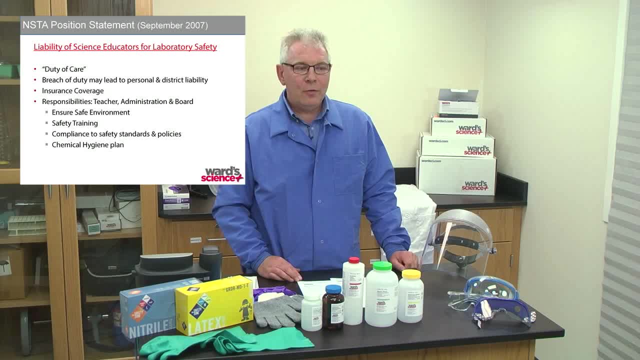 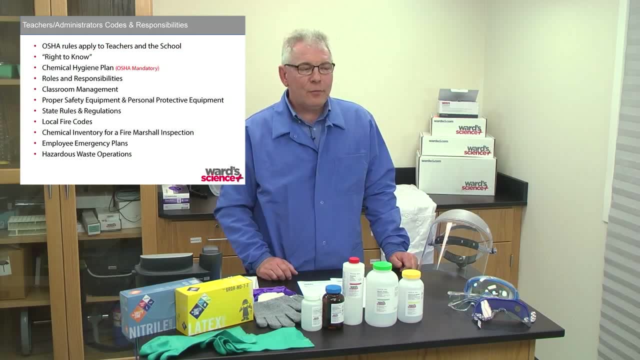 the sense that you have an employee-employer relationship with your school. Next, So some of the things that we need to worry about. So we have to worry about OSHA rules and how it affects teachers in the school. You have a right to know in your classroom, or actually as an employee of a school, what 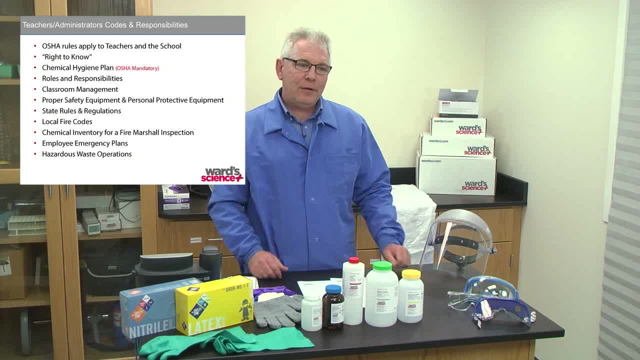 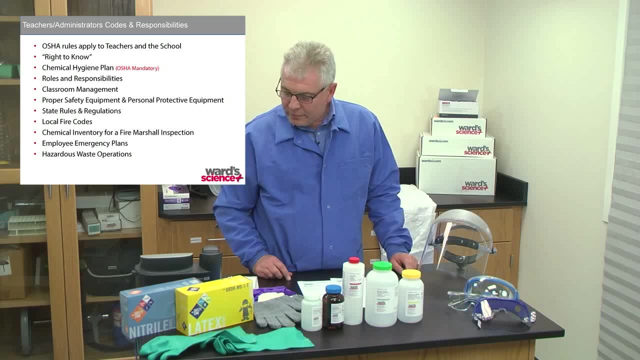 are the chemicals that you're exposed to. Here again, every company. here again this is. we're talking about OSHA, so it's a US rule. Same thing happens in Canada under WMIS, and there are other countries that have the same thing. Let me just stop. There is some feedback going. 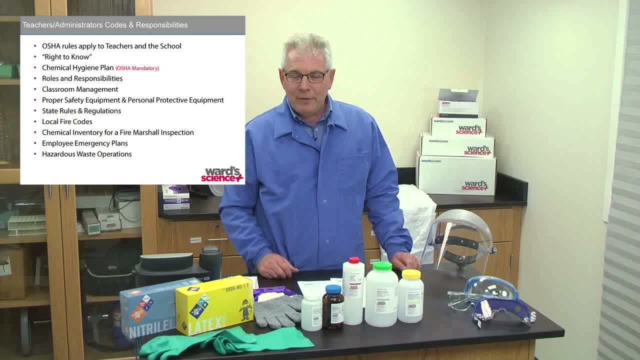 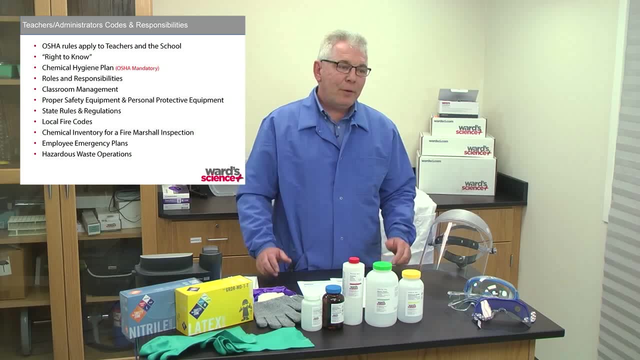 on. so, if you can, everybody press star six, make sure we're muted. There's some feedback coming back, so make sure that it's you're not talking. Thanks, appreciate that. We want to make sure that in that classroom management role that we 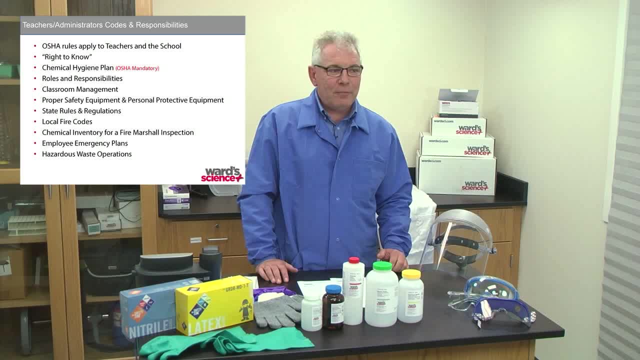 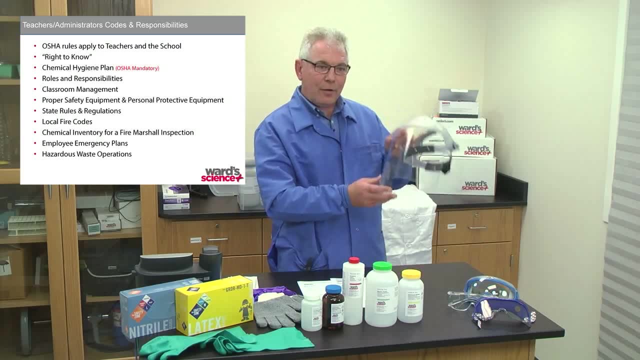 are managing that classroom and sometimes that's a little difficult sometimes, but we want to have that. make sure that happens. Proper safety equipment. So here again are you know? are we, do we have the right equipment in the classroom, Whether it's goggles, face shields and the personal protective? 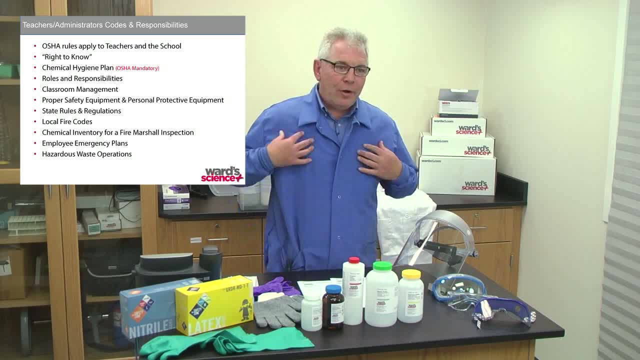 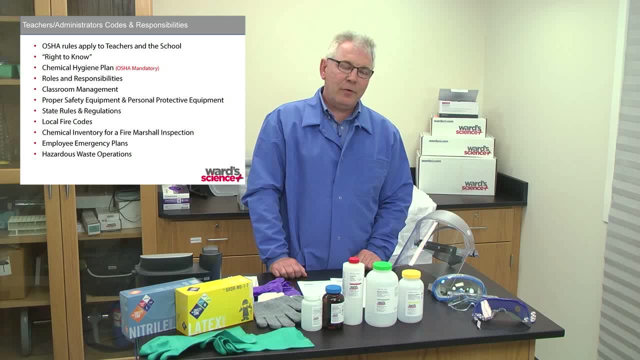 equipment, whether it's gloves or an apron- Here again, I'm just wearing a lab coat. There are state rules and regulations- that we'll talk about a little bit- and, of course, local fire codes. So your local fire codes, fire. 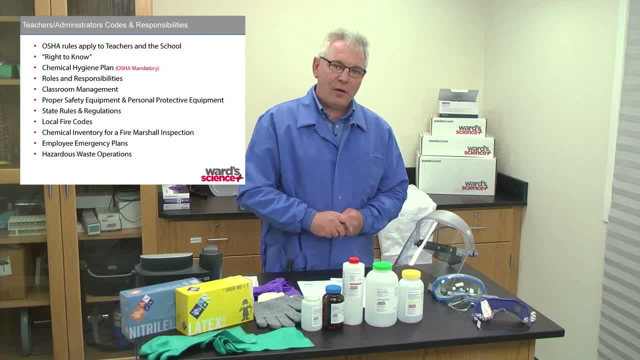 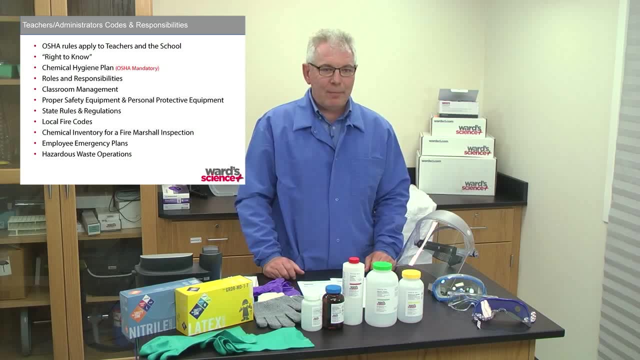 you know they are a good example. they can trump whatever state law you have. So if a local fire marshal came in and said: you know, I really only want to have, you know, X amount of flammables, even though state law might have a different ruling. 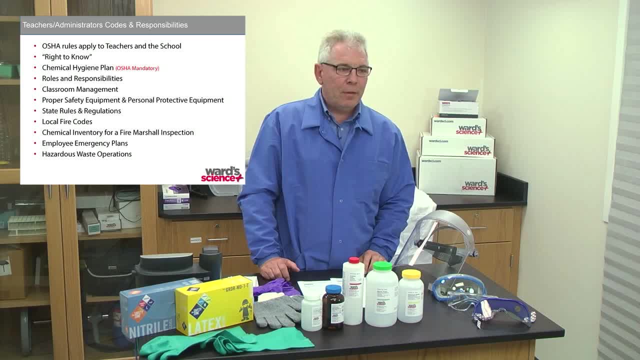 That's fine, because you kind of have to follow that local rule. We'll make sure that we have a chemical inventory system for and or even if it's on an excel spreadsheet or the back of an envelope. We have to have something that keeps track of the chemicals that you have in your system. 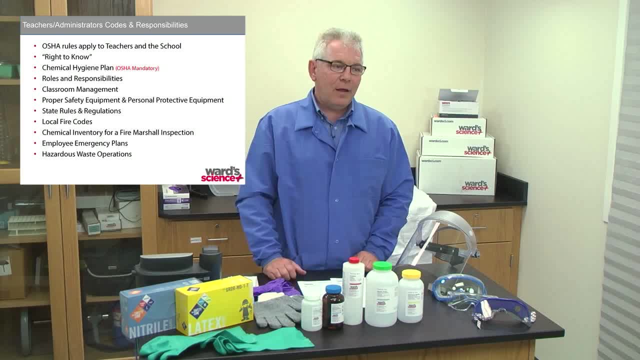 operation and or classroom. here again, that's something that you need to have. there are a lot of really cool things that Ward sells, so they have a chemical inventory management system that's online so you can access it on the internet. everything resides on the cloud today. you have to make sure that we have 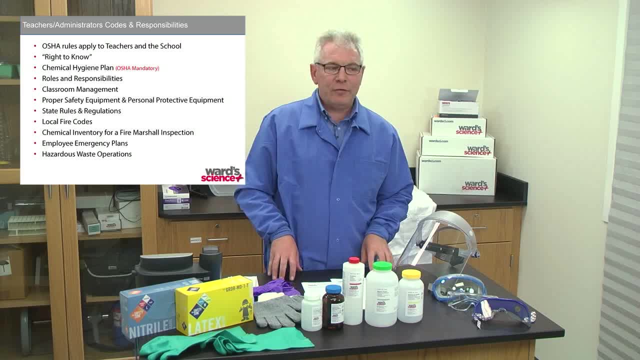 some kind of an emergency employee plan and we have to understand hazardous waste operations. so we want to make sure that in even with hazardous waste, that we're not taking hazardous waste and just throwing it down the drain. we want to make sure that we're getting rid of it in the right way. so if you've ever 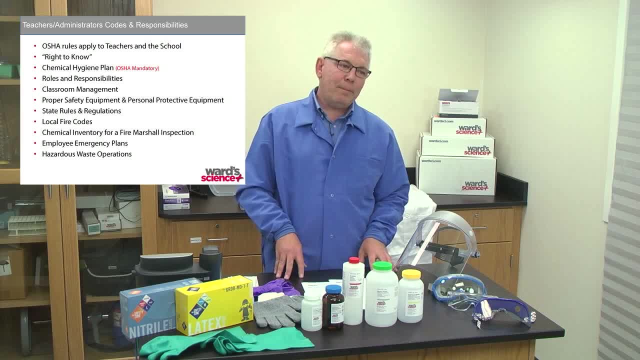 heard cradle to grave. so basically a cradle to grave operation is whatever chemical that is. until it's it's owned by the school district, that gets rid of it forever. so four thousand years from now, if it came out of the ground, the school district still owns it. a lot of reputable companies today we'll actually 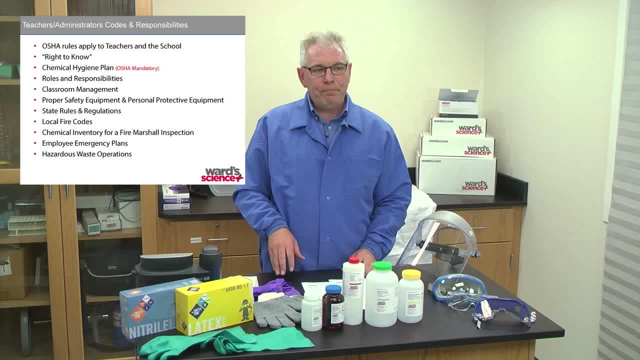 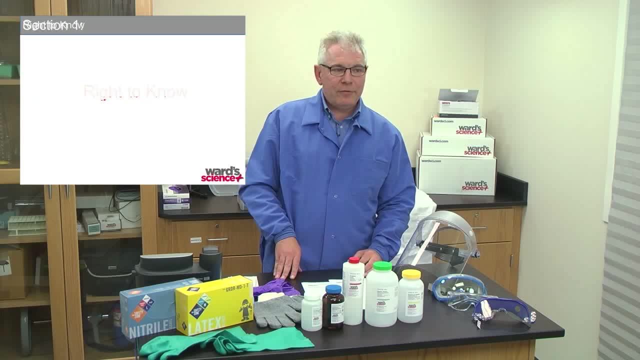 you use incineration, if it can be, versus landfill, So it's actually incinerated. So under section one we have a right to know, So OSHA has a right to know. hazardous communication plan. That standard actually changed a little bit this year. 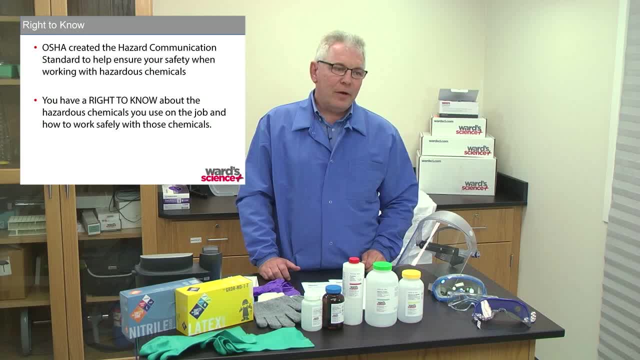 and we're gonna go into some detail around that Has Com started right around the late 70s, early 90s, So, I'm sorry, 80s. So you have a right to know about all the hazardous chemicals that you use in a job and how do you work with them safely. 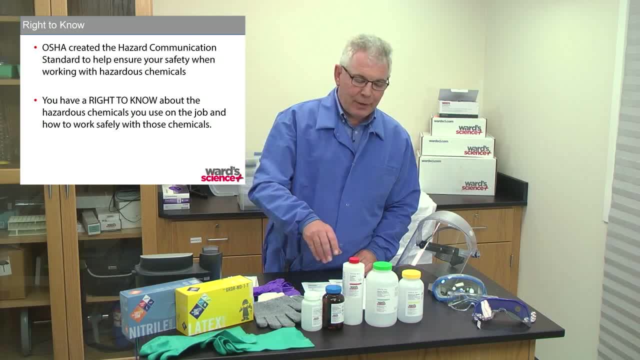 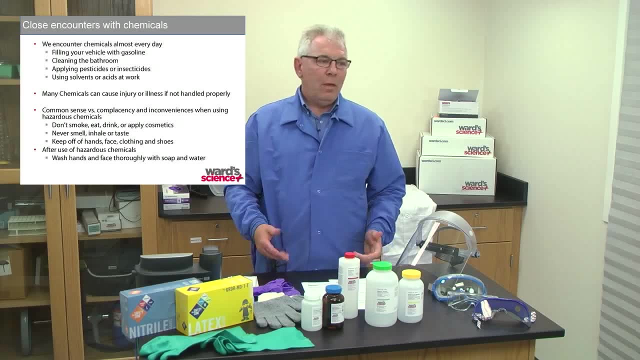 In a laboratory. So the first perspective around that, of course, is always gonna be the label that you have on the chemical You can go next. please, Before I get into actually laboratory, I wanna talk about some close encounters that you might have with chemicals every day. 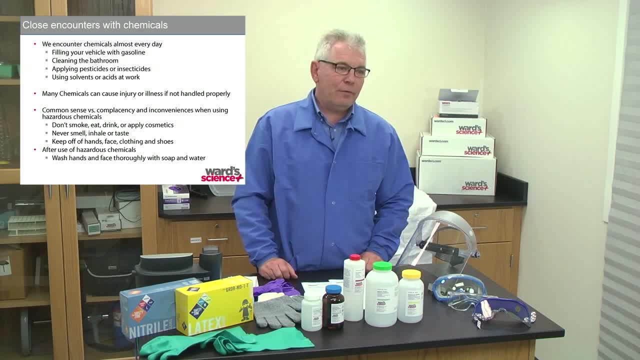 So every day people say: oh, I don't use chemicals. But if you're cleaning the bathroom, you might be filling your car with gasoline. You might be applying pesticides or insecticides on your lawns using solvents or acids. 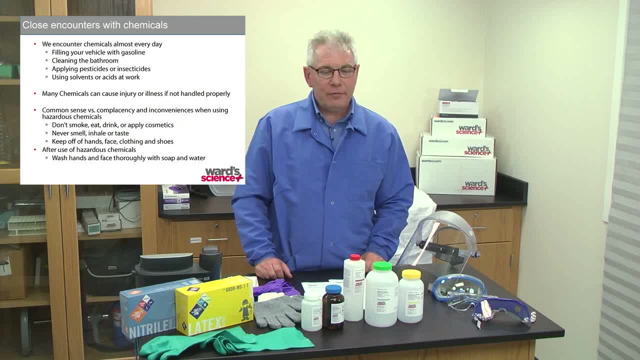 drain cleaners and so on. So there's chemicals can cause injury or illness if they're not handled properly, But at the same time, if handled properly, they can be very, very safe. So we wanna make sure that we have common sense. 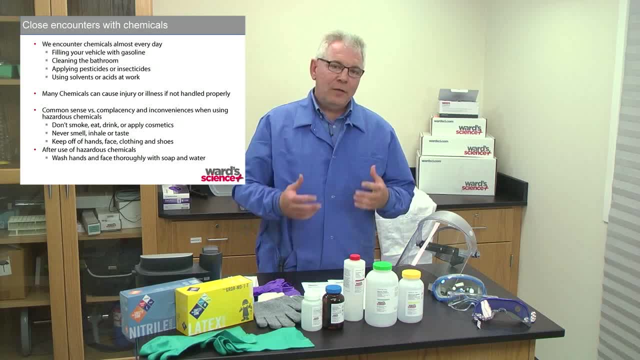 versus complacency or inconveniences. You know, sometimes when you're at home you can actually run a lab and run a classroom, but yet at home you might. ah, why should I bother to wear safety wear, I might have a little workshop in my basement. 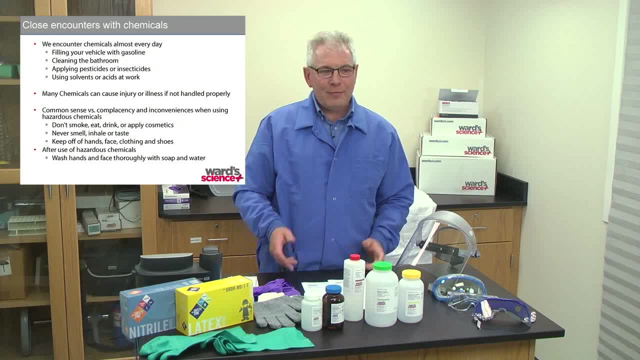 I might have a grinder wheel, You know, should I put a pair of safety glasses on? Well, it's just something insimplistic, You know, and that can be the time when you get injured, So you have to think about it. 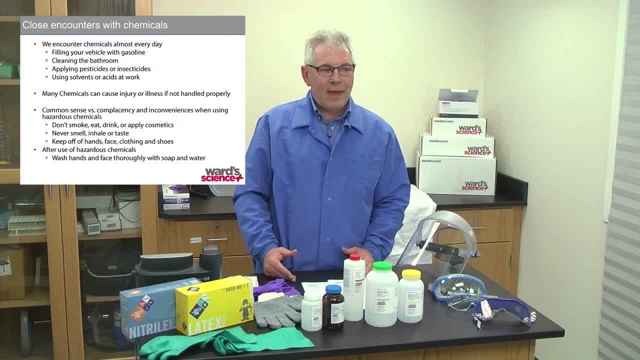 when you're trying to manage a classroom, that you wanna actually make sure that you are following those common sense rules. that we're wearing safety glasses, maybe a face shield when we're using acids. We wanna make sure that you know it's common sense. 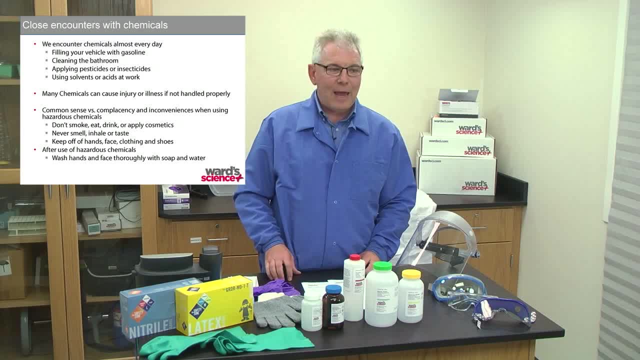 but yeah, don't smoke, eat, drink or apply cosmetics, you know, in the lab. Here again, we wanna make sure when you're managing that classroom, kids aren't pulling things out and sneaking gum or eating in the lab. 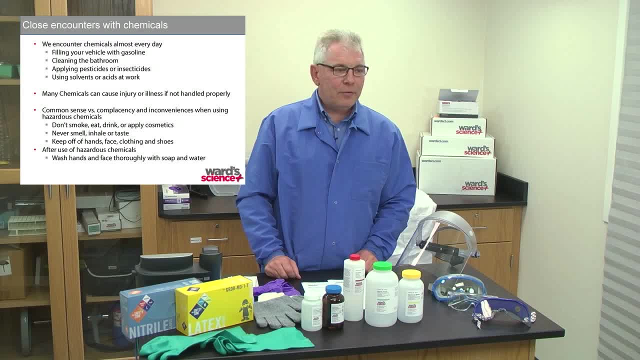 We wanna make sure that we're never smelling, inhaling or tasting chemicals And we wanna make sure we keep things off hands, face, clothing and shoes. And, of course, after using any hazardous chemicals, we wanna make sure that we wash our hands. 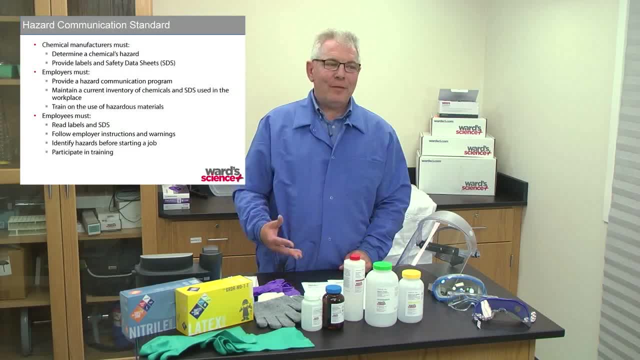 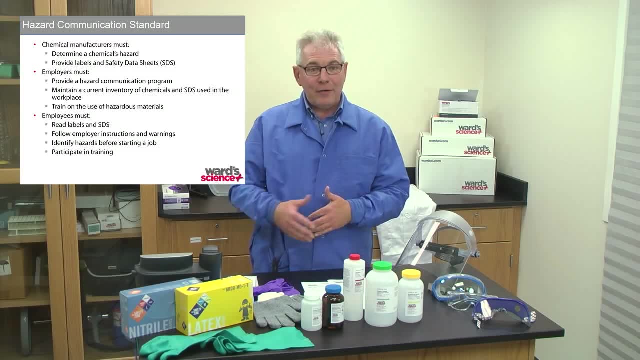 and face thoroughly with soap and water. Okay, so let's talk about hazardous communication standards. So, within that standard, we wanna make sure that the chemical manufacturers. so if you're manufacturing chemicals, it's a little harder than just distributing. So if you're manufacturing 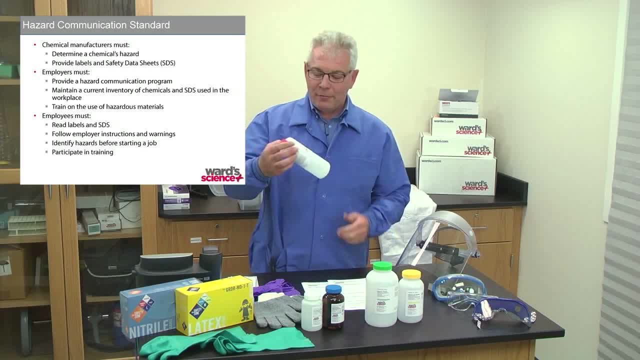 we have to make sure what those hazards are. So today we have a bottle from Wards. Those hazards are gonna occur or they're gonna be on the label. We wanna make sure that we're getting a safety data sheet, So what's called. 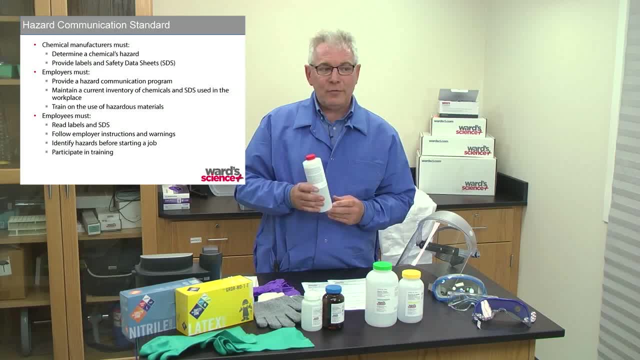 what used to be a material safety data sheet is now an SDS or safety data sheet. That change took place June 1st 2015.. A lot of the Wards chemicals had safety data sheets as of 2013 or 2014,. 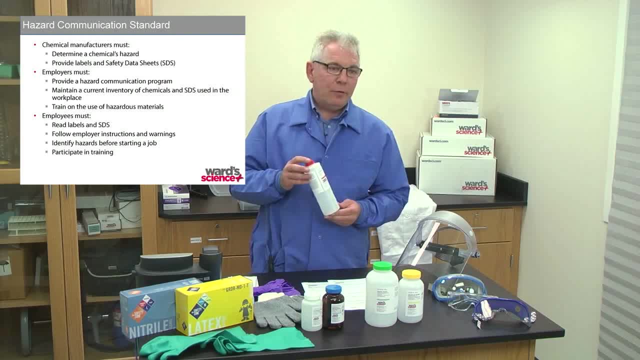 so way ahead of the change that occurred with those in June 1st, but as an employer. so the employer meeting a school district, if you're a teacher, has to have a hazardous communication program and maintain a current inventory. or chemicals and SDS is in the workplace. 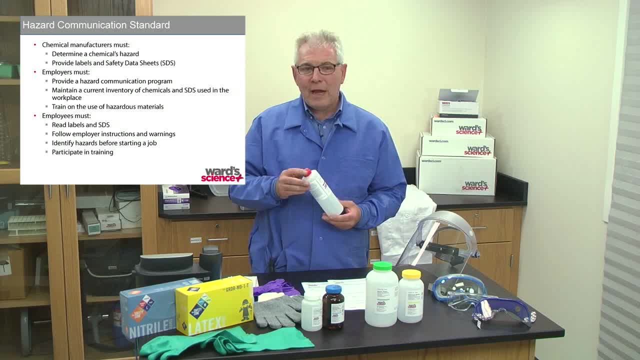 And then you have to go through some kind of a training, which is usually through a hazardous communication training and how to read a safety data sheet and how to read a label. Employees go back. So, employees, we actually have to go through, you know. 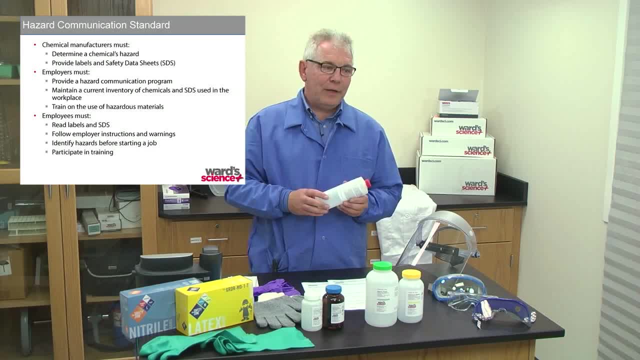 We actually have to make sure we have a responsibility too. So, you know, if we're in a lab setting or school, we have to make sure that, yeah, you know what We're really reading the label of the SDS. 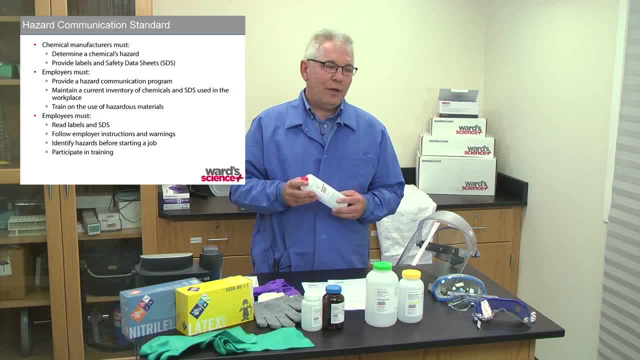 We have to follow instructions and warnings. We have to make sure that we identify those hazards, of course, before starting a job or a lab. So if we're going to start the lab, we want to make sure that we're reading the safety data sheet ahead of time. 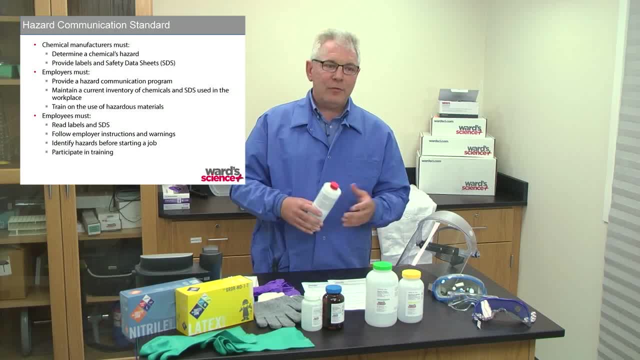 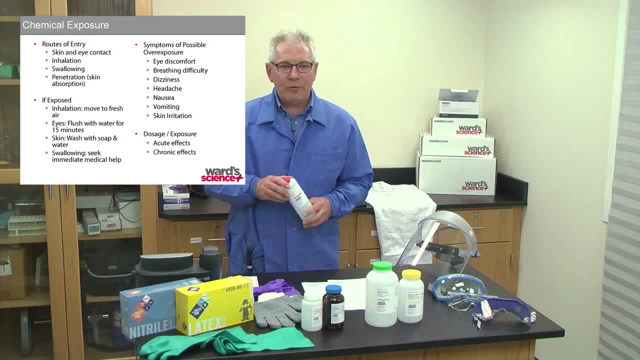 or the label that we don't spill something and then go back and try to figure out later. And we want to make sure that we're participating in training. Next, Let's talk a little bit about chemical exposure Here again. so what are the routes of entry? 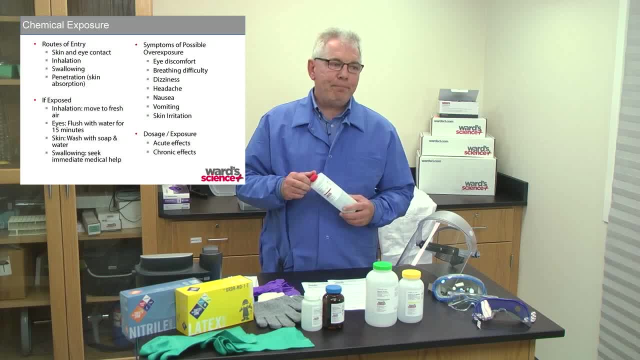 So the things we have to worry about in that classroom setting or a lab, you know, skin eye contact, inhalation, swallowing or penetration, Penetration doesn't really occur that much in a lab setting versus an industrial where something is penetrating the skin. 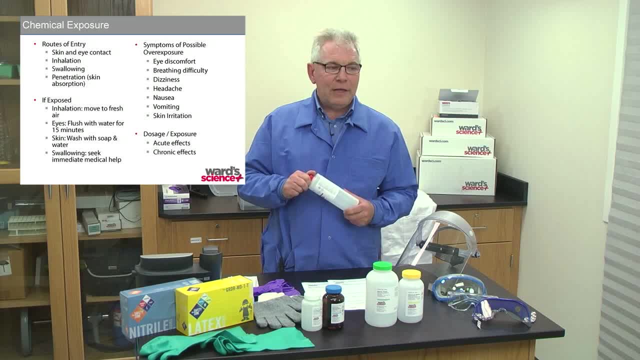 We want to talk a little bit about, you know, if exposed. So you know inhalation, if you're going to move that person to fresh air. Here again, if something, if you're inhaling Eyes, you know we want to make sure that we're. if something gets in your eyes, you're flushing those eyes for 15 minutes. 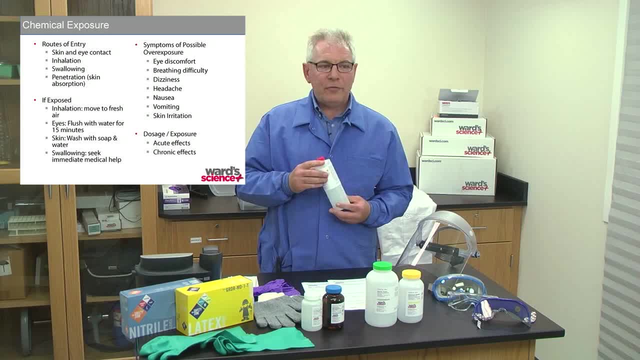 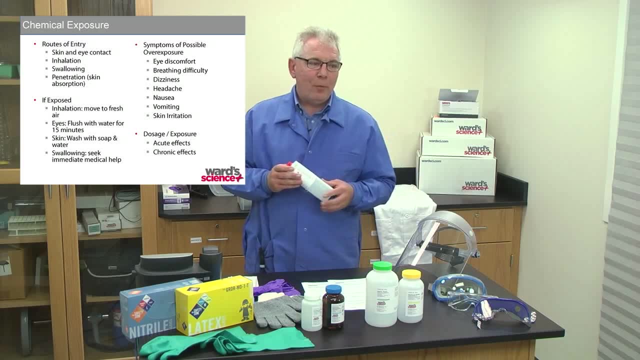 That is an OSHA standard, So we have to have those eyewash stations available so that we can actually go for 15 minutes. I always use the example of my wife. So she was a teacher, also worked in a lab. She actually got picric acid and in her eyes and one of her friends basically took her head and put it into an eyewash and capped it there. 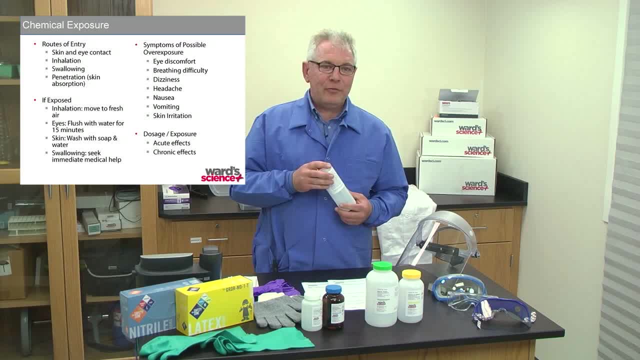 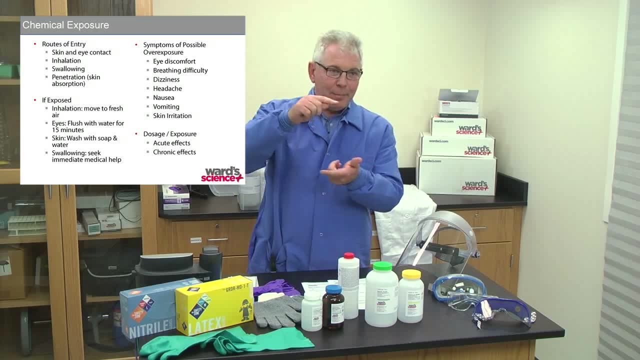 So it helped save her life, It helped save her eyesight. but here again you have to make sure that that that eyewash stations available, those little bottles that you might see, um, that are about this big, um, that is not enough water to actually have 15 minutes of of of washing. 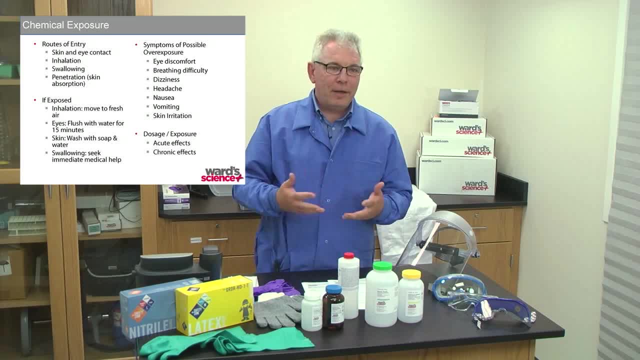 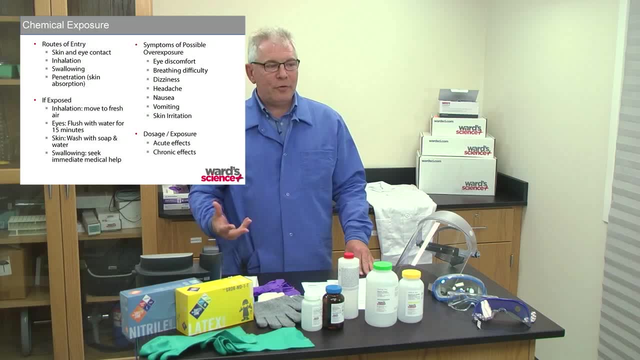 It's not the most comfortable thing, um to stick your head into water, but it it's, it's, you have to do it. Scan If you get your. so, if you get chemicals on your skin, we want to make sure that we're washing with soap and water. 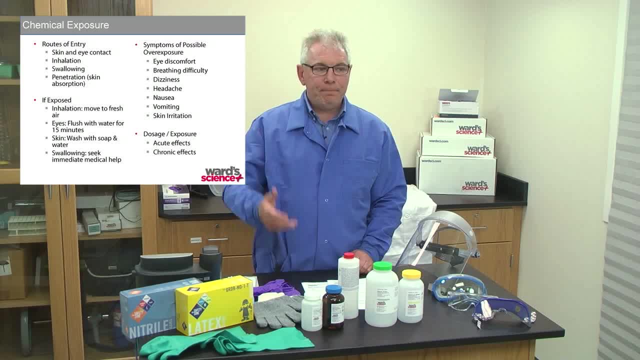 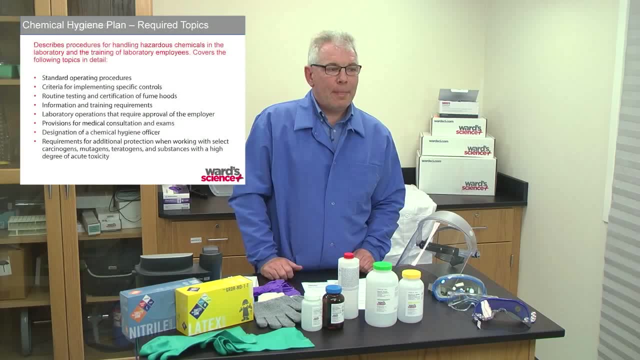 And, of course, swallowing. we're going to seek immediately- Uh, immediate- medical condition. on the right hand side, you're looking at the different symptoms of possible overexposure next. So, chemical hygiene plan. So the thing with the chemical hygiene plan: we want to make sure that we have one for every school. 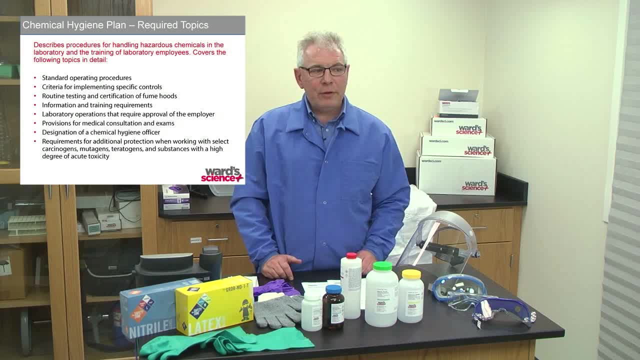 So here again, this is a notion of standard that we have. We want to make sure we're describing procedures and handling a chemical- hazardous chemicals- So we want to make sure that we have that chemical Hi Gene plan. So we have a standard operating procedure how we're going to work in that classroom. 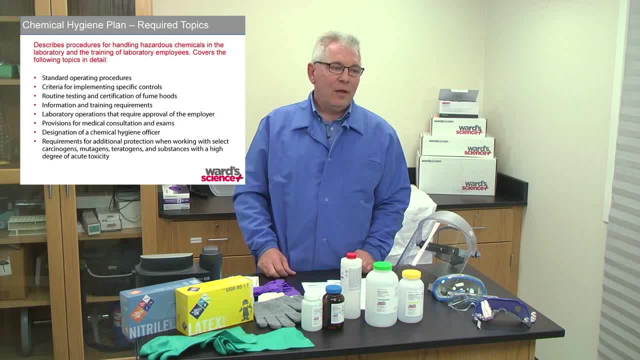 So we don't have criteria for implementing those controls and routine testing of those fume hood. So we want to make sure that you know, here again, with a few input, you know we come in in the fall and we start. we want to make sure that the fume hood is actually working and we want to make sure it's certified. 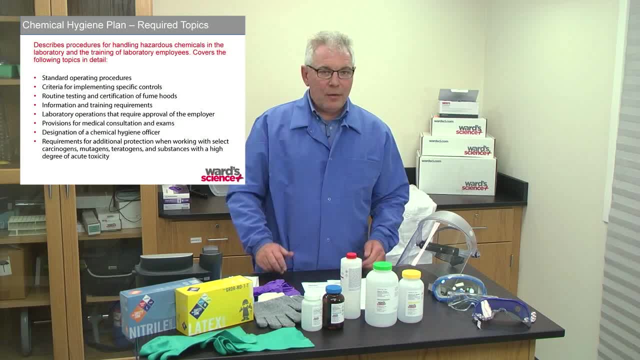 You know what is that? um, exposure, um for the fume hood, so that you know, over the summer a bird didn't actually end up in the event. Um, so we want to have, We want to have that certified at least once a year. make sure it's it's working. 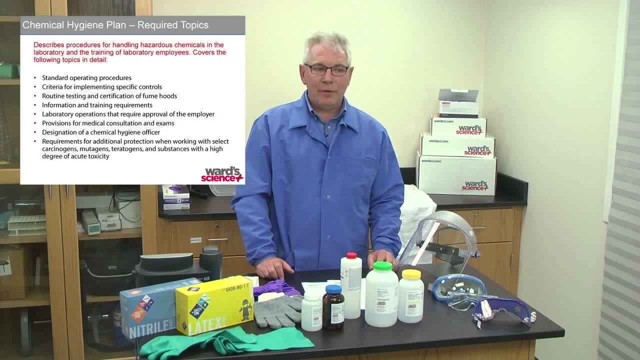 Um, we want to make sure that any kind of laboratory operation we're doing require the approval of your employer. So if you just try a rogue lab, you know we want to make sure that it's um, it's safe. Um, we also want to have a chemical hygiene officer in every school or lab. 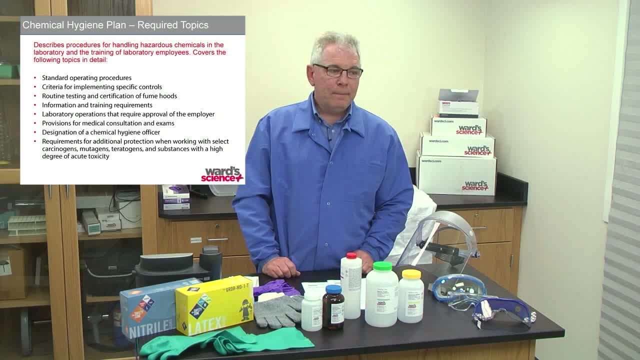 So we want to make sure somebody's responsible for safety for others And, of course, we want to make sure there's any additional protection when working with carcinogens, mutagens, terror. Here again, those aren't usually used in schools but we want to make sure, if that is happening more at a college level, that there is some additional requirements around those. 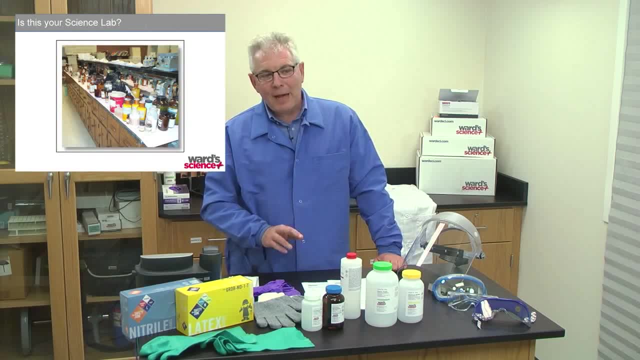 Is this your storage system? So if you want to look, there is um if you want to go back. so this is. these are actual pictures that were taken off the internet. I've been using these for a couple of years. 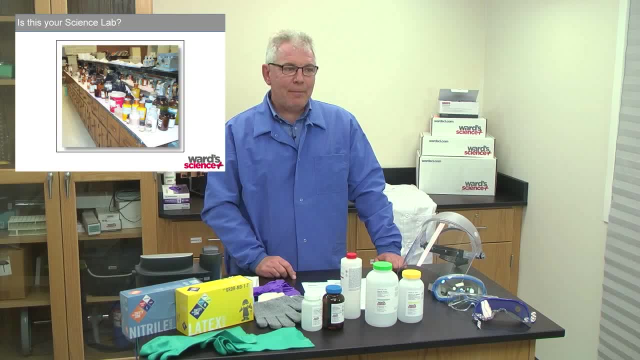 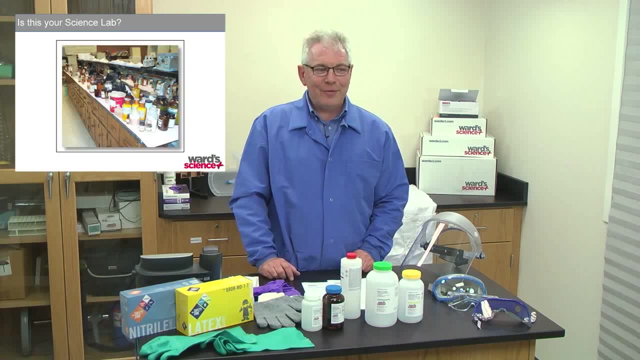 So my safety training these are: this is an actual um lab, um in a school. So this is kind of how they store their chemicals. It's not the greatest way to do that. There is no segregation Here again. I want to talk about a little bit about segregation. 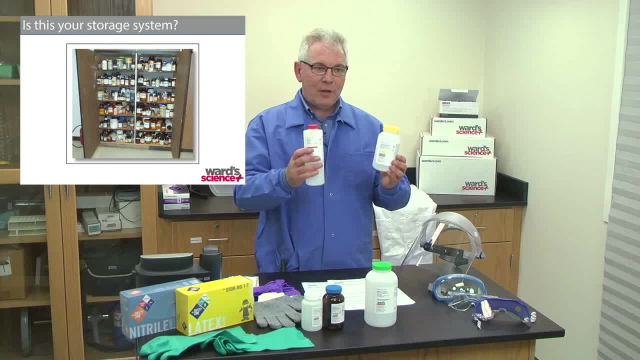 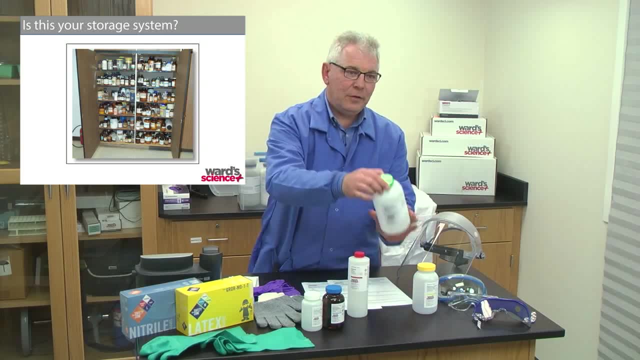 We're going to get into details. So when you buy a chemical boards we have color coded systems. So you know red is flammable, yellow is an oxidizer and there's a little cap here That's yellow. So you can see. green is our general storage, blues are the poisons. 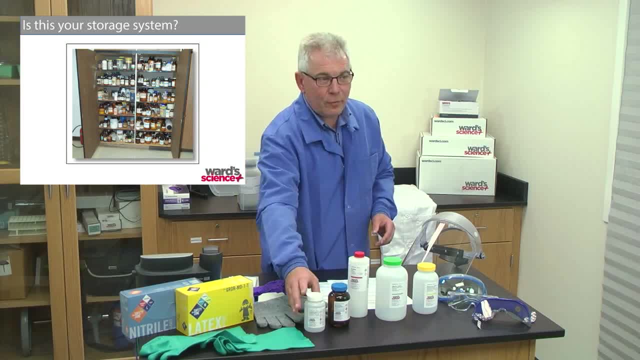 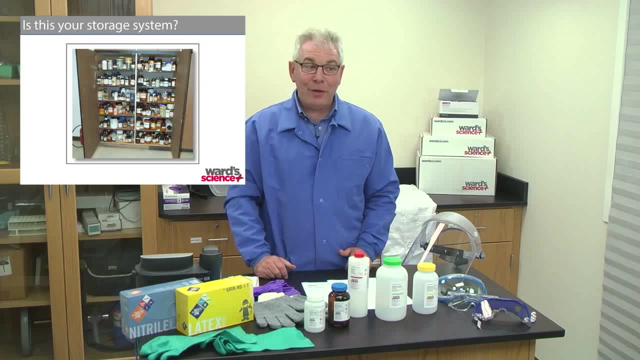 You want to make sure they're on the lock and key and white is corrosive. You can see the one in your uh on the PowerPoint is just a random mix of A to Z, not any. it's not a great storage system. 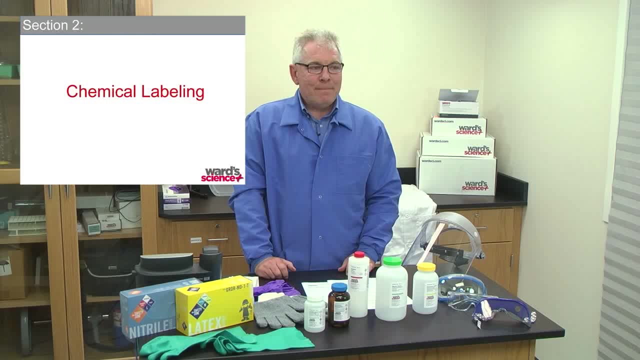 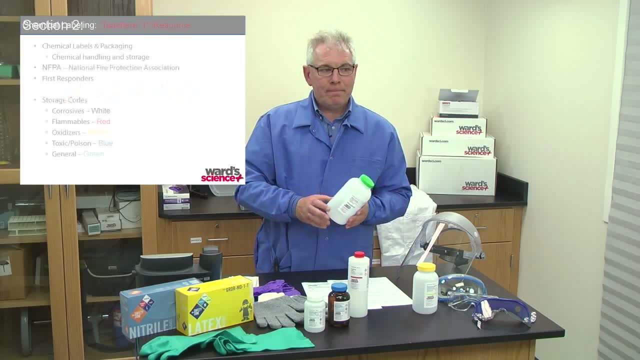 Next. So we're going to go over chemical labeling. So that's our first line of defense in our chemical labeling next, So when we get in here again, we're living in an SDS world today, So we want to make sure, and I talked a little bit about our storage codes. 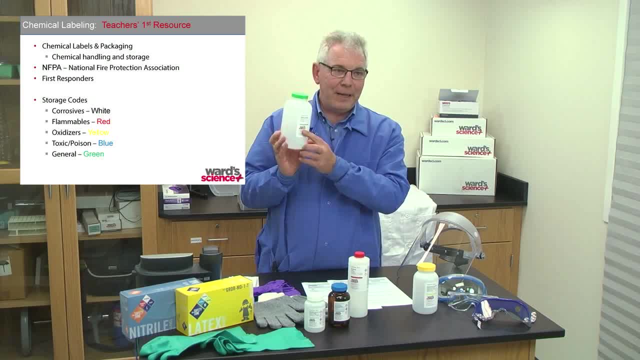 Those are actually on the top, So it's not like does it say storage code green in a band, but we have a color cap now, today, today. So this is a storage code green or a low hazard um counter chemicals, sometimes referred to as general storage. 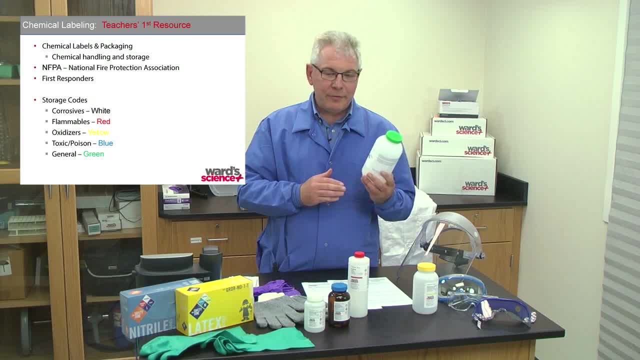 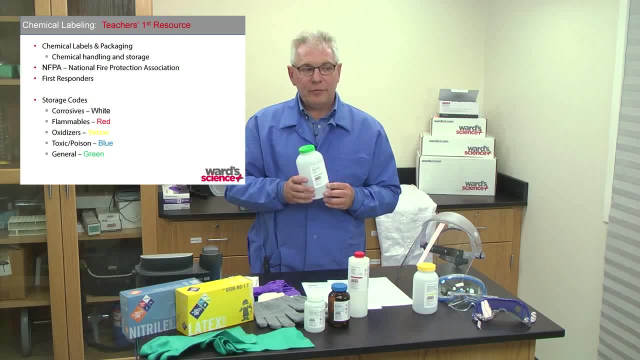 Um, we want to make sure that people understand our storage system. um, by using the storage system, there's five different ways to store it, So we are corrosive, flammables, oxidizers, toxics or poison, and general storage. 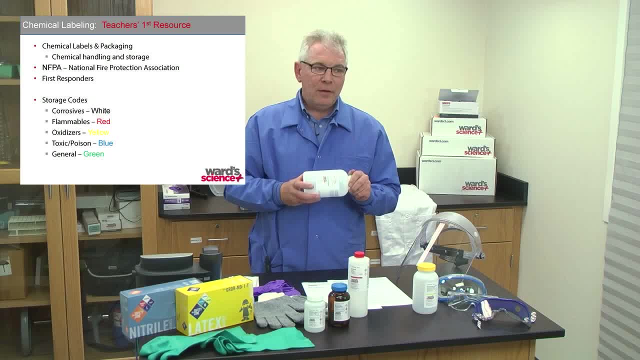 Very simple. It's going to um eliminate any kind of uh worry in that classroom setting as you segregate it by color code. There are others that um storage systems that are on the market today. Some of them are very confusing. 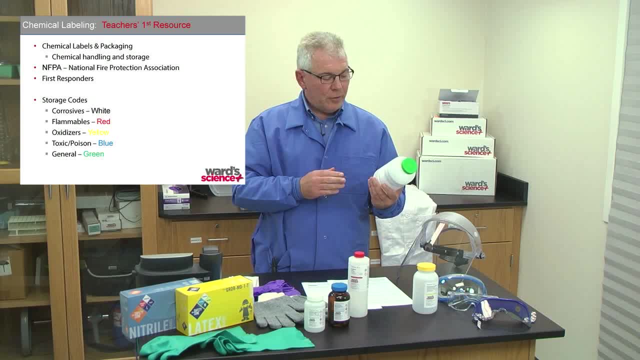 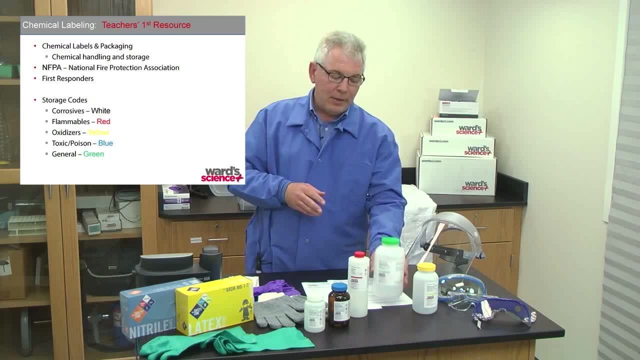 They can go up to 18 different ways to store your chemicals. Some of those Um. this is a very simple uh way and a lot of industrial um companies use this, especially in academia and uh college and beyond. 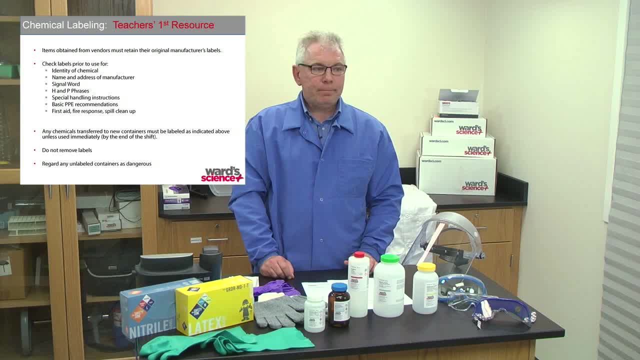 Next please. So chemical labeling. So what do we have to worry about? And that's changed a lot since June 1st. So we have a very robust label today and for our boards- chemicals, but today it actually has to have an identity of that chemical. 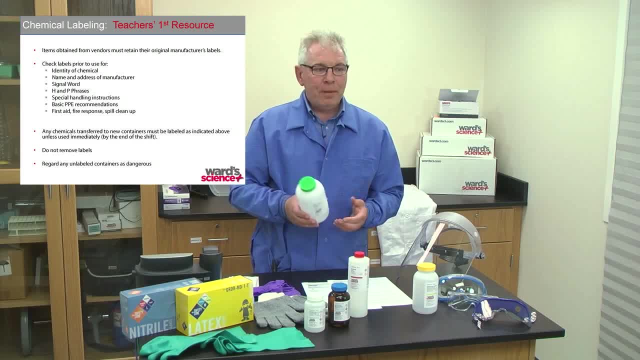 We have to have A name and address of a manufacturer who made the chemical Um. there has to be a signal word. So those signal words might be warning or danger. There are hazardous or H and P phrases. There's special handling instructions. 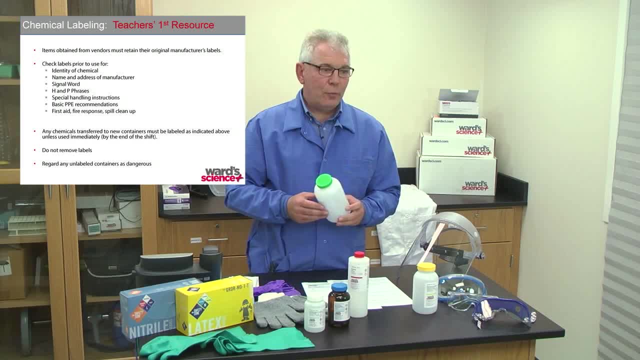 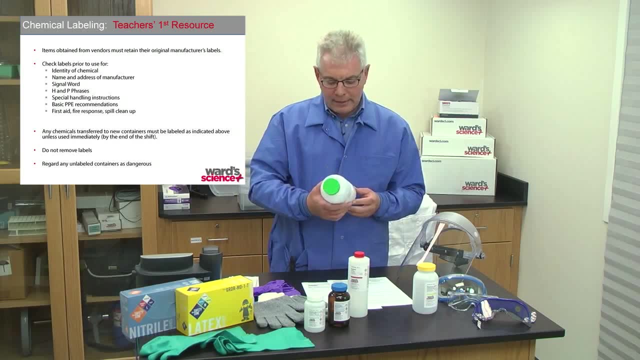 There's some basic PPE which are um: what do you need to do to um sort of personal protective equipment? It's a first aid, response and cleanup. So today you can buy a chemical in a concentrate format and if you're making those, 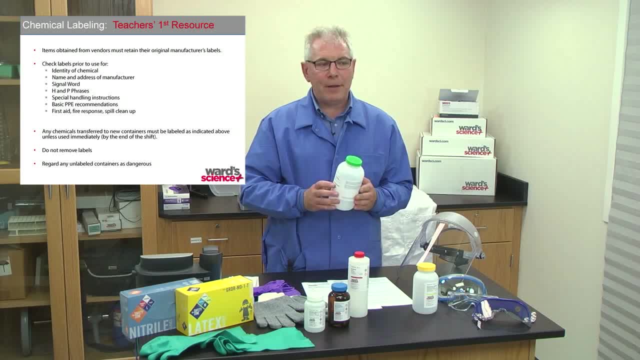 Chemicals for your classroom, we want to make sure that they're labeled property properly. So if you're using them within that class day, that eight hour period, and not storing them overnight, it's a little different than if you're making bulk and storing them overnight. 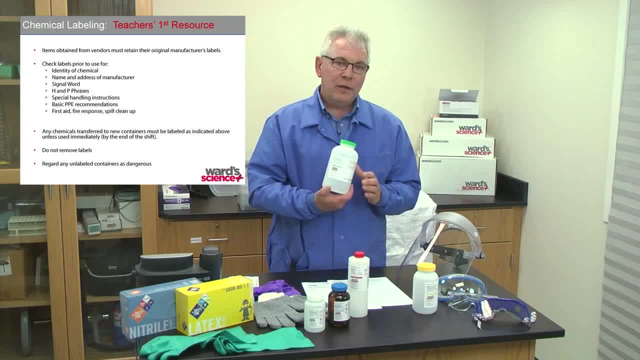 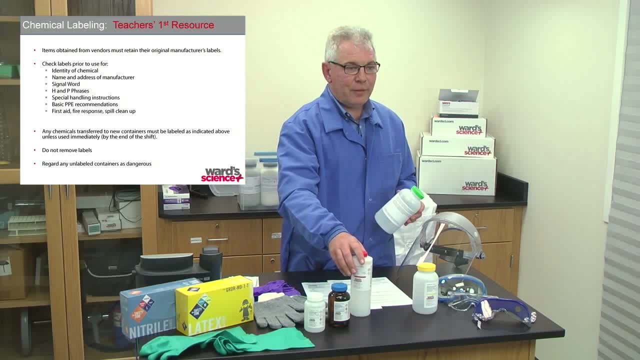 So once they're stored overnight, we have to follow GHS rules and you're going to have- we'd have- to create your own labels. If you buy a chemical from wards and it's already pre-mixed, you can just put that back up on the shelf. 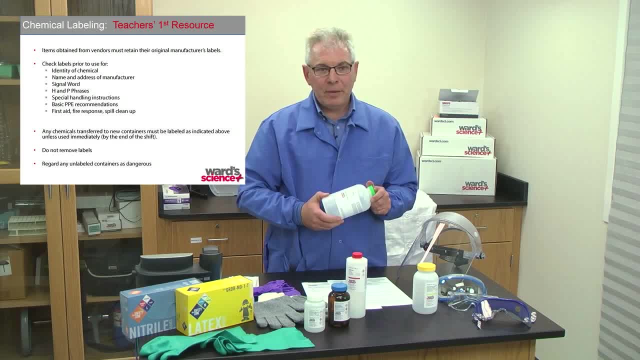 So we also have to worry about unlabeled containers. So anything that you see is unlabeled, So you find it in the back of a classroom. We really want to consider that dangerous. We don't know what's in there until we can figure out what it is. 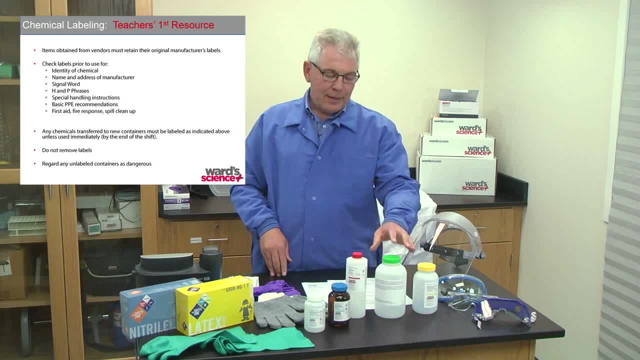 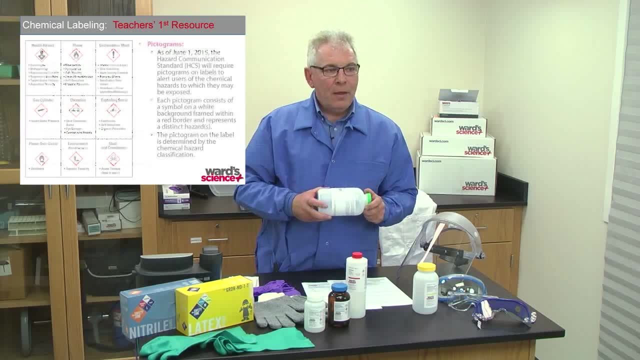 If you're transferring chemicals from one chemical to- I'm sorry- one bottle to another bottle, those that bottle that you've transferred to has to be um labels. So on your PowerPoint you're actually going to see on the left-hand side, um, you're gonna see the new icons. 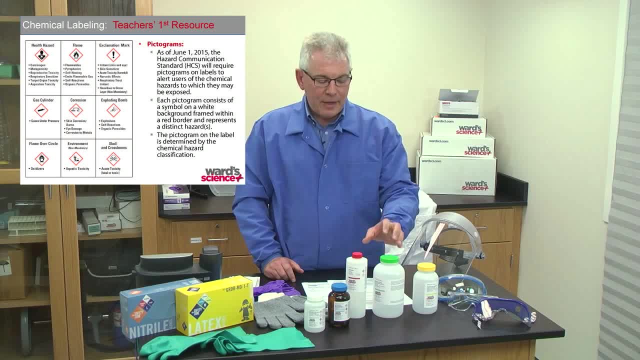 So these are actually picked. The pictograms are designed. they have a red diamond around them. So when you see a pictogram and you may actually have a chemical that has no pictogram so it may not be classified under GHS. So don't worry if you don't have some new chemical. 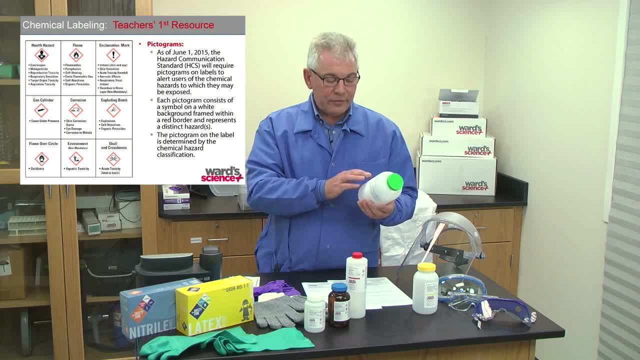 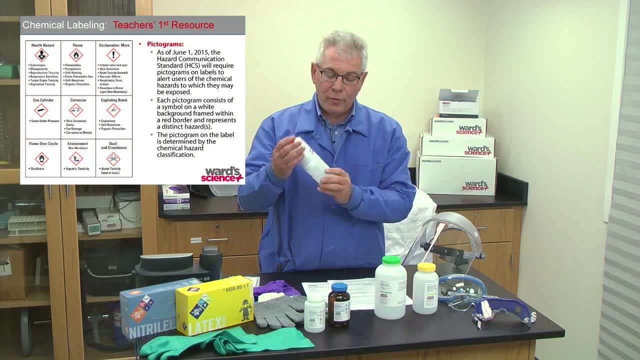 So potato starch- here again, a general storage, and it says this substance is a mixture not classified under GHS. It's not going to have a pictogram next to it, Of course, acetone- it's going to have two pictograms. 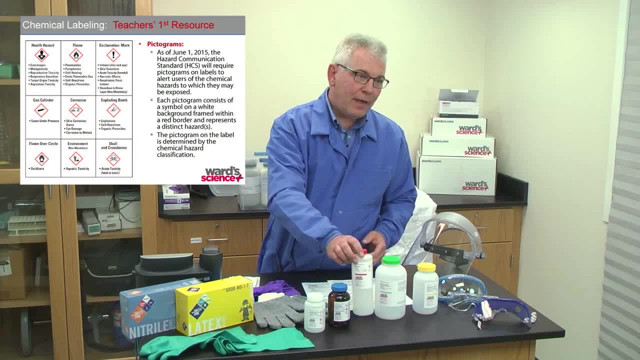 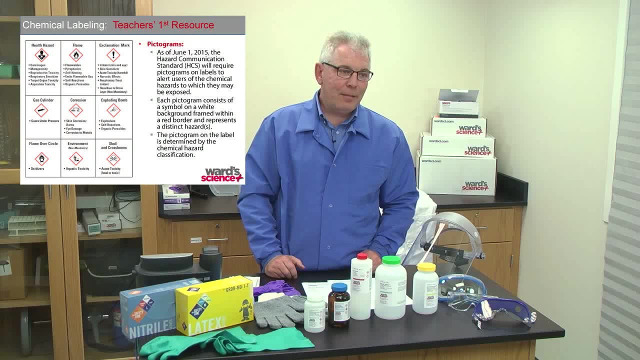 So we have a flammable and exclamation point. So the different Health. there's different pictograms around those warnings, but they're good. when you see the red diamond, that's actually going to give you a heads up ahead of time that you might want to read that label here again. 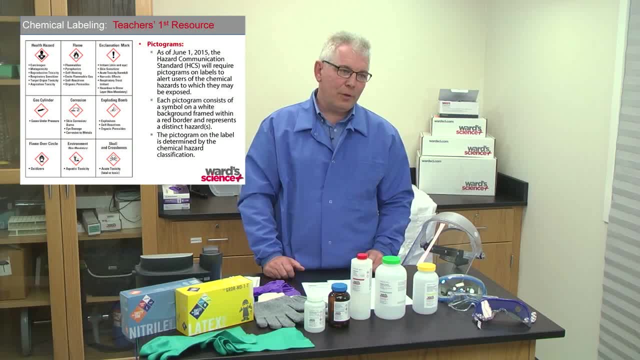 We've should always read it, but the idea around the GHS, or the globally harmonized system, is it's actually going to create a safer workplace or laboratory for you. So the nine that you have to worry about: um, we have a, and I call it the little running man with a, and it's got a lung there per se. um, the health hazard, and that can really be. 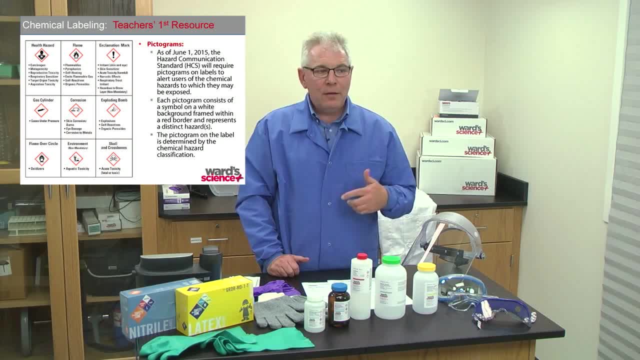 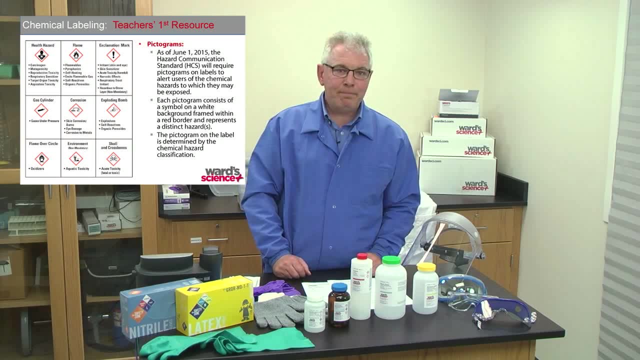 Any Thing in the sense of a teratogen can go back, So it can be a teratogen at the same time. Flower also has that same um health hazard. So in an industrial setting a flower in a mill um is a dust hazard. 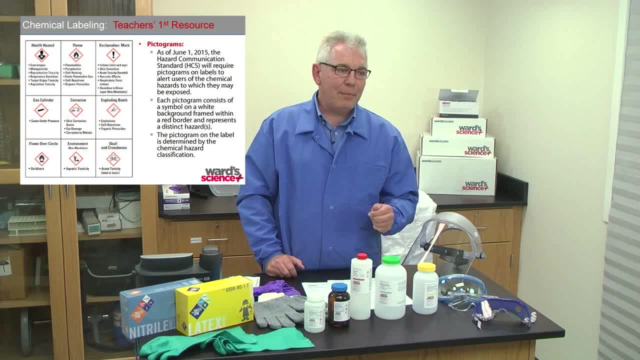 So it also has, uh, an inhalation dust hazard. Um. there's a flammable symbol and exclamation point. There's a gas cylinder as a corrosive um or corrosion uh diamond. There is an exploding bomb. 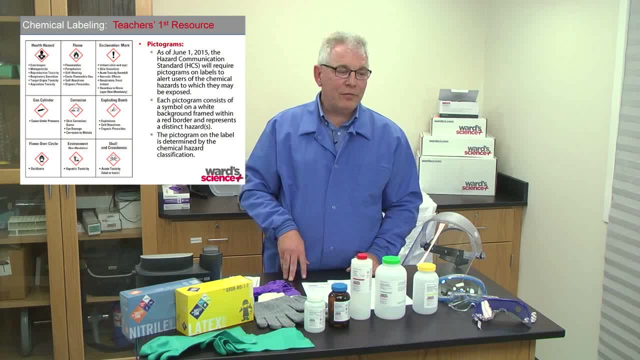 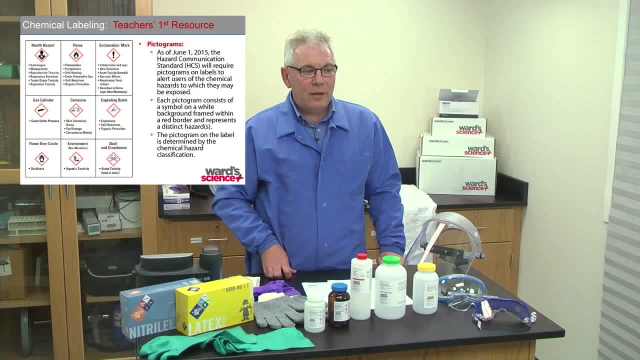 There is a flammable flame over a circle. Now, This Is the one. it's an oxidizer And this is the one that gets most confused with the flame. The difference is the oxidizer has a little circle with a flame on top. 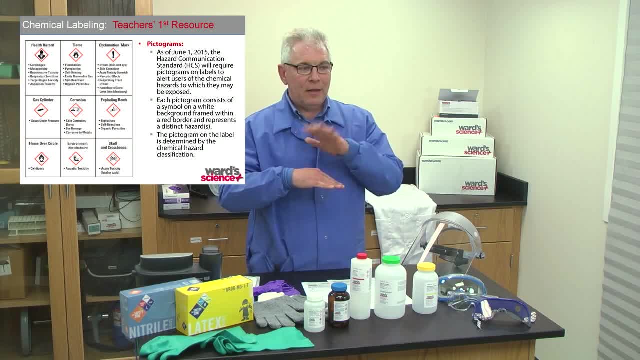 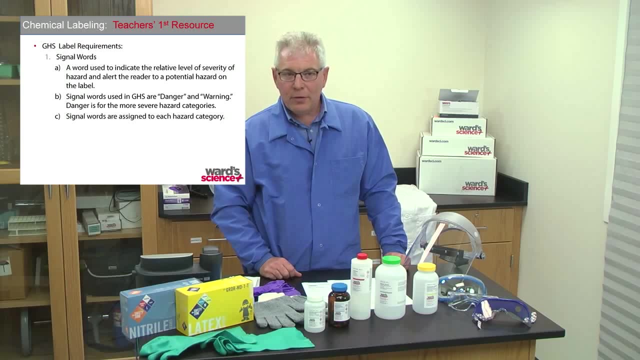 So that for oxidizer in the flame, if you look, is a straight line with a flame above it. then there's a uh- aquatic toxicity- and then a skull and crossbones next. So here again you may have products that's in your um lab or your. 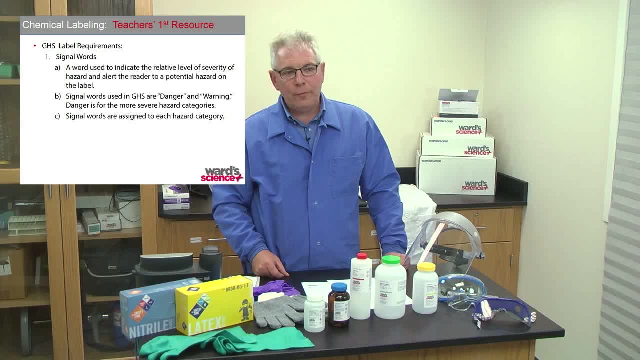 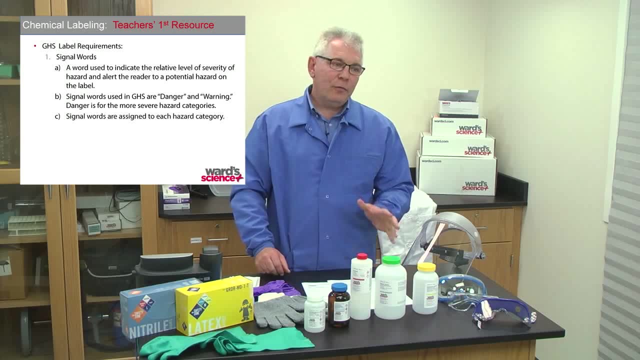 School That may have been manufactured previous to uh January 1st 2015,, those labels, still um, can be in existence. The changeover again occurs in January- sorry, June 2016,, where all of the labels have to be in your lab, have to be converted to the new GHS uh format. 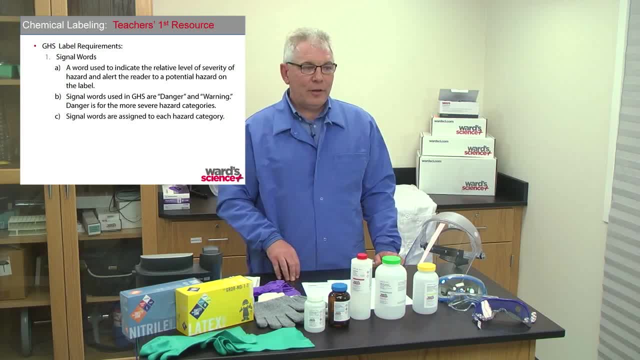 Let's go over some of the GHS label requirements So we have a signal word. So that signal word is that danger warning. You'll see that a lot of chemicals today are the main. same chemical You might Use yesterday might have a different warning or signal on it word that it was yesterday. 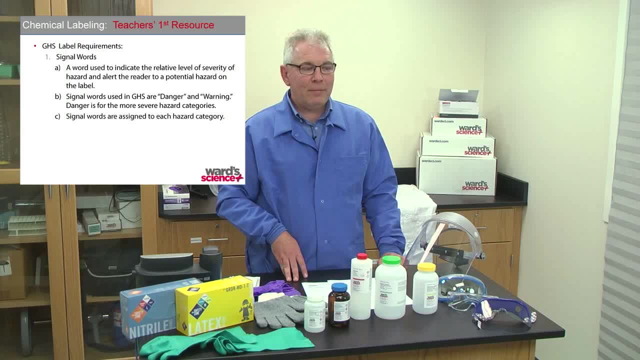 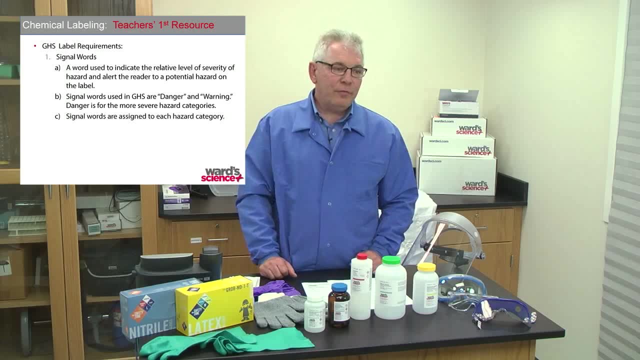 So you might have seen. caution, If you bought something last year, it might be warning or danger this year. Here again, chemicals have been classified under GHS, And so there you might be a more severe hazard than you've seen You're used to seeing. here again, that's supposed to make you step back and read the label. 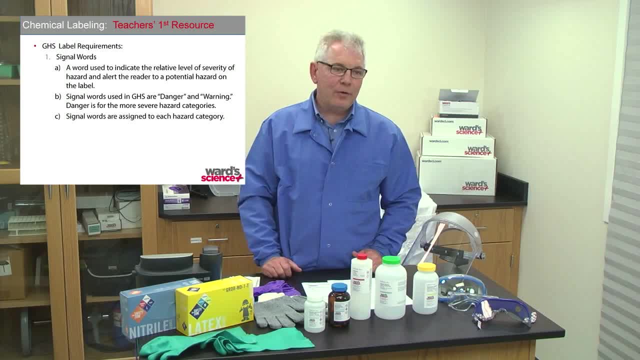 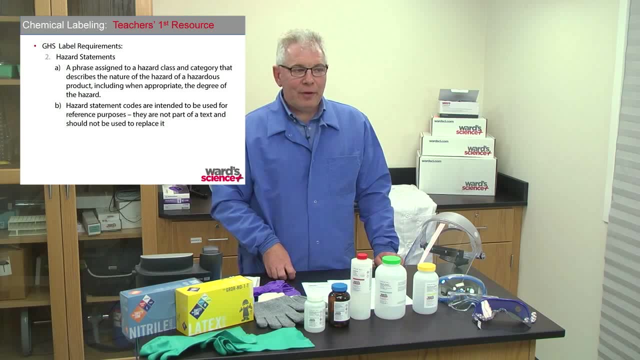 Nothing's really changed in the chemical composition, It's just how it's been classified. Next, please, So the other GHS requirements. we have hazard statements, So these are phrases that are assigned to the hazard class or category, and then we have hazard statement codes. 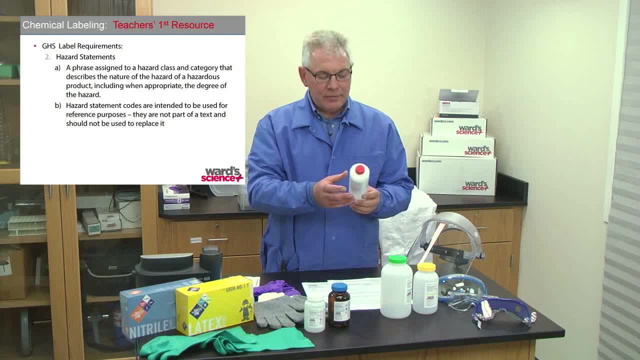 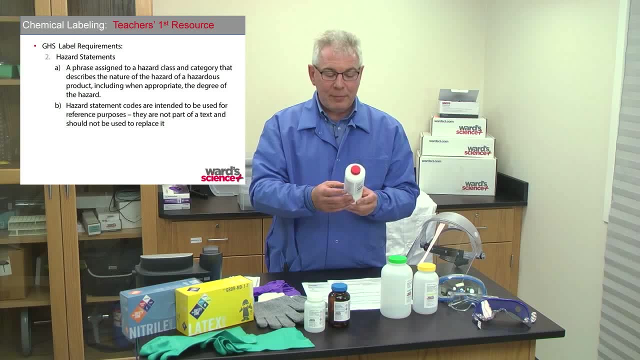 So it can get very uh wordy or robust on these labels. So here again, this is acetone and it's hard to see on the label, but it's filled with a lot of words. So danger: highly flammable liquid causes eye series, eye irritation. 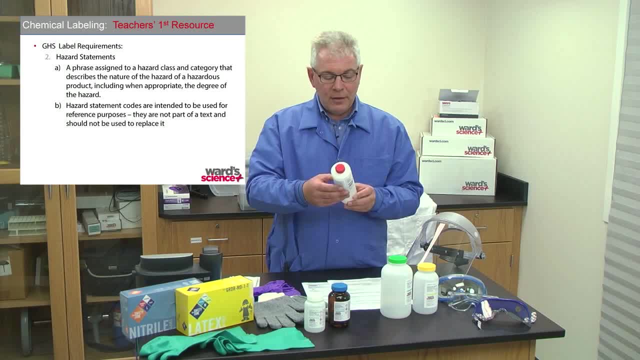 And there's a lot of words that are going to go through. what happens if you get it on a skin? Um, what happens if you get it on in your eyes? what are the things that we have We'll worry about before we use the chemical. 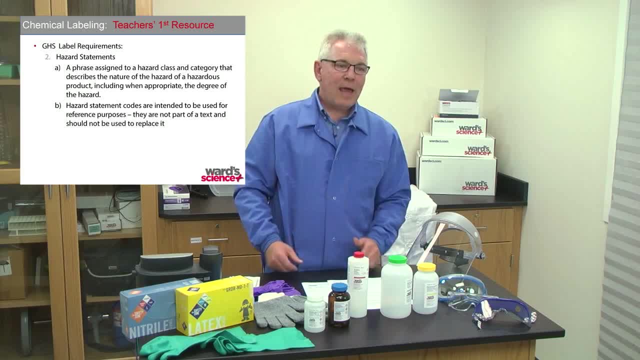 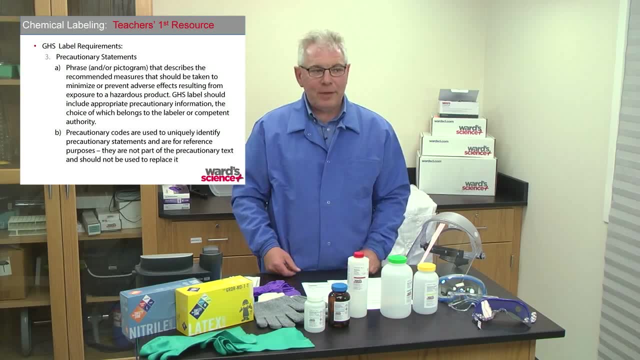 So here again, more robust labels that you're going to find today that you have in the past. Next, please, Precautionary statements. So these are phrases, or they're called, sometimes called P phrases, And those are phrases or pictogram: the phrase, the end of the pictogram that describes the recommended measures that really are used to minimize the adverse effects around the using the product. 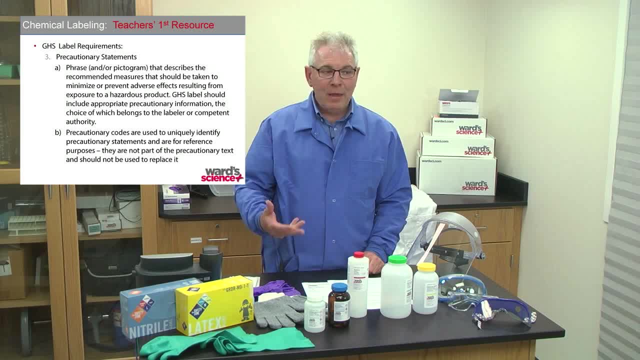 So a GHS label is going to have those precautionary information ahead of time. Here again, if you are making your own chemicals in that life and for your lab and storing them into your overnight, um, you'll have to do the same thing. 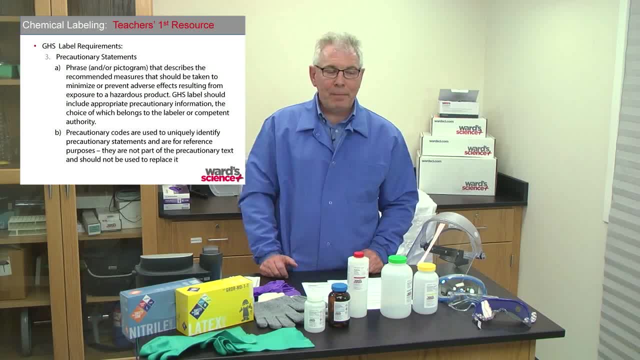 You'll have to classify and also label your own chemicals. in the past, Um, you might've been able to just put it on the shelf. you know, one N HCL, one normal edge edge cork acid. Those have to have now, have to have um, all the P and H phrases ahead of time. 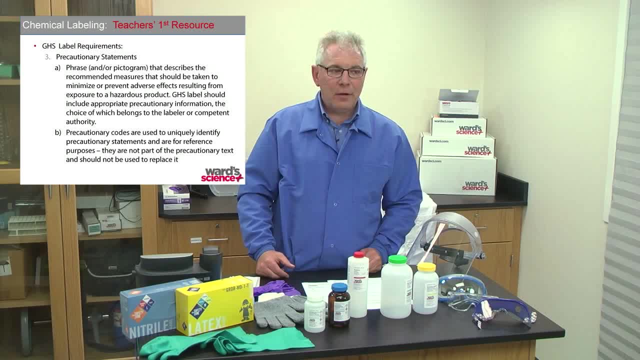 If you're going to make your own products. not a lot of teachers are um have the time to come in at five o'clock in the morning anymore. Like some of my old teachers, um, they used to make all their stuff ahead of time. 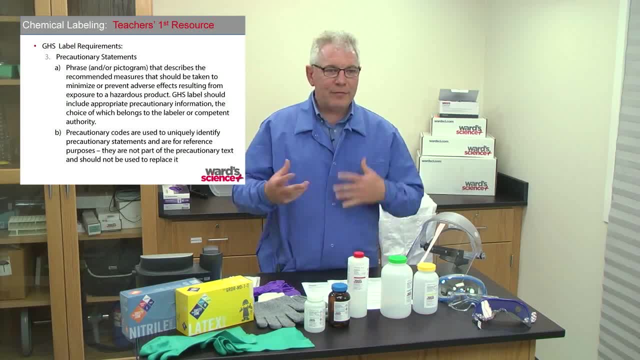 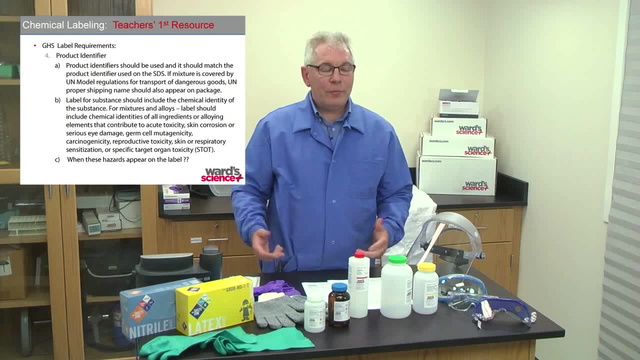 Um, those are. it's a little harder to do that today with all the different testings and things that are going on in the classroom. Next, please. So some other um GHS label requirements we want to talk about. So, product identifiers: we have to worry about what the product is. 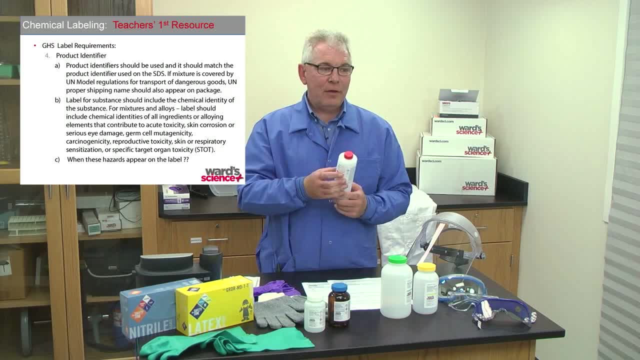 So there's an identifier- Yeah, this is acetone and we actually have to have a UN number around that- And then we want to make sure that the chemical identity is there. And there's also there might be some uh mixtures or alloys that might be on a mixture that we have to identify. 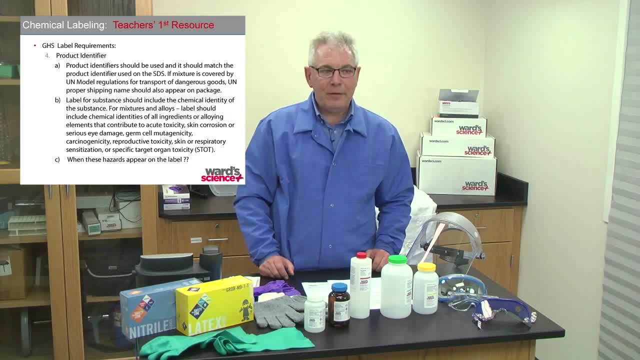 So, um, there are other hazards that might be there in those mixtures. Those are usually going to occur. You'll see it on a label, but also under the contents, but under the STS too. Next, please, Supplier information here again. in the past it wasn't a requirement, is today. 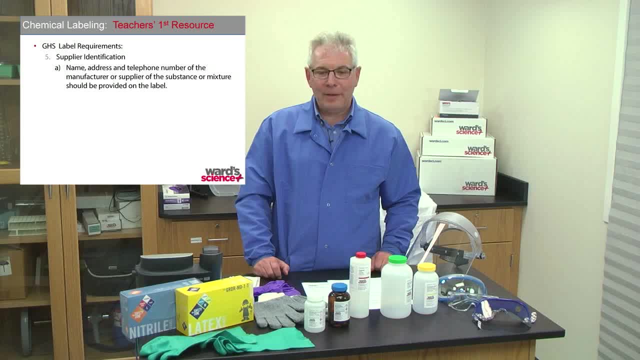 So name, address, telephone number and manufacturer, supplier has to be on the label. If you're making your own chemicals under GHS, you actually You become a chemical manufacturer and you would have to put your name or your school's names as that person making the chemicals. 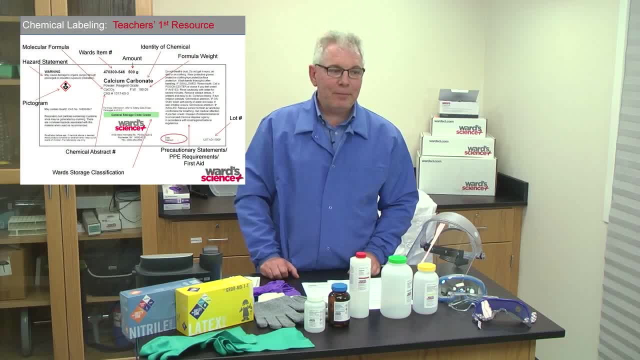 Next, please. So here's a pretty robust label. This is only calcium carbonate, but you can see there are a lot of H and P phrases here. There is a um warning and there is a pictogram around that. So even though um you would think calcium carbonate is pretty innate, there could have quartz in it. 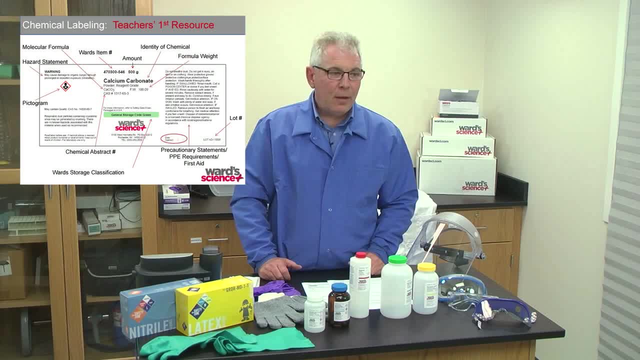 And so there- that's why it has a warning- um. here again you can see Wards science, the chemical abstract number, the um catalog number, the amount and the formula around there and the lower right hand side, you'll see a lot number. 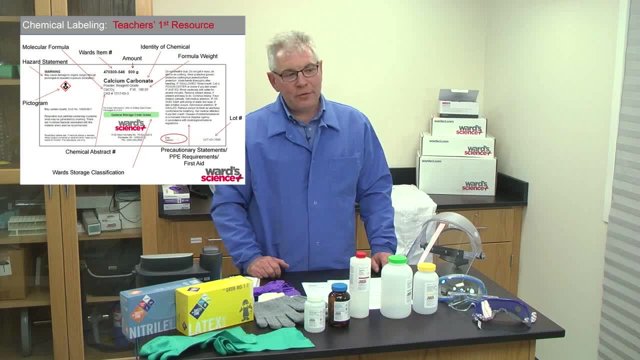 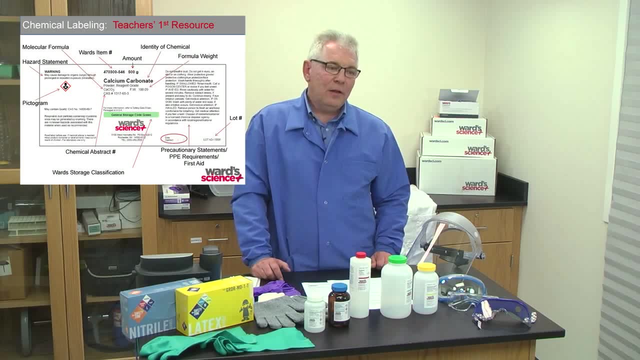 So if you want to- the cheating way to learn how to read these lot numbers, so you can see an ad and I think it says one: three, zero, zero, zero. So the uh boards uses a Julian date. So the first digit is 2013 and there would be a three digit code after that. 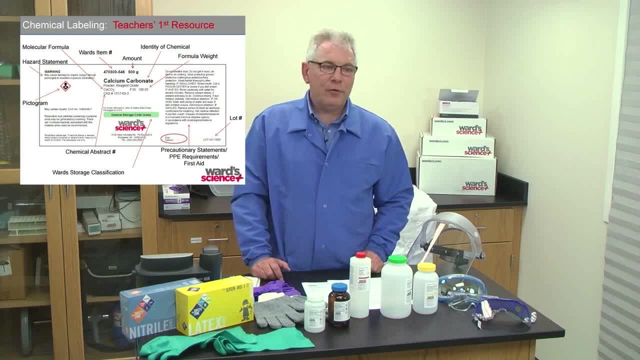 So if it was Uh 13,. zero, zero one, It'd be January 1st 2013.. Uh, yeah, uh, it would be January 1st 2013.. Uh, it would be January 1st 2013.. 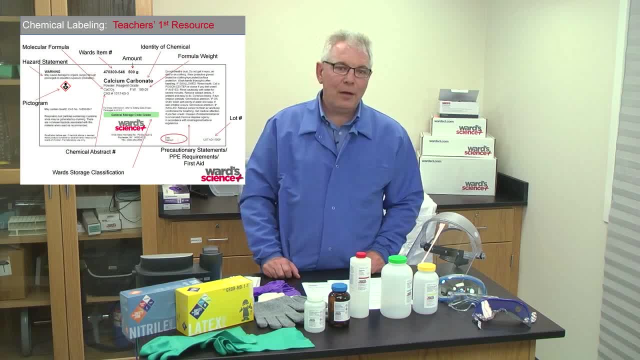 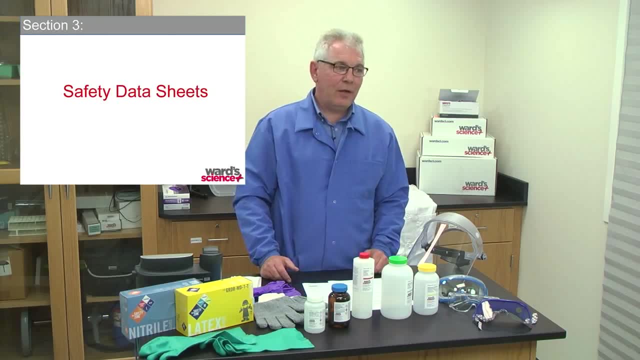 2013 is when it was manufactured, So you can see the manufacture date of the product when the board manufactures it. Next, please, Safety data sheets. So here's our. so here's a secondary section around. first part is our labels. 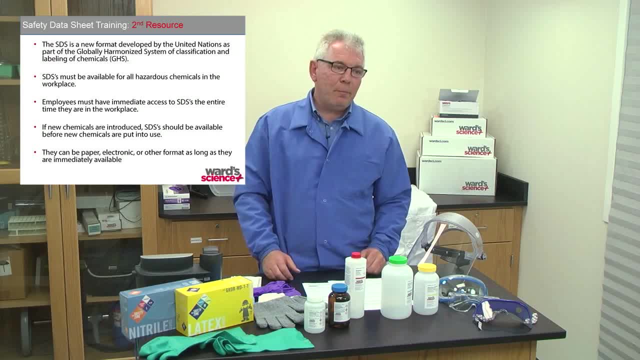 the second part is safety data sheets Next. So there's 16 different parts of the safety data sheet Next. So we want to worry about, so the safety data sheet. this is a new format, So all of these safety data sheets. 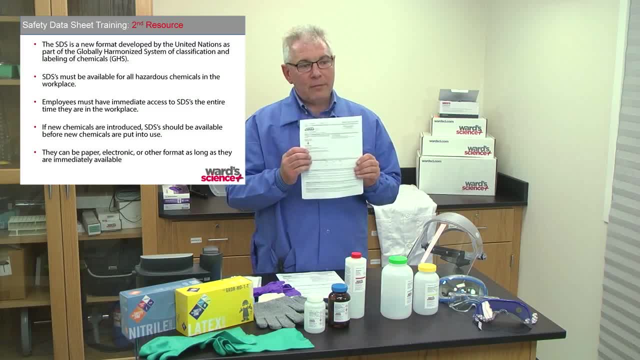 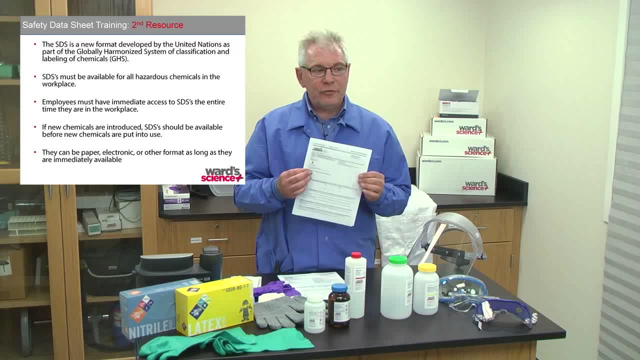 so we have there's- you're gonna get there's- e-files today that occur on the awards website. In fact you'll see both for Canada, French and then English for the US. So you see a four page sheet. 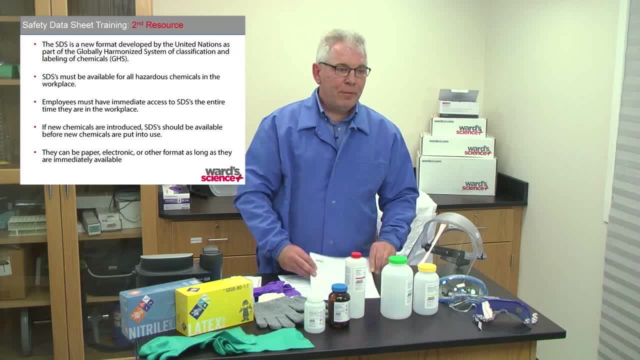 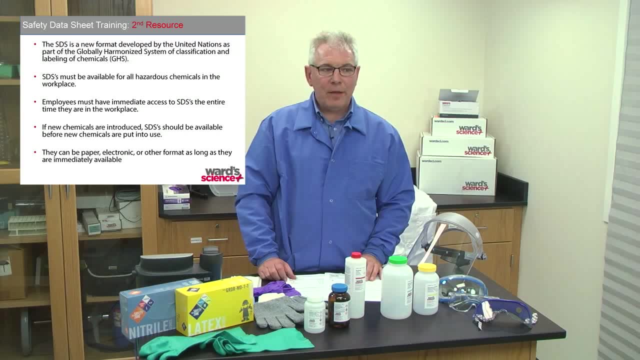 Here in the US it would be a two page sheet. You have to have those SDSs that have to be available So you can have those on an internet site or some kind of a network at your school. You may just want to print it out. 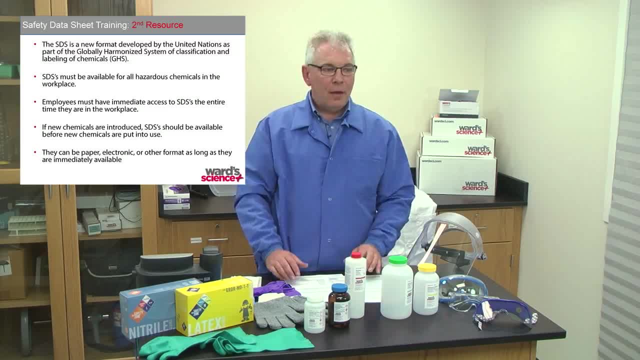 and have it as a paper file. So there's two different ways you do it. You just want to make sure that you they're immediately available. They are in a section or part of your school where you can get to them If you use the awards chemical inventory management system. 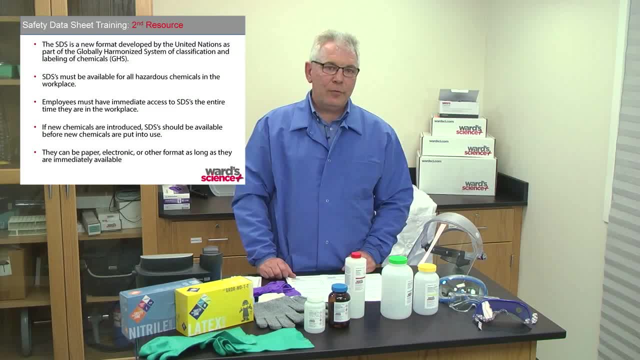 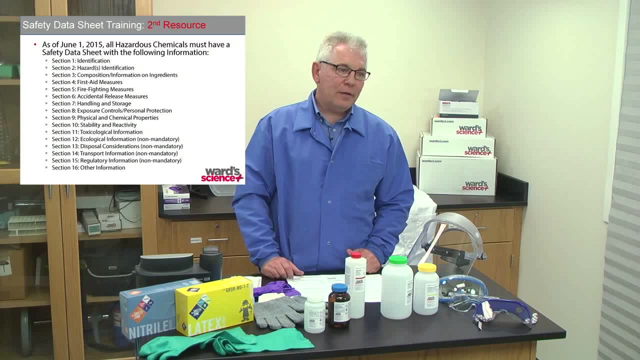 those are all on a cloud and you could actually access those anywhere with your chemical inventory Next. So let's look at some of the first part. So you're seeing the first part of that chemical SDS. So you can see on the left hand side. 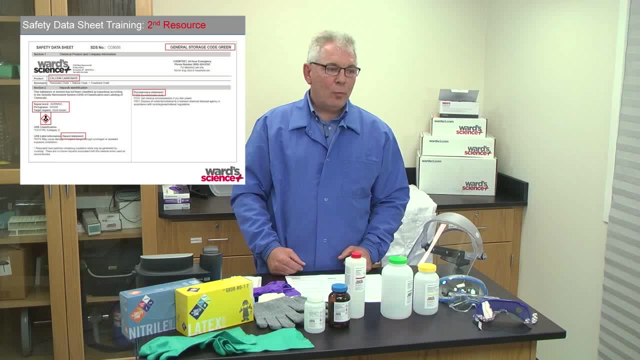 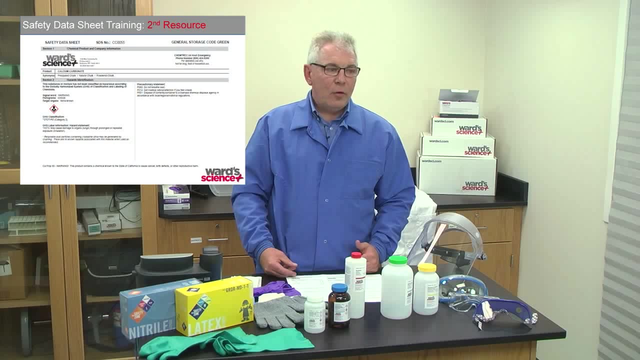 you're going to see calcium carbonate. you're going to see the pictogram, the warning symbols and some information around that. Next We're going to go through all these 16 parts of the SDS. So in section one you have the identifier. 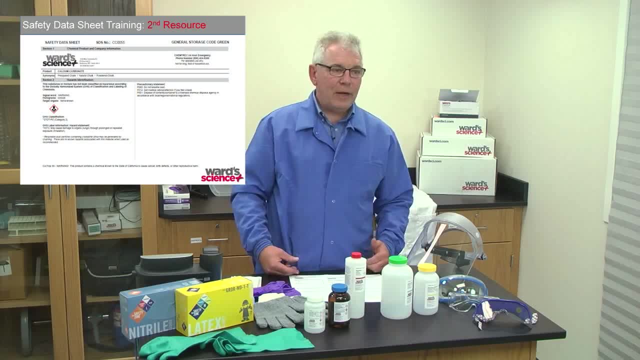 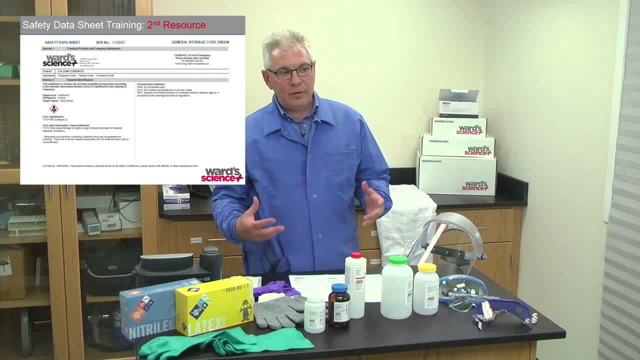 of who that manufacturer was. In section two you're going to have all the health information around the chemical. So you want to look at number one and number two first. So number two is probably the most important, with number one being the name of the chemical. 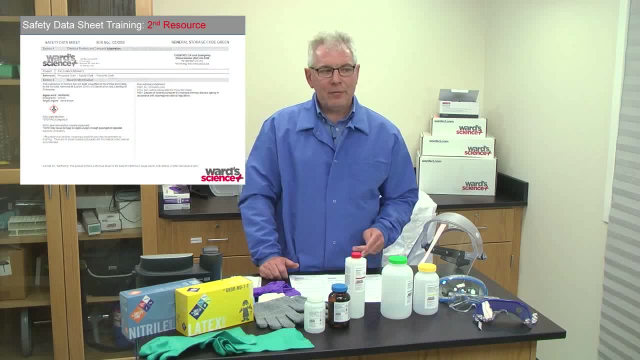 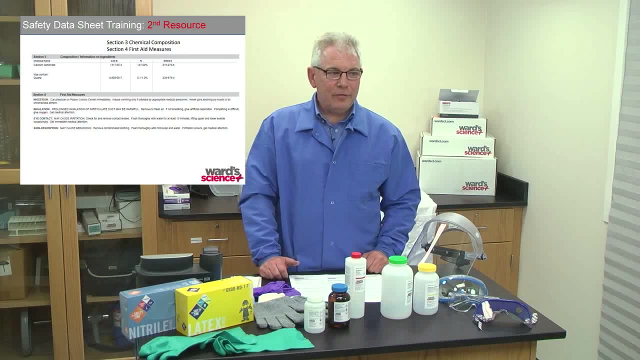 Number two is: what are the things I need to worry about Next? So in section three we have a chemical composition, So you're not going to see a lot of trade secrets like you might have had in the past. People used to try to hide formulations. 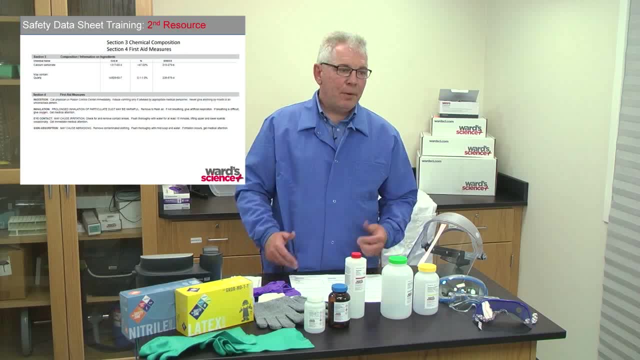 There are trade secrets that are allowed under GHS, but you really have to spell out some of the compositions of the chemicals and the ingredients around those And you'll see the composition percentages And below that you're going to see some first aid measures. 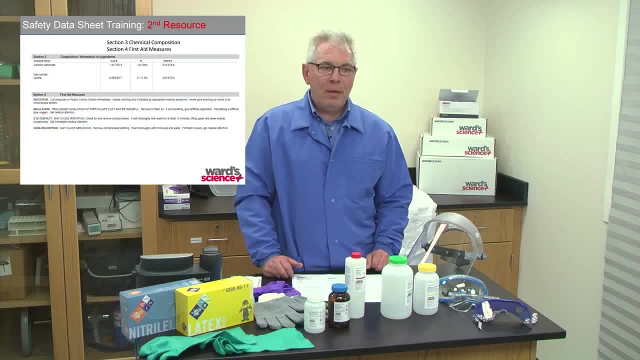 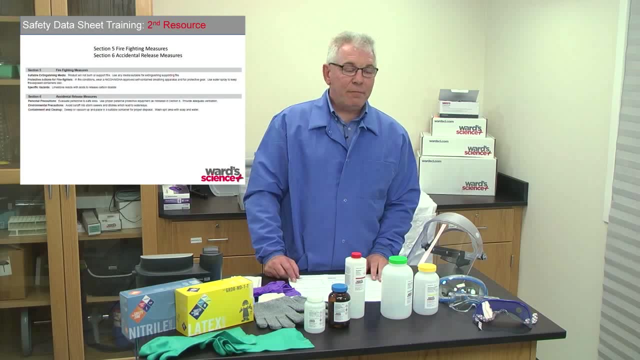 So here again, an important part of first aid. You want to read that ahead of time. What happens if somebody comes in contact with a chemical? Next, please, Section five is our firefighting procedures, Here again as teachers, lab administrators. 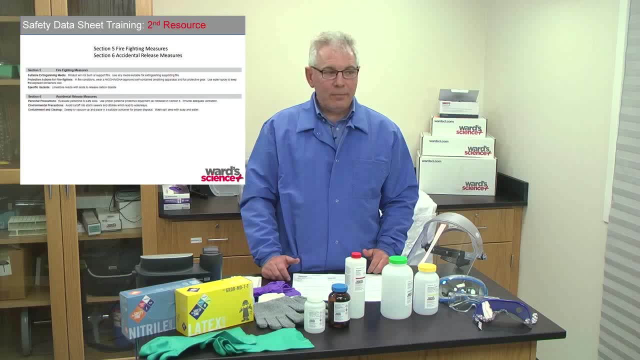 we aren't firefighters, So there is some common information there, but a firefighter is going to want You may be trained. And here again, if you are trained to use a firefighter, you have to make sure that you're trained on an annual basis. 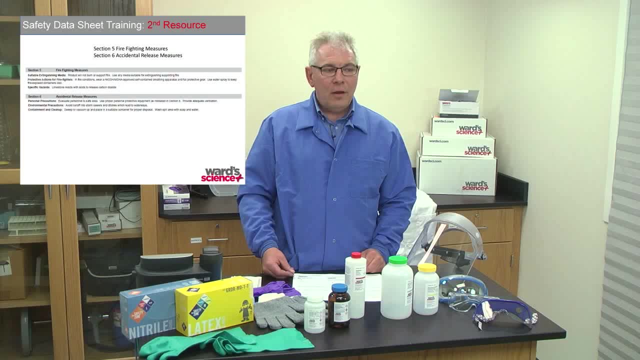 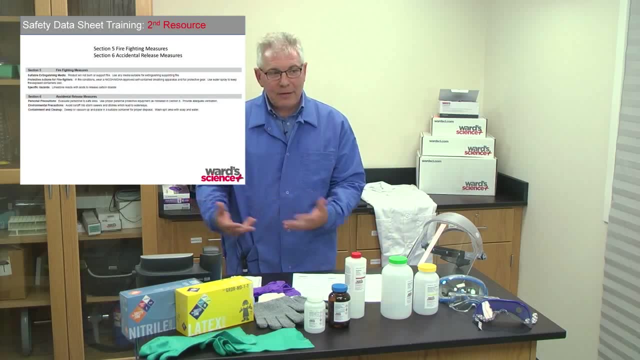 You can't just say, hey, I can use a fire extinguisher. That is training that your employer has to provide to you. Section six is accidental release measures. So what happens if I spill it Here again? it's nice to read that ahead of time. 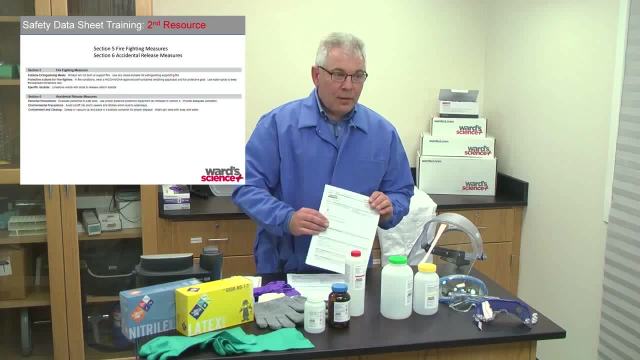 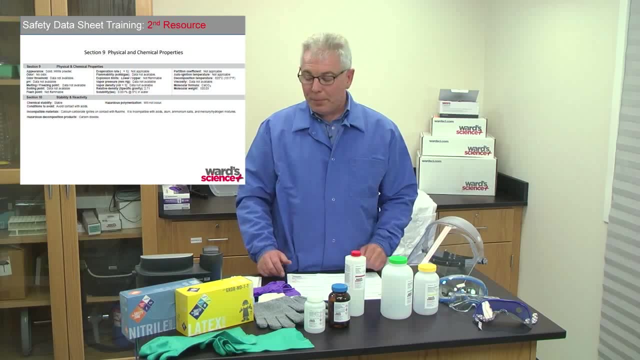 that we can actually read the SDS Next Section nine here: physical and chemical properties. Great thing you can do. So if you want to run a coolant, Coolant. You want to experiment with your students, They can Google a lot of things around the composition. 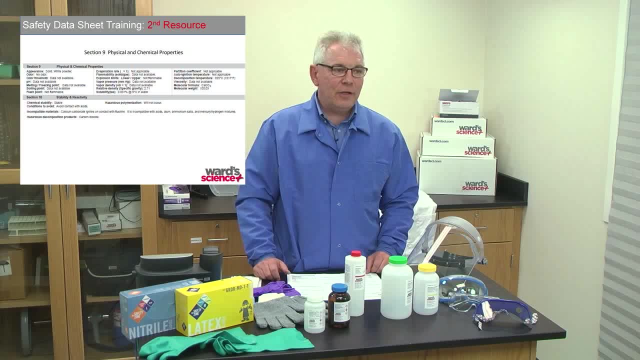 or the physical characteristics of a chemical. At the same time, they can actually use the SDS to look at what is the melting point, what's the freezing point, So you can get a lot out of that section nine, And then section 10 is going to be that's. 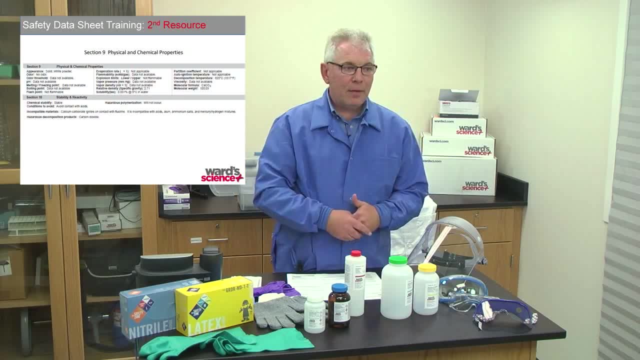 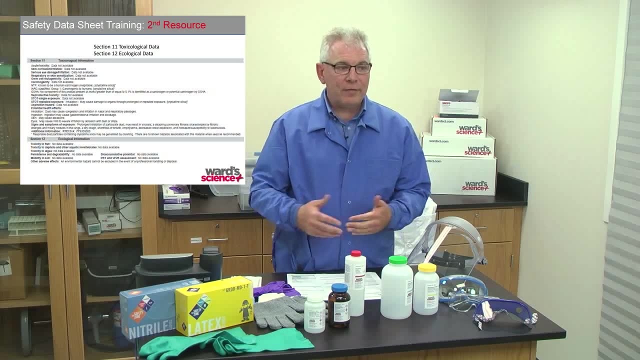 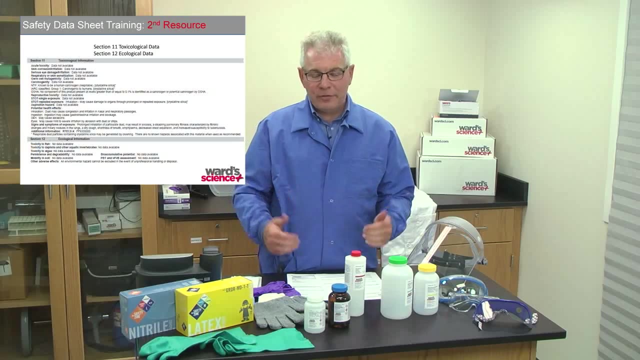 stability, sorry, solubility- of the chemical. Next Section 11 is toxicological data. So the more hazardous it's a chemical, the more toxicological data that's to be there. now that's kind of where you start. beyond that in section 12, osha doesn't care. 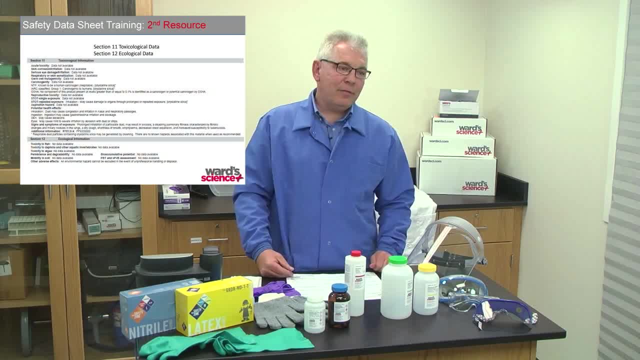 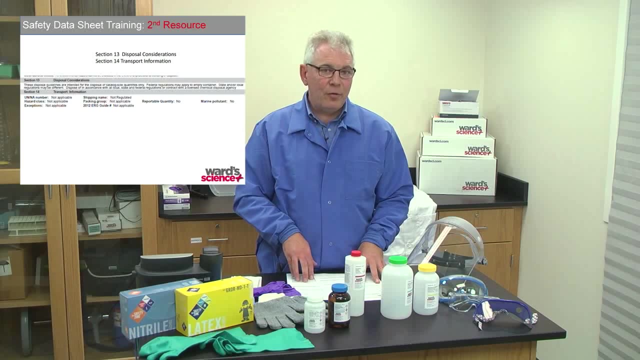 anymore, but other people do so. the epa worries about section 12, or ecological data of the chemical. what happens if it's released into the environment? next section 13 is our disposal considerations and of course, 14 is transport. so remember, if we're taking a chemical, that's. 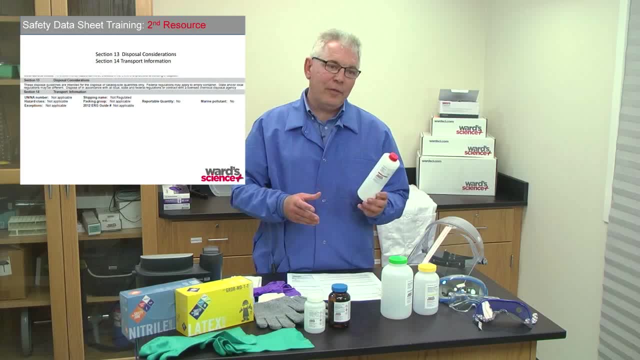 hazardous putting it in our car and going to another school. we want to make sure that one it's. you have to be trained or certified to do that. you can't just put it on the road and go down the road with a chemical. so there is transport information around shipping a hazardous material. 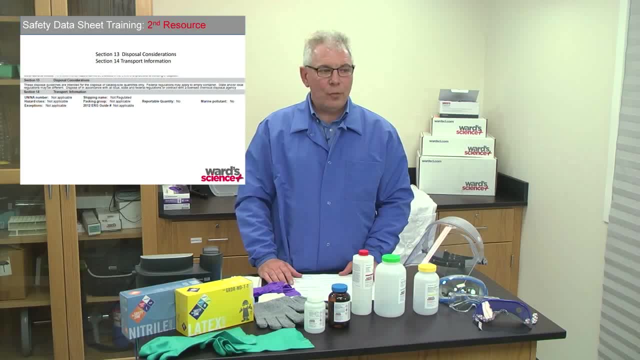 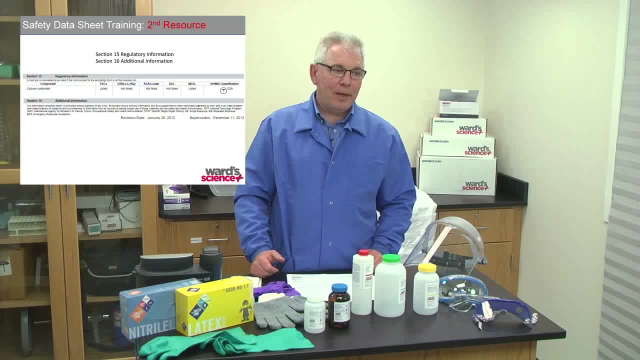 versus a non-regulated product the ot doesn't worry about. next, section 15 is just other regulatory information. it might be around some local federal laws around circla or rickra. there's rickra codes around. so if you're getting hazardous getting ready, hazardous race, sometimes um safety clean or different companies might ask. 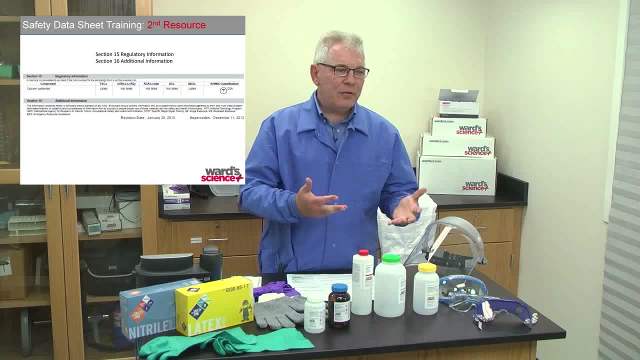 what is the rickra code or the chemical you're trying to get rid of, and then there's some additional information under 16.. so all those safety data sheets have to have 16 parts as as part of the new guidance. in the past it was as low as eight or nine, and now they have. 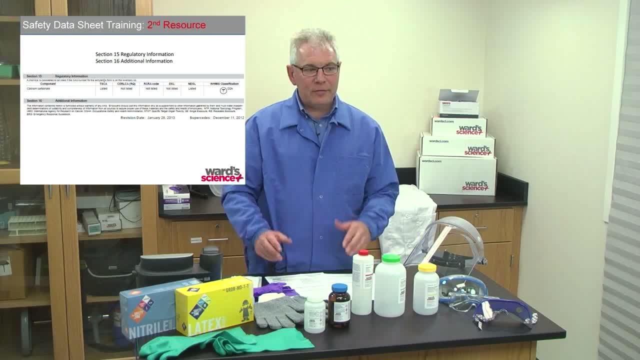 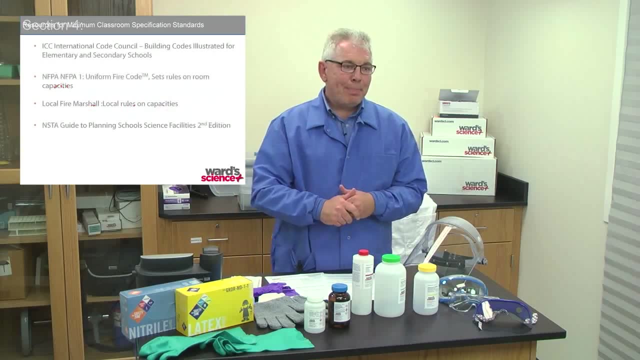 to have 16 parts to be compliant. so all sds's have to have 16 parts. next, so classroom and laboratory specifications. so, um, next, so we don't worry about you. know our classroom, so there are some guidelines around. you know the right classroom. you might make sure if you're reading or you're. 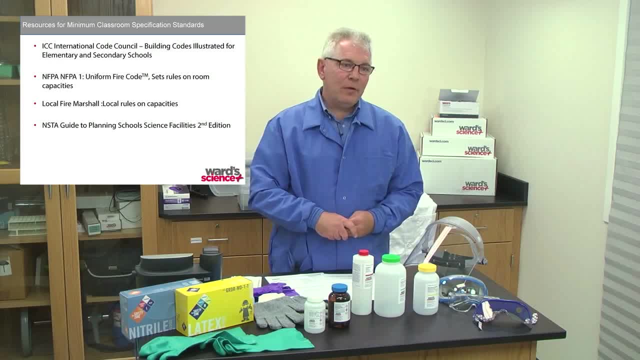 planning for the future. here again it's lifelong learning. sometimes we might be put into a classroom that might have been the music room. it's might have changed. so as you get an opportunity in the future to build a new classroom or there might be budget dollars available, we want to make sure that you know people are reading the icc international code. 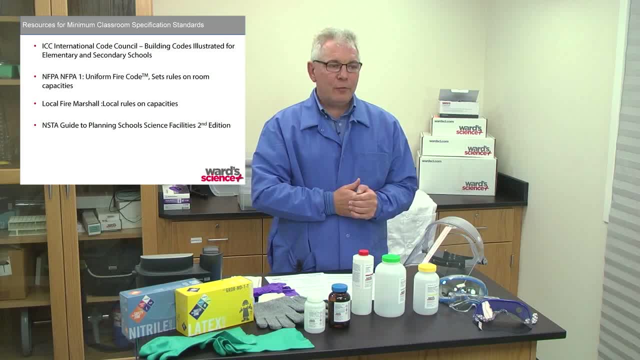 around that. there are some nfpa guidelines or uniform fire code that set some room capacities, and there are your local fire marshals. a great um can be great help. nsta also publishes a guide on planning schools and science or facilities in their second edition, and they actually have. 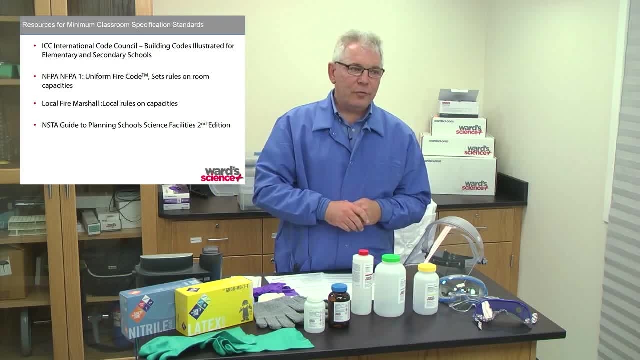 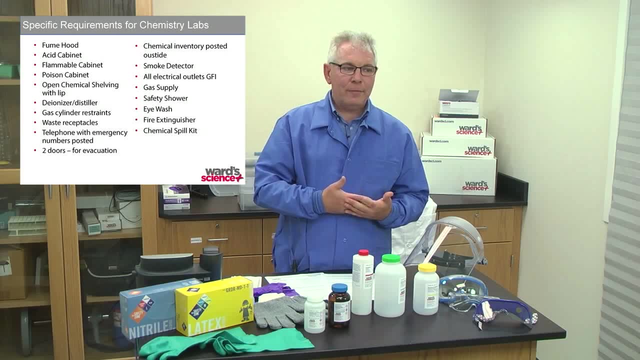 some guidelines around what they feel is ideal square footage for a classroom. here again, here's an ideal classroom. so if you had a chemistry classroom, you know we want to make sure. do we have a fume hood? do we have an acid cabinet? do we have a flammable cabinet, a poison cabinet? you know there is open chemical. 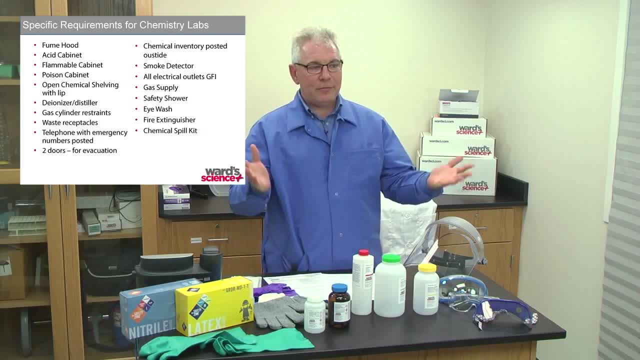 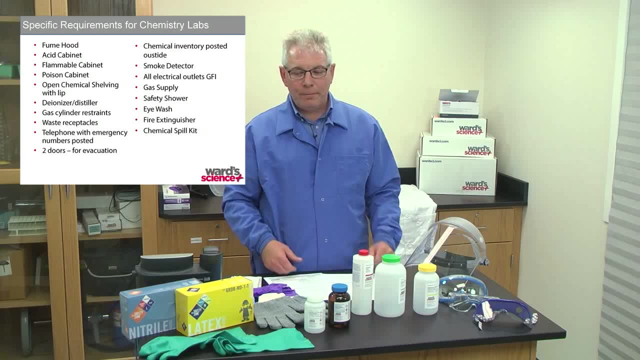 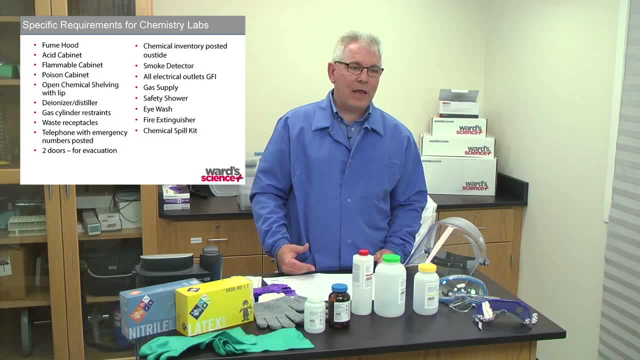 shelving with a lip if you're in the state of california, we, that is has to be a closed situation here again. deionizer distiller for our lab. these are. you know, some of these are just ideal things. you want to have glass gas cylinders if you have gas cylinders in the classroom. 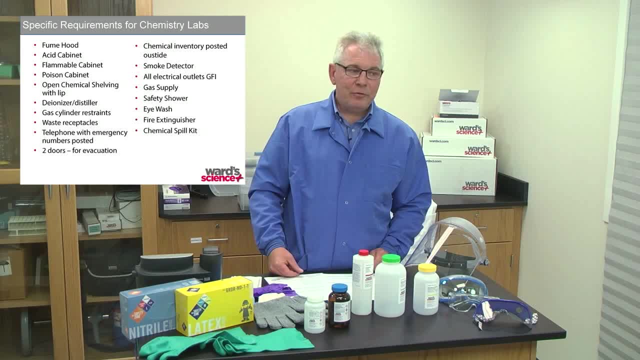 we want to make sure that they're restrained to the wall. we want to make sure we have the right waste receptacles. telephone numbers with emergency numbers are posted. it's really tough when you get into a situation and in an emergency and trying to look for a number. ideally you would have two doors. 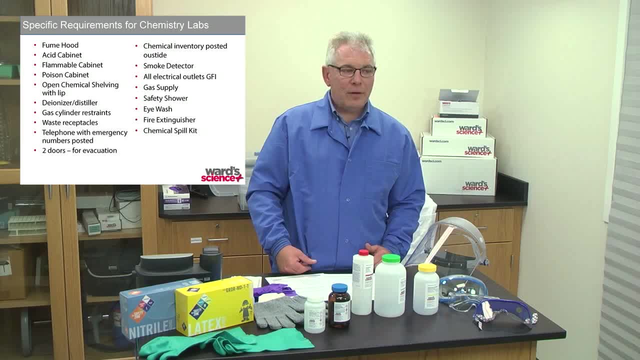 not a lot of classrooms have that or even lab settings, but you want to also have that chemical inventory, so it's posted outside or posted on the or the main might be in the main part of the school, someplace where you can get it other than maybe. 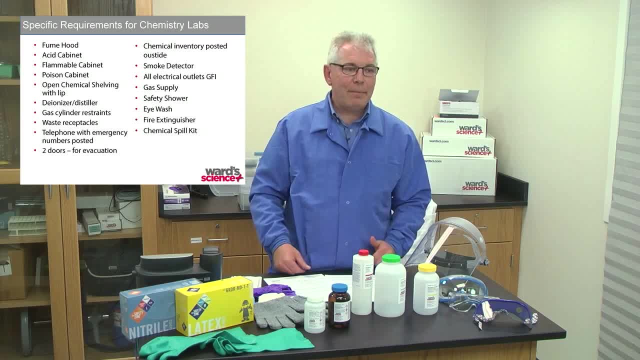 in that chemical storage room or in a some place where something happens. smoke detector, gfi, of course, even a biology classroom if you are dissecting specimens. it's ideal to have gfi plus gas supplies. we want to make sure that we have a safety storage, a shower. 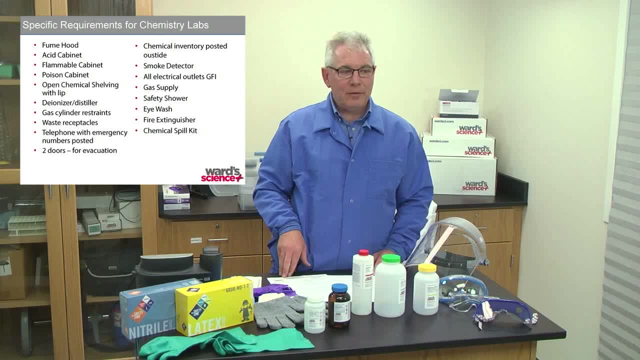 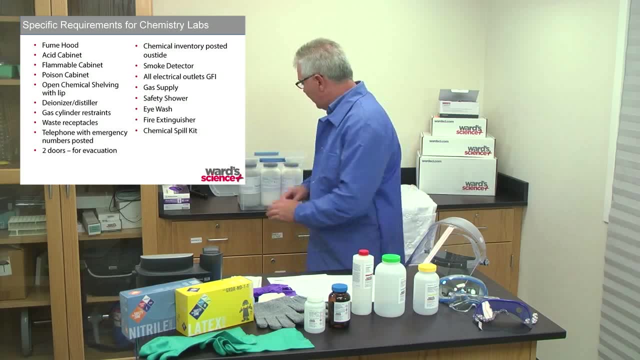 for all of our classrooms. i wash that for 15 minutes fire extinguisher. but here again we have to be trained if we're going to use the fire extinguisher and, of course, a chemical spill kit. so you know, all classes should have a nice little chemical spill kit. they're not, they'll have to be. 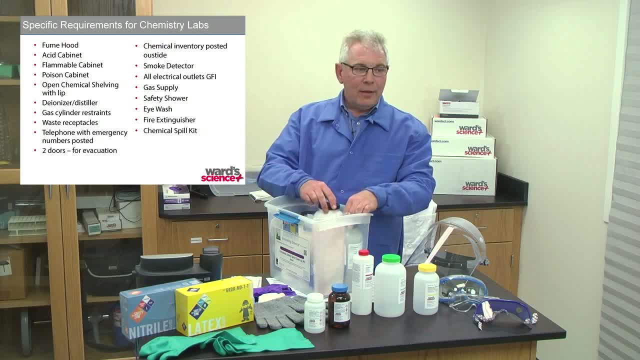 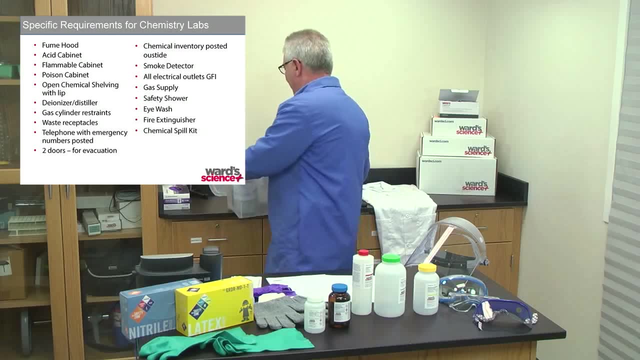 very big, they can sit in, you know, but we want to have, we want to have these ahead of time so if something happens, we can actually deal with that chemical spill as it happens. next piece: so ventilation. so we want to make sure that our room is ventilated, so we want to make 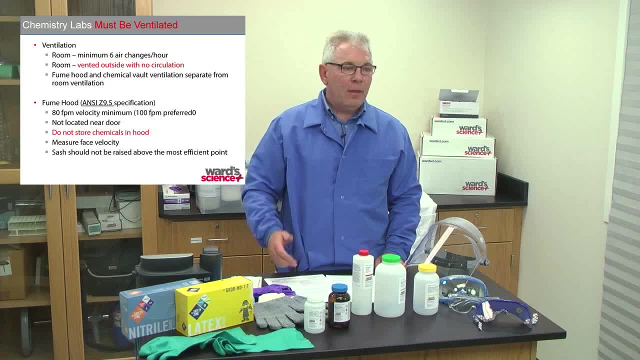 sure we have at least minimum six air changes per hour. with venting, we want to vent outside, so we don't want to have that circulation that goes on inside a fume hood and chemical vault ventilation should be separate than room ventilation and of course, with the fume hood we want to follow the 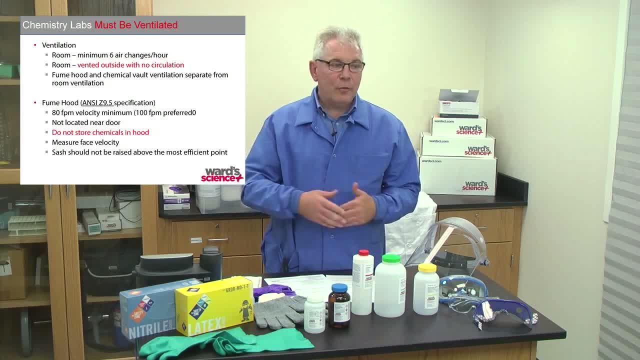 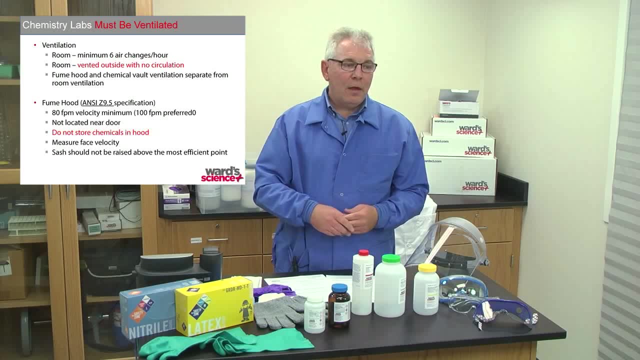 ansi z 9.5 specifications. so we want at least what's called 80 feet per minute of velocity. 100, of course, is preferred. we don't want to locate that near a door and we don't want to store chemicals in our fume hood, so we want to actually have a separate storage area. it's hard to work in. 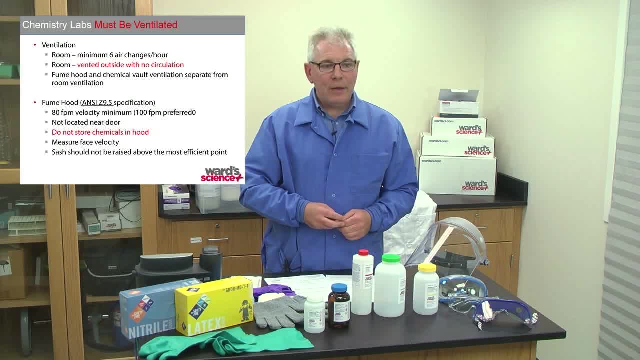 and actually have chemicals in them. here again, your some other teacher might have chemicals stored in there. if you're trying to do a reaction, they might react with what's what's in there. we want to make sure that we're measuring our face velocity every year, so even though the door goes, 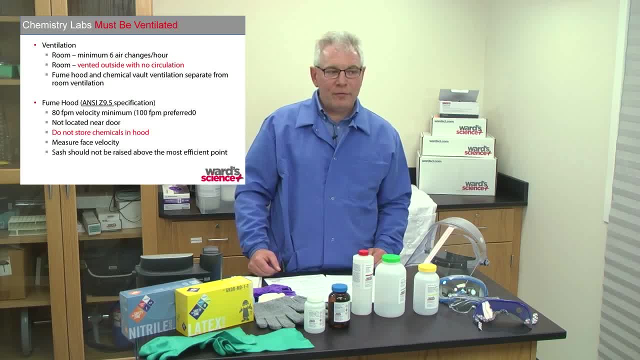 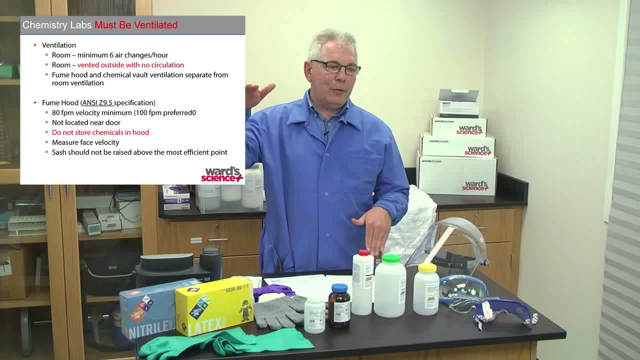 up and or the window goes up and down. we want to make sure that we're measuring the face floss. we know that it's working. there isn't a bird nest, say, in the venting- it's. it's truly, truly working and the sash really shouldn't be raised above the most efficient point. 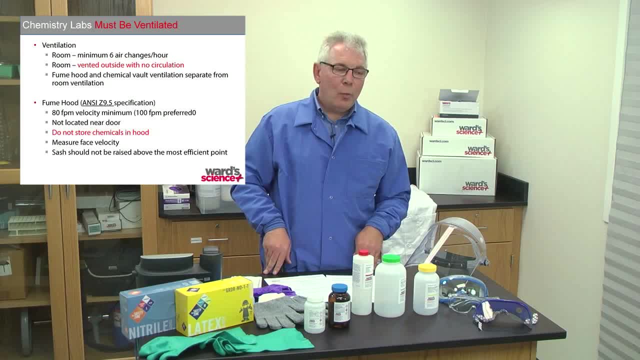 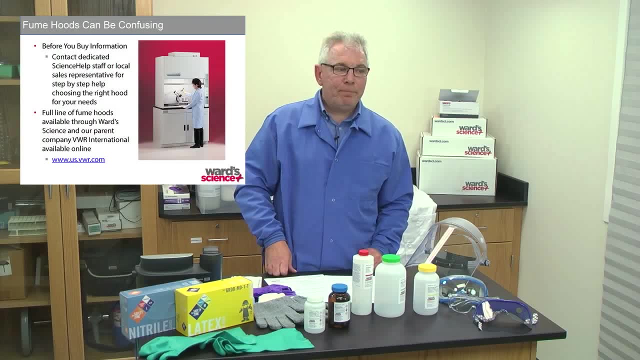 so a lot of times you want to take a little piece of tape or mark off where that most efficient point is. next, please. fume hoods can be confusing. here again, a lot of reps out there can help you with that. there's a simple thing at the bottom: usvwrcom or bwrcom. 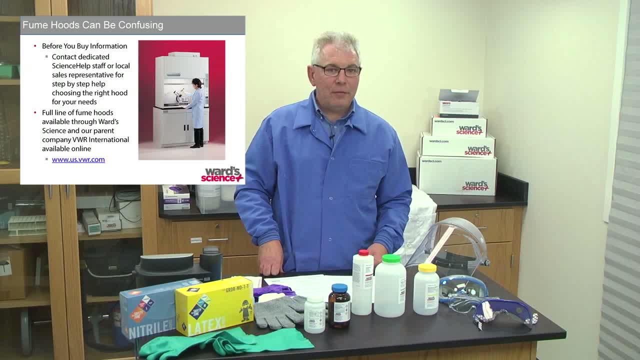 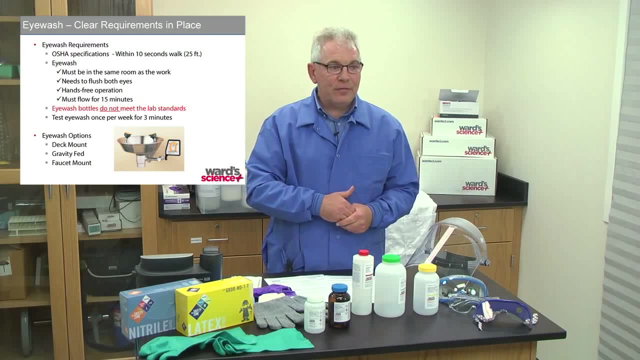 can help you. there's full line of how to look for fume hoods in the future when you're trying to purchase one. but here again, we want to at least have 100 feet per minute next house when you're trying to make an eye wash. so we want to make sure we have an eye wash within. 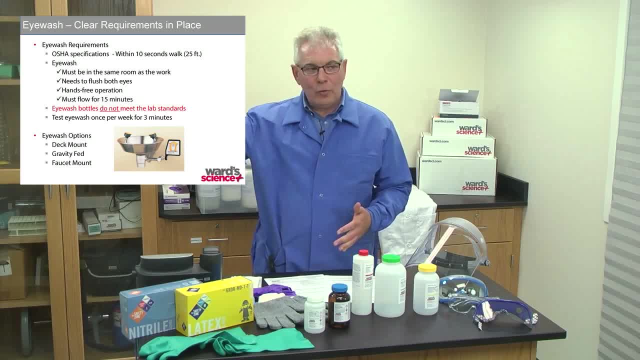 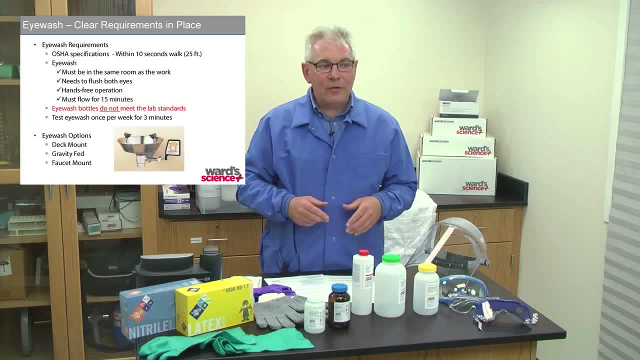 10 seconds of a walk, about 25 feet, in the classroom. we also want to make sure that we're not going out the door and down the hallway to find those, so they surely should be in the room. we want to be able. um, they need to flush both eyes. they also need me. they have to flow for. 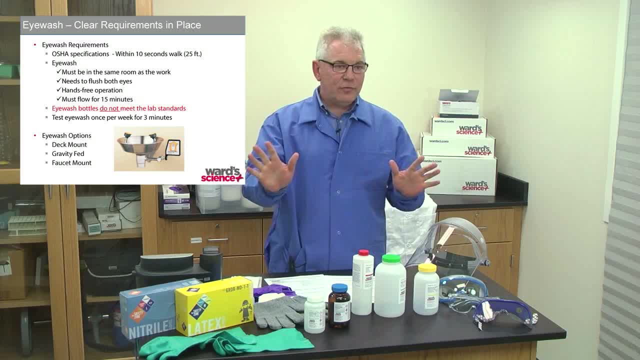 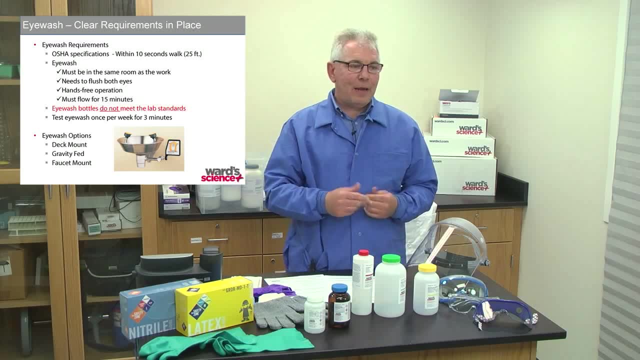 15 minutes and they may need to be hands-on, so if you turn them on you can't just keep the handle on, they have to. just when you turn it on, it stays on for 15 minutes. don't meet the lab standard. We talked a little bit about that And we want to make sure that. 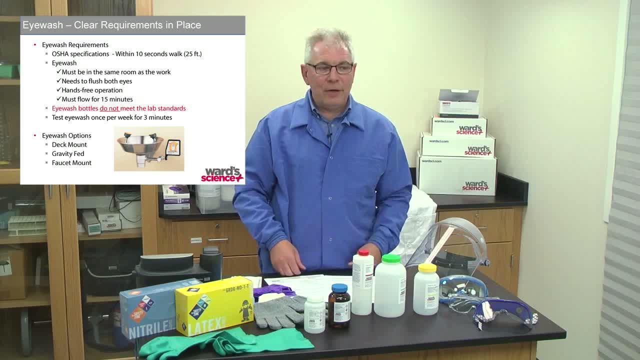 we're testing those eyewashes once a week. One of the reasons around testing those eyewashes is that we want to make sure that they don't just sit all year. They build up bacteria with stagnant water As soon as you turn that eyewash on. the one thing you don't want is you. 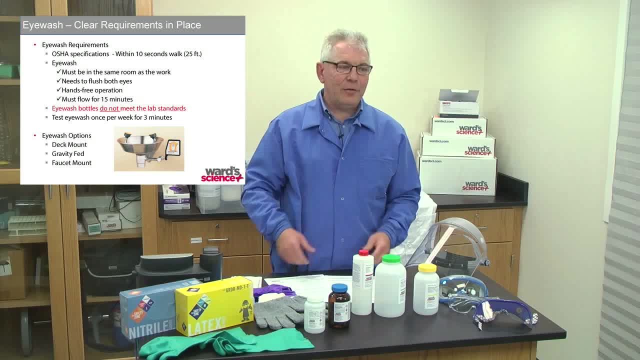 have chemicals in your eyes and you don't want lots of other things in your eyes too. There's a lot of options around eyewash, So they can be deck mount, gravity fed, faucet mount- Here again there's opportunities. if you don't have a plumbed area, There are gravity fed that can fit into your. 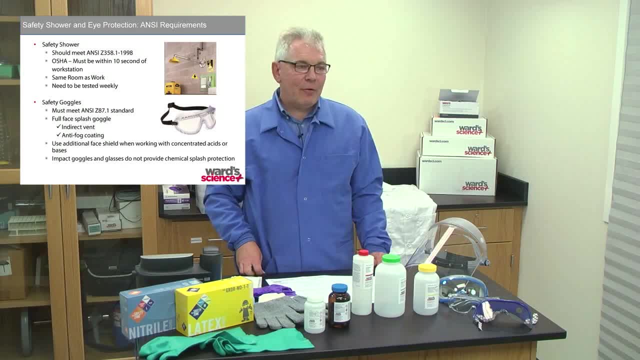 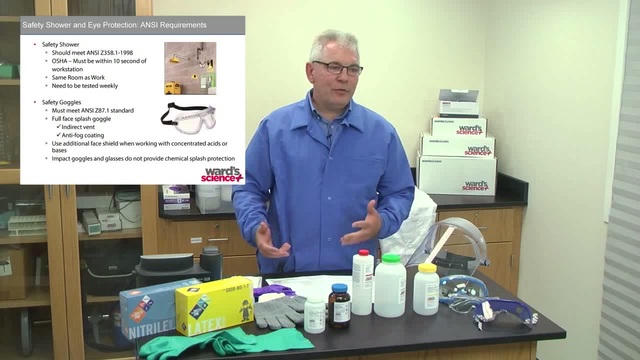 lab, very simplistically, Safety showers. So there's an ANSI standard around that, So they all should have a Z358.1 standard on that. They really should be, you know, ideally within here again, within 10 seconds of where you're working, the same room as work, And they really need to be. 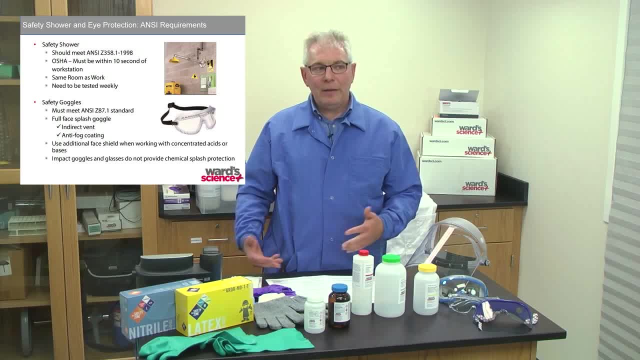 tested on a weekly basis. Here again, I say weekly. Can you test at least monthly? You know, testing, Testing is a good thing. Do they work? Take a pail, put it up there, pull the bottom or pull that handle, And then the handle should stay on. So you shouldn't just pull it and keep it down. 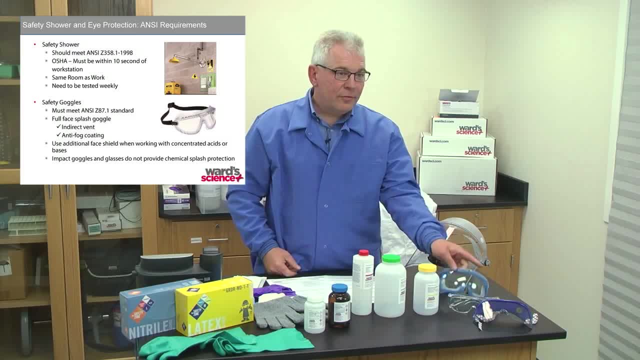 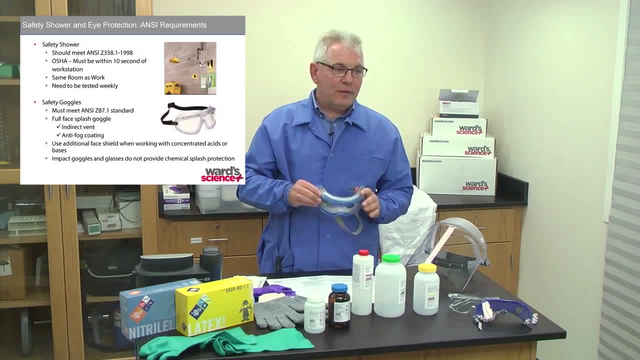 It should stay on until you push it back up. So goggles: So here again, I'm wearing glasses right now, but you know, you can get goggles to go over top of glasses, or they have to have that Z87.1 standard which you'll find on the side of goggles, And you can get indirect and anti-fog. 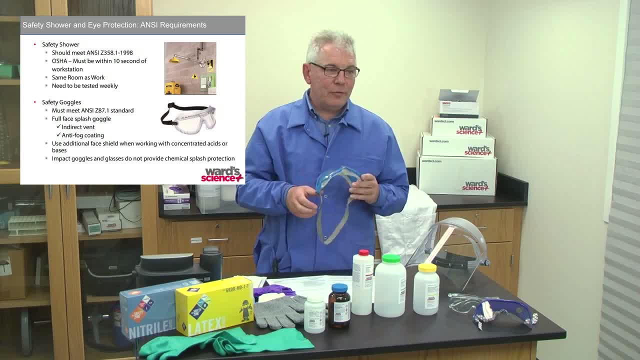 coatings today, So you want to make some that's comfortable, where the students you know the worst thing that can happen is you have a student that's wearing them and they're getting all fogged up and you know they still stick them. 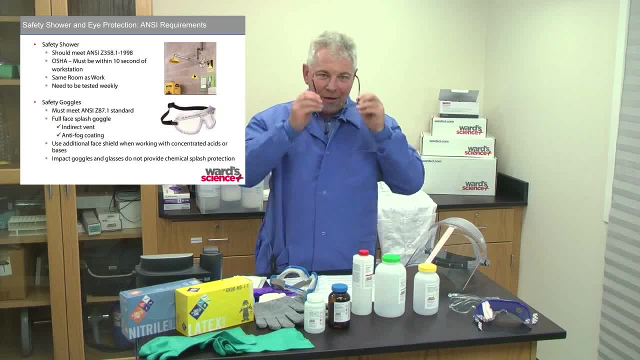 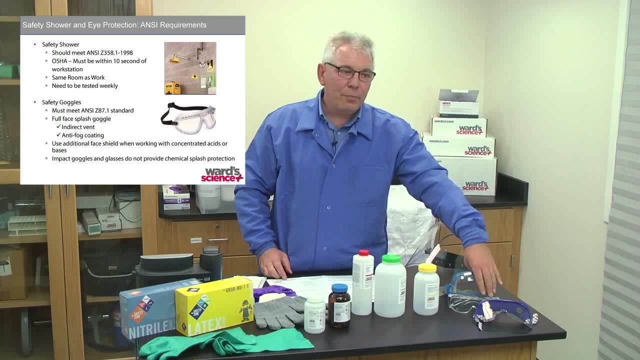 on the top of their head And you know they're really just because they can't see through them and it's not doing them any any help. There are impact goggles and glasses, but they don't provide chemical splash protection, So you can find those sometimes in a technology environment. 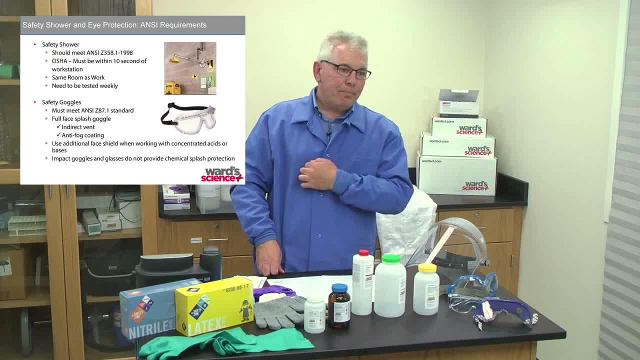 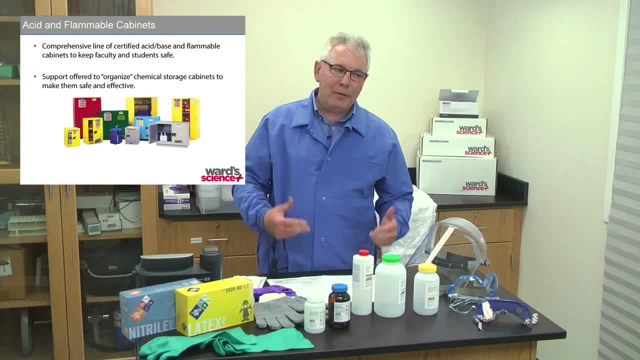 or industrial arts as we used to call it. Those would not work in a chemistry classroom. Next, please, Acid and flammable cabinets. So here again, we want to make sure that we have an acid cabinet and a flammable cabinet. We want to be able to organize those chemicals in storage. 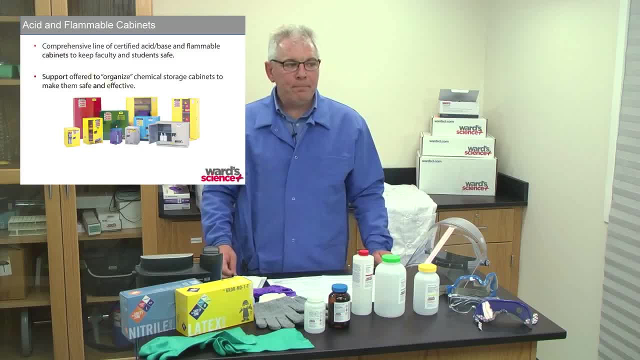 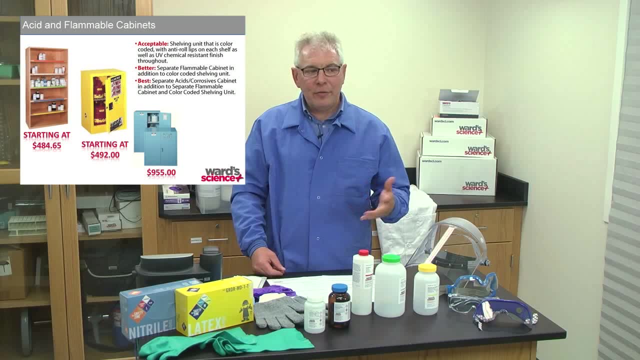 cabinets and make sure that they're safe and effective. Next, Here again these are: there's different aspects here that you can see acceptable, better and best. So there's different things that you can look at in the way that you're storing chemicals. You know open. open shelving is with. 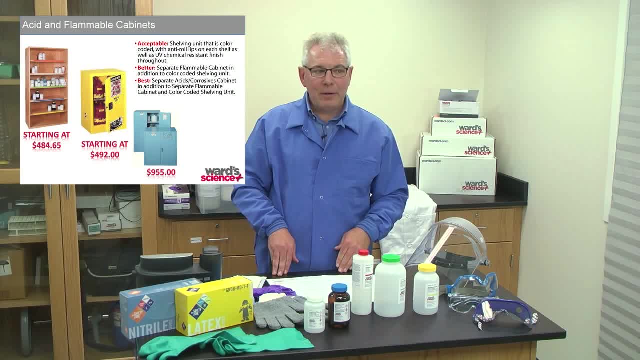 color coding is is perfect. Of course, a separate flammable cabinet is more ideal. If you don't have money for a separate flammable cabinet, we want to make sure that we're separating our oxidizers and our flammables by at least 20 feet, So we can't really keep those together Here again. 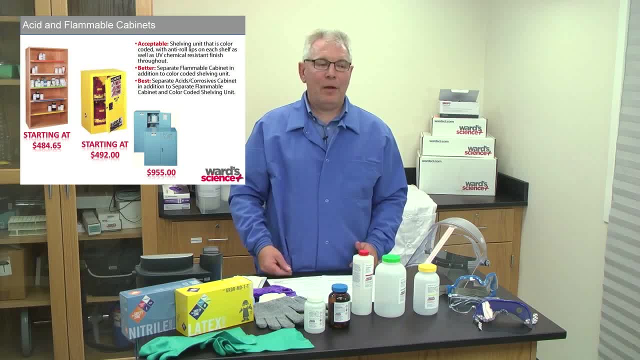 if you're putting your flammables in its separate cabinet. that's a more ideal setting And, of course, if you had separate acid and corrosive cabinets. sometimes those are really nice if they're underneath your lab Fume hood, so that you're minimizing the amount of walking that you're doing. Next, please, Chemical. 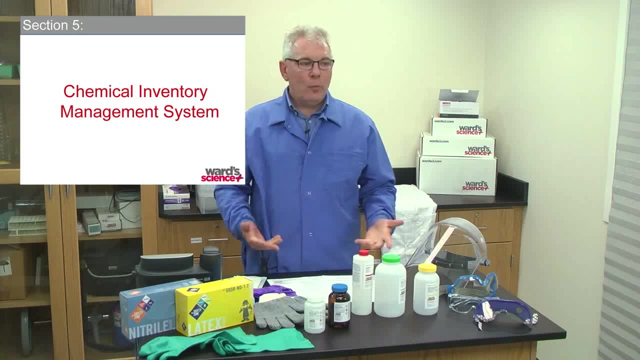 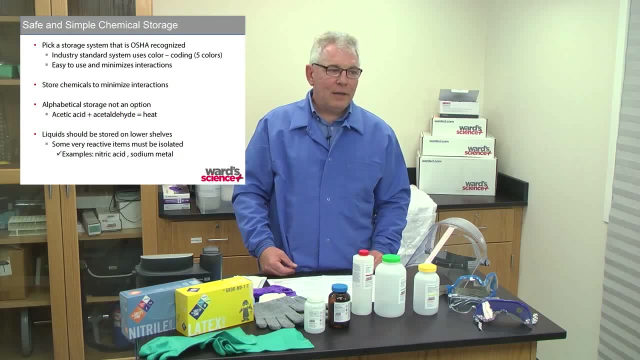 inventory management systems, or SIMS as it's called. So Wards has a chemical system. So here again let's talk about the storage system. We talked a little bit at the beginning. You know, we don't want to store our chemicals- A through Z, all mixed together, If you look, you know. 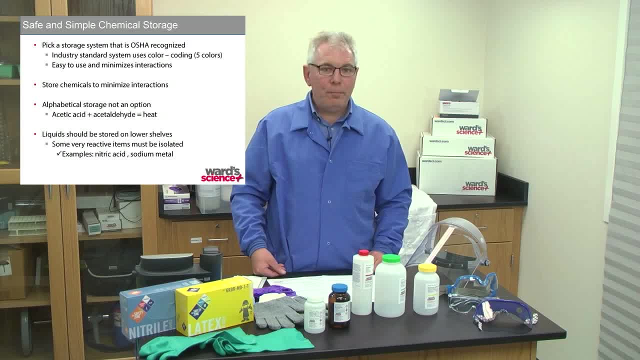 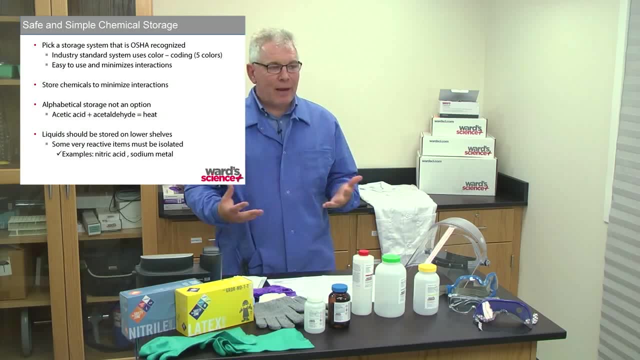 acetic acid to acetaldehyde. both are A but also mixed together if they leak would create a very good exothermic reaction. We want to store our chemicals so they minimize, you know, interactions. you know in the labs Liquids really should be stored on those lower shelves. We want to make 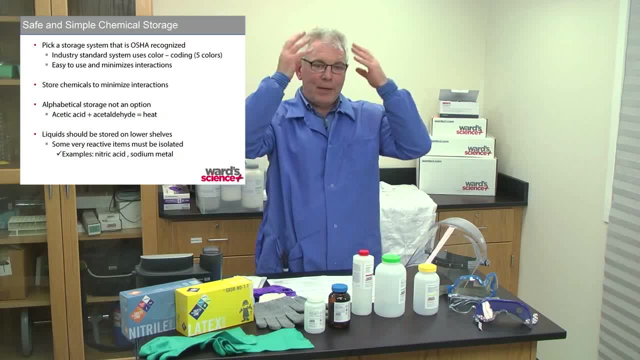 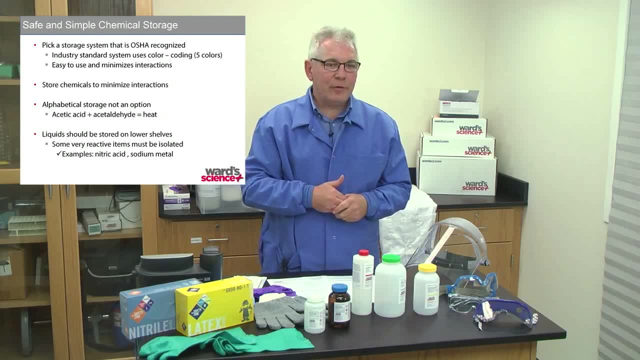 sure that you know something's not above your head so that you grab it, you know, and something the cap's not on, something comes on you. We also want to make sure that we're segregating certain items like nitric acid- it should have its own cabinet- And, of course, sodium metal as a dangerous 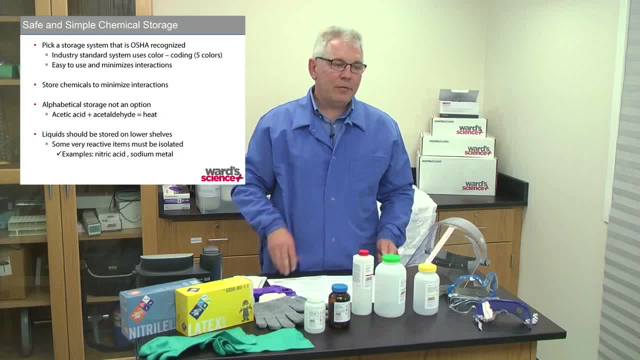 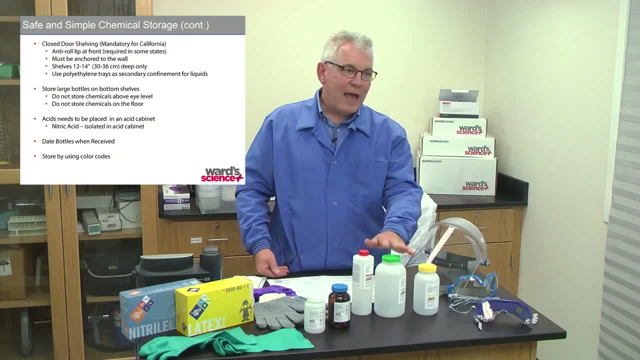 and wet is stored. They come in these nice little safety packs today, But those are very nice to segregate those separately When you're storing them. they come in mineral oil but you want to keep them in that mineral oil With a safe and simple storage system that Wards has. you know we have closed-door shelving Of. 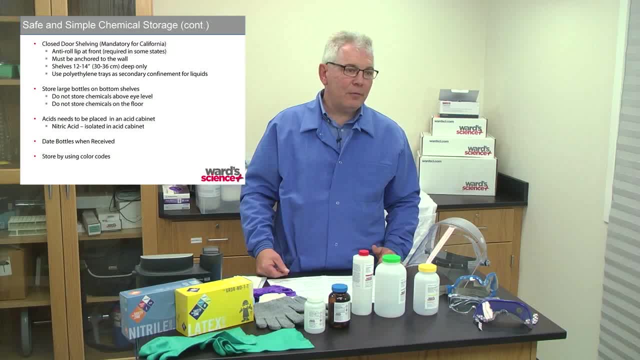 course it's mandatory for California. We're going to have some kind of an anti-roll lip in the front and we want to make sure that it's anchored to the wall. So what we're seeing can happen is a shelving unit comes down on you. If it's just a simple shelf, that's stored if we put too much. 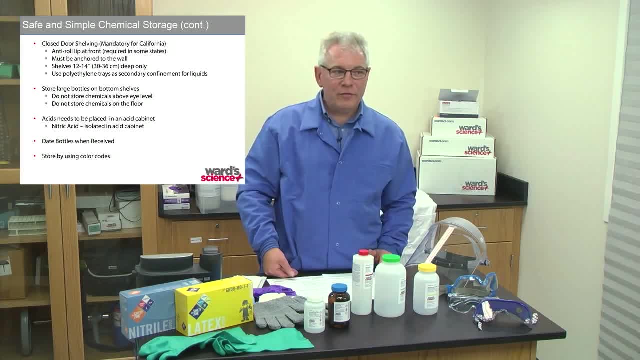 on it. shells really shouldn't be too deep. You know, 12 to 14 inches is ideal setting for that classroom or that lab And ideally if you can have polyethylene trays for secondary containment for liquids, it's really nice. The worst thing that can happen is you come in on a Monday morning. 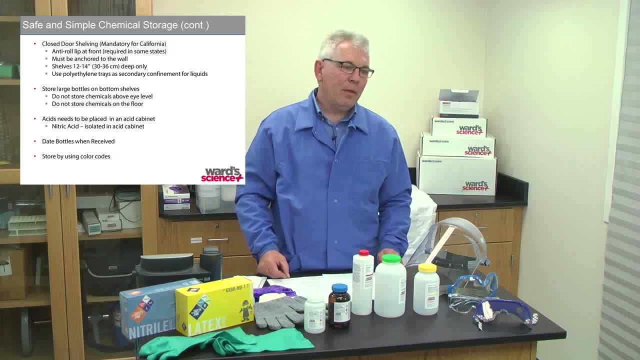 and you come to the spill that you have to clean up. Talk a little bit about large bottles. you know if they're down below versus above your head And really acids need to be stored in that segregated cabinet. One of the things you want to do is there's a spot. 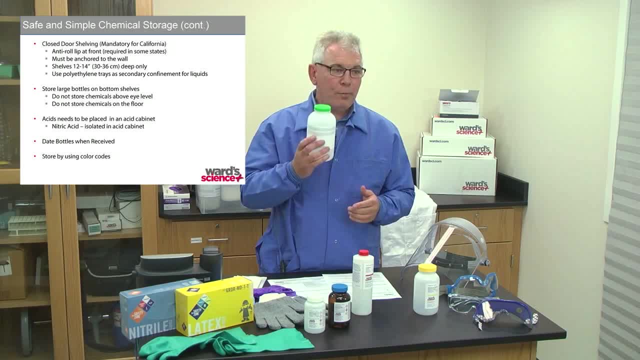 I want to make sure that you take a China marker or something out of a marker you know. mark down when you receive that chemical. Here again, it may be your classroom, but next year you may get promoted and moved to a different school or go on to do something else and somebody. 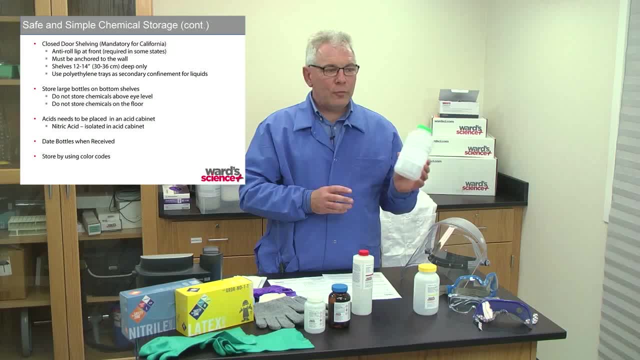 may adopt your classroom. So things that were in your head someone can see. you know I only got those last June or you know I got them in June 2004.. So you know I was in a school district in. 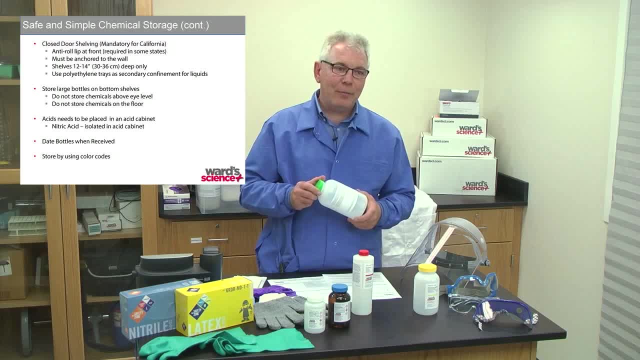 and I told the teacher: you know, if the chemical is older than you it's probably time to get rid of it. So there were things that were in our classroom that were from the seventies, And so it was. you know, that helps sometimes maintain your inventory, And a lot of times there may be. 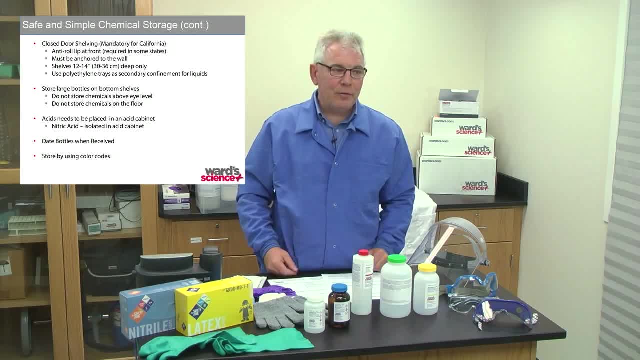 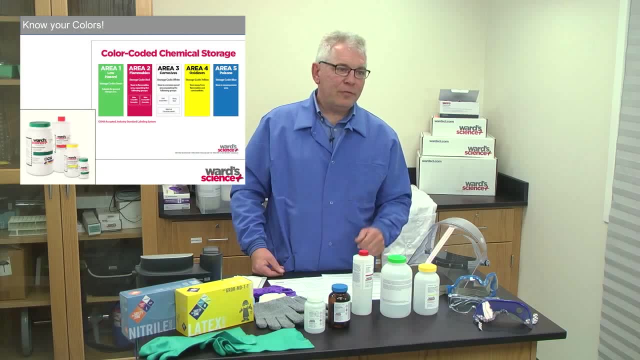 chemicals that aren't used in your curriculum anymore, you know, and you can evaluate those at the end of the year. But make sure you're storing your chemicals by your color codes. This is, you can see, a color coded area. So there's, you know, green, red, yellow. 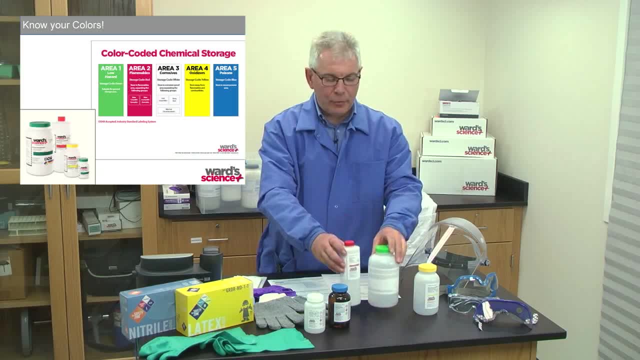 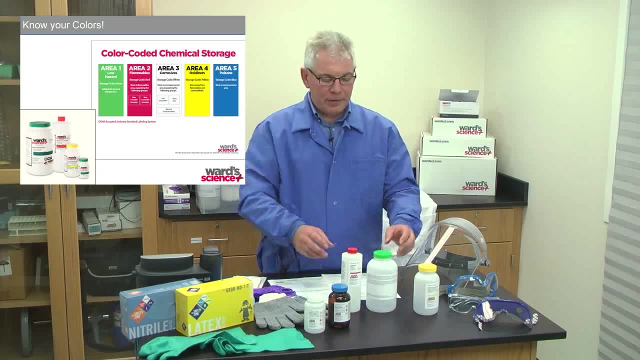 white and blue. It's here again with the color caps. It just makes it so simple to look around the classroom or the lab or your chemical storage area and see the different colors on the top, And if something is you know together like this, you know, of course, yellow and red. we want to. 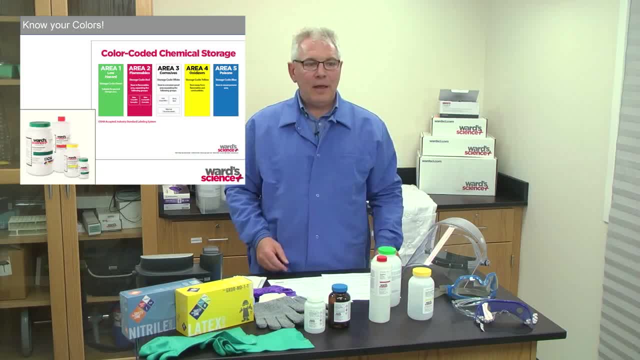 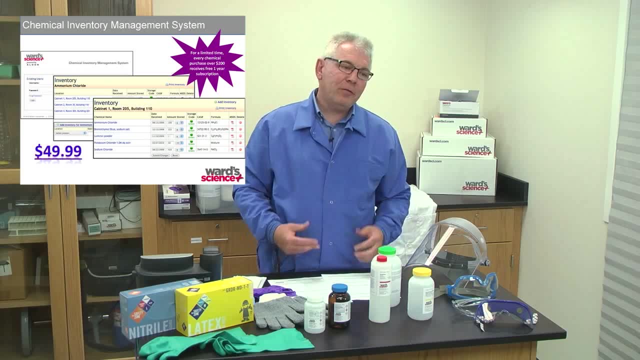 segregate that by 20 feet, but you can see that just by the color codes at the top of the bottom. Next, With a chemical inventory, management is completely cloud-based. It's going to be able to store. it has over 2,300 chemicals in the database, but you can also add your own chemicals. 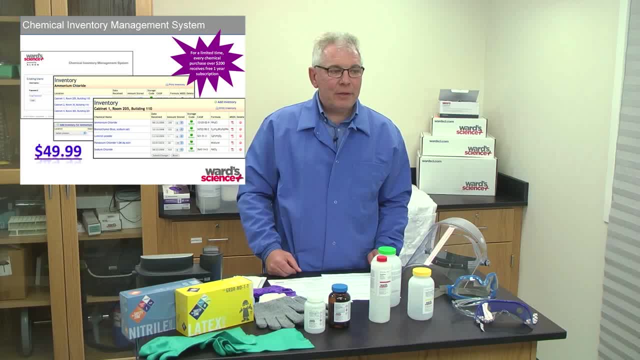 So $49.99 for a building. you can keep track of all the chemicals in that building and you can sort by. you know what are all the hydrochlorics in our building. You may have run out of something and another teacher down the hall might have it in one of their, in a biology classroom. 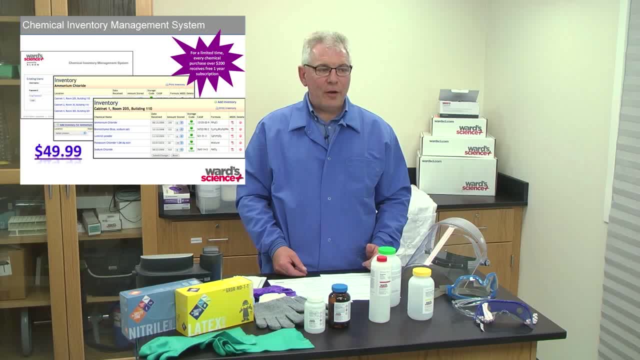 or maybe a physics setting that you didn't know And you can actually share, instead of trying to rush an order or get something flown in overnight. It's so expensive to try to ship chemicals via airplane, whereas you can actually manage your chemical inventory a. 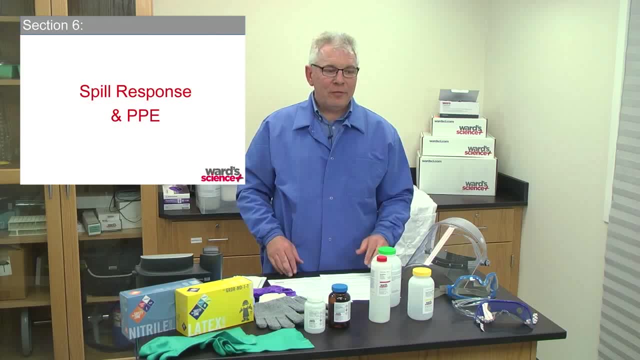 little easier: Spill response and PPE. So we talked a little bit about spill response. You know I had my my kit here. So we want to make sure that in the setting that we know what we're doing, we want to be kind of trained to do that. It's really good if you can get together as a 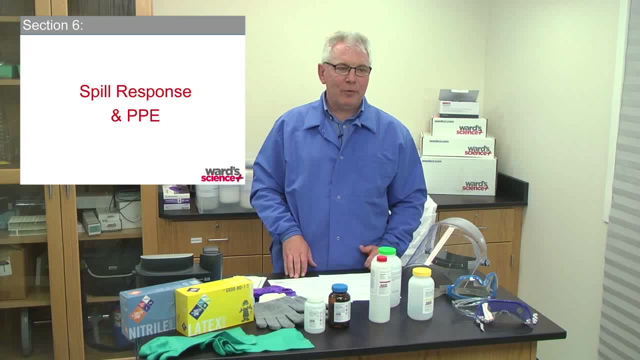 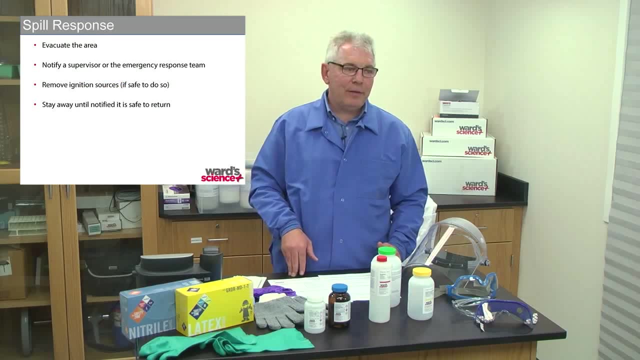 department kind of go over the setting What happens, What are the most hazards? You're going to have to go through all the chemicals we have in our lab or our classroom, But if something happens, you know boyish case, let's- you know, evacuate the area and let's notify a supervisor. 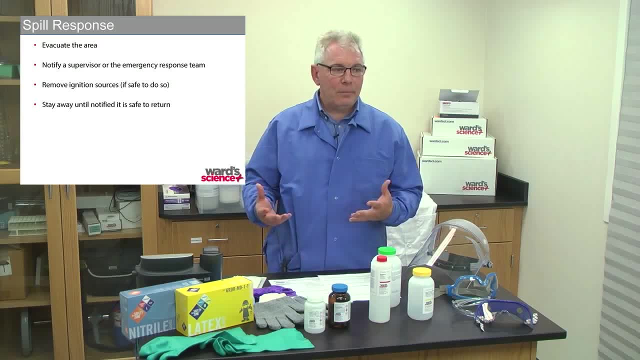 a chair In some case. you know the principal. we want to get the make sure that there's an emergency response team. that's needed. We do need to remove any ignition sources if it's there's flammable And stay away until you know it's notified for safe return. You know. 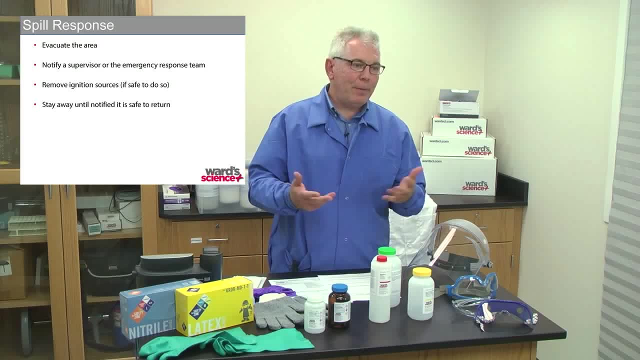 if it's a simple little- you know something like Biuret or Benedict's solution in a biology class- you know it's small enough that you can handle it yourself, then that's great. But if you don't feel comfortable doing it, we want to make sure that you get out of the area and that you have 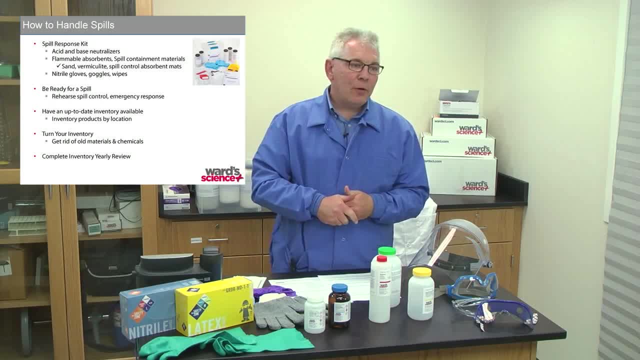 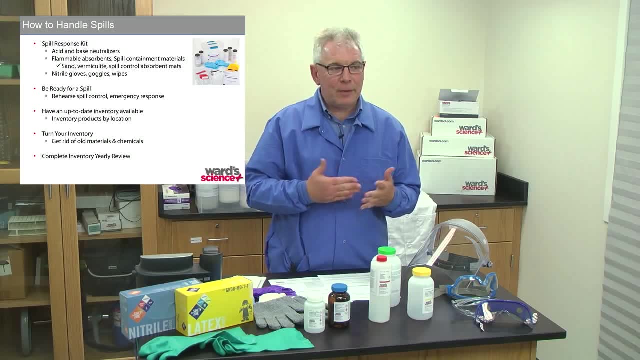 a training professional help you. There are a lot of spill response kits that are available. We want to make sure that we also have acid and base neutralizers, So if you do spill an acid or base, that we can neutralize those right away. And then, of course, flammable absorbents are. 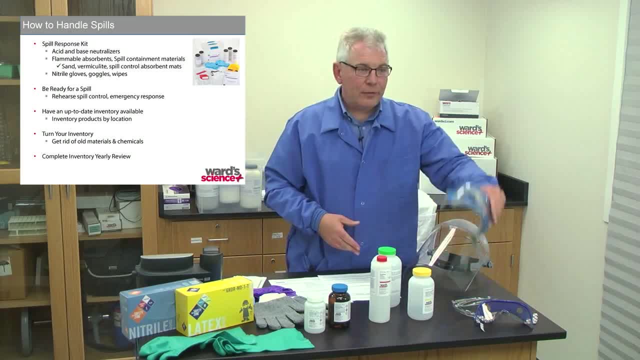 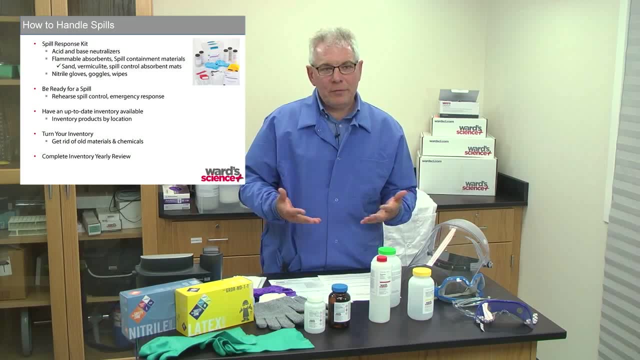 very simple. We want to make sure that we're wearing our, our nitro gloves, our goggles, and we have wipes available. We want to be actually, you know, be, ready for a spill. So I talked a little bit about, you know, take your, your, your department, have a meeting about. 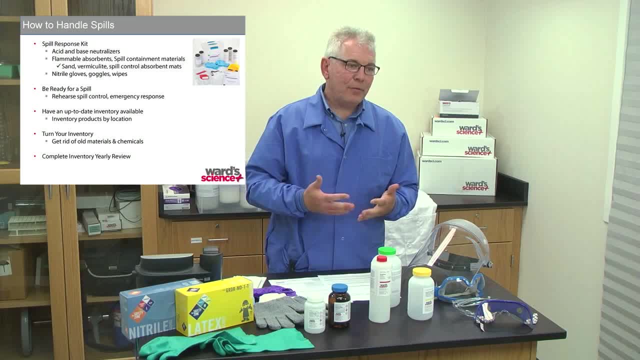 it go over rehearse a spill. What happens you know. so you can find a lot of problems. Maybe you decide that you know what if something happens. you know we're just going to hire somebody. There are companies out there that can take care of that for you. We want to make sure. 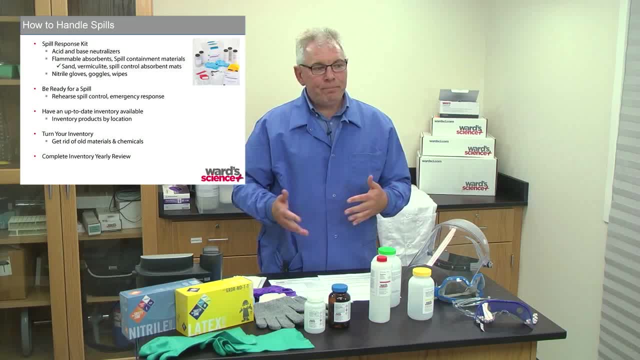 that we have an up-to-date inventory Here again at the end of the that class year. you can use that inventory to plan for a spill. We want to make sure that we have an up-to-date inventory Here again at the end of the that class year. you can use that inventory to plan. 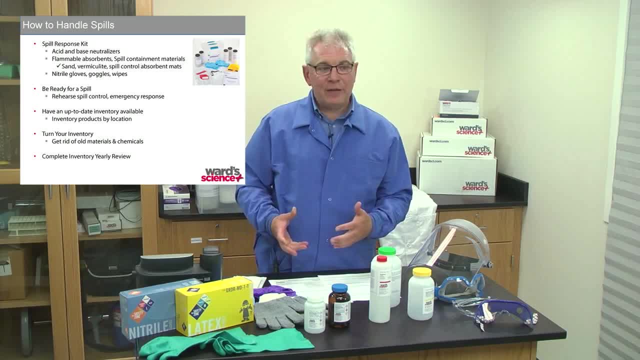 for next year. What are the next year's curriculum? How's it changing? We're changing our textbooks. We don't need this anymore. Hey, we're going to need this. Or there are ways to share chemicals within your school. You know, we want to make sure that we're getting old materials. 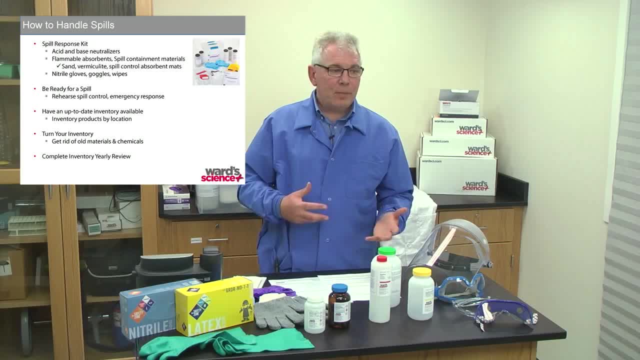 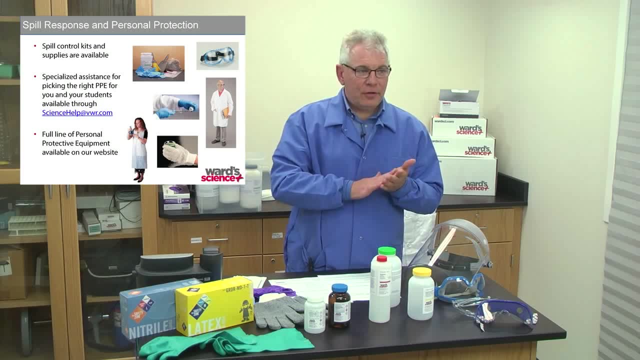 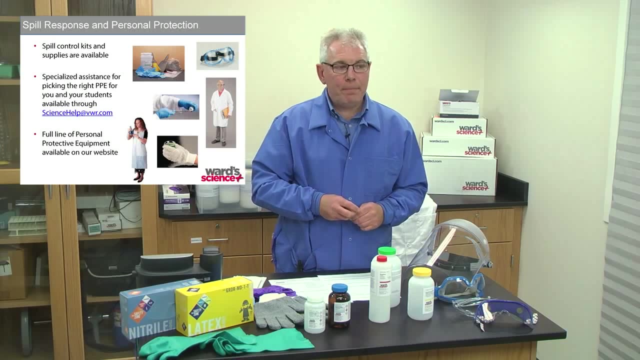 getting rid of old materials and chemicals that we're actually and completing that inventory yearly Next. So spill response and personal protection. you know, with those spill kits there is assistance. If you do need help, you can always email sciencehelp at bwrcom. 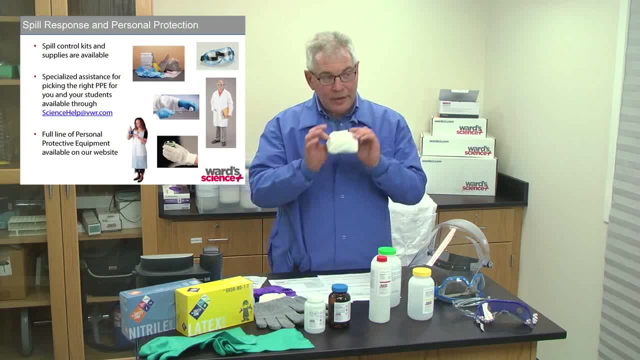 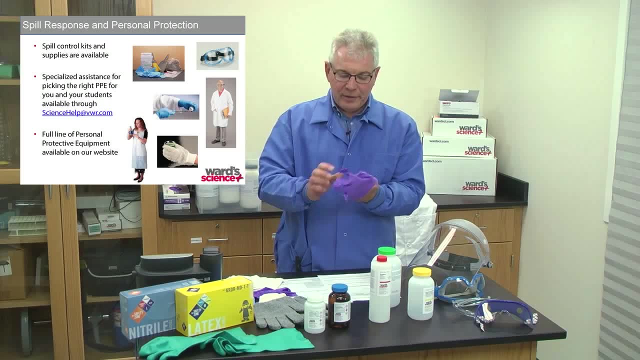 And that's it, Thank you. And there is like a full line of products. So you know, there are simple things, like you know, disposable aprons: We want to make sure nitro gloves are perfect, And one of the things I like to talk about sometimes are nitro gloves, Of course. 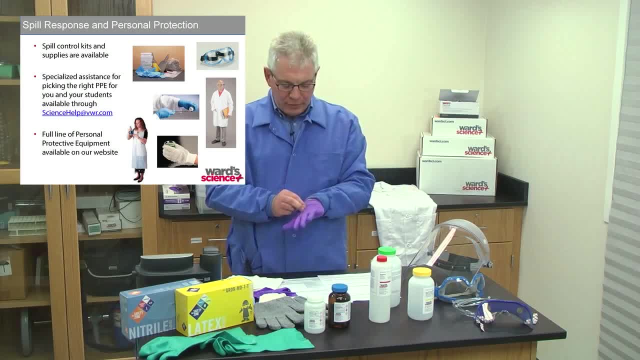 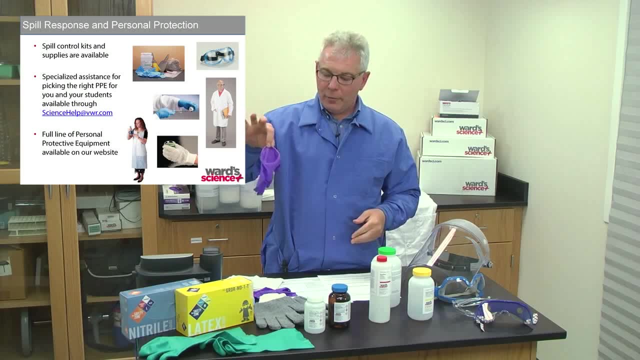 I have big hands and I'm putting out small gloves, but you know, when you're dealing with a glove want to make sure that we grab that bottom of the glove. you know we're turning it inside out And so actually, if something's on your glove, it's on the inside. Next, 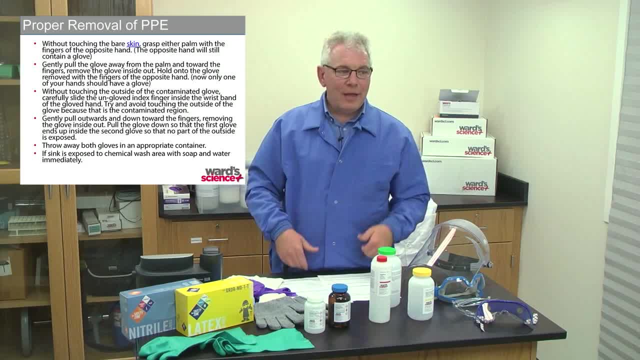 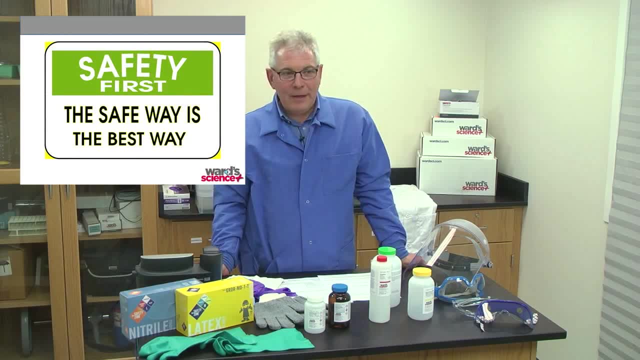 So this is kind of like that per the proper removal. It's kind of like I just did it simplistically, but it's kind of written out for you. Next, Safety: first you know, here again, in that classroom, that lab, wherever you end up in life. 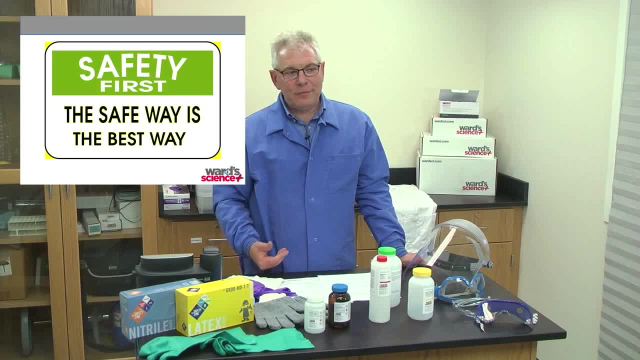 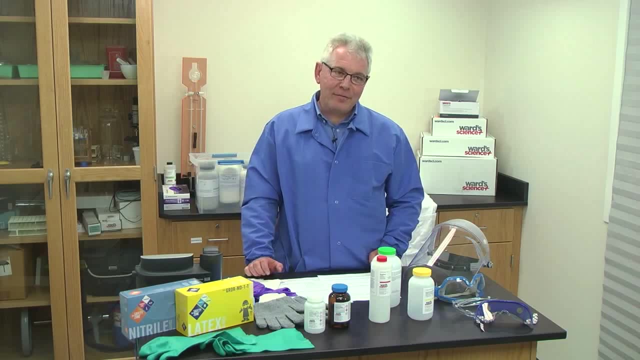 you want to make sure that truly it's the safe ways, the best way. We don't want to cheat the system. We want to make sure that, from a due diligence perspective and a liability perspective, we're doing it the safest way. I want to thank you so much for joining. I know I talk really fast, so it's. 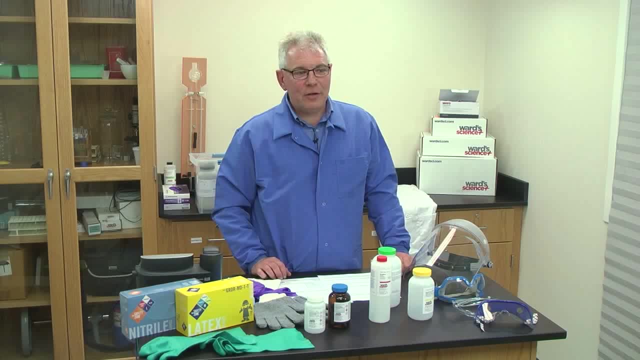 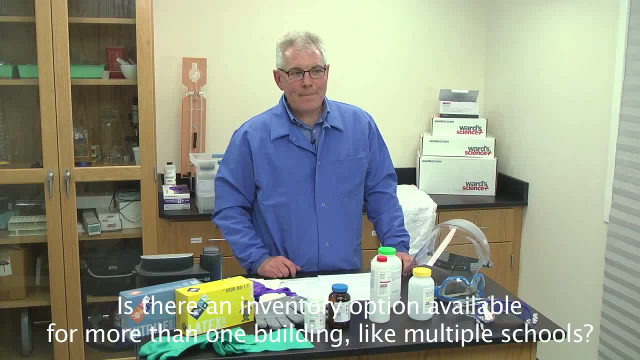 about 45 minutes into the presentation. Do you have any? if you have any questions, you can go them online or star six on mute. Yeah, So there is a question that actually came in now. Is there an inventory option available for more than one building, Like, let's say, multiple schools? 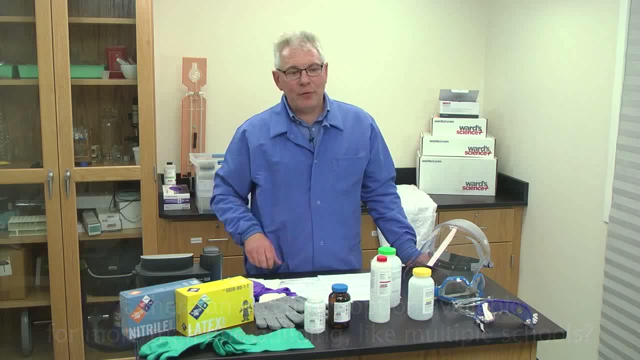 Yeah, So there's another. besides the $49 version, there is a $199 version that goes up to 20 schools. Yeah, So there's another. besides the $49 version, there is a $199 version that goes up to 20 schools.